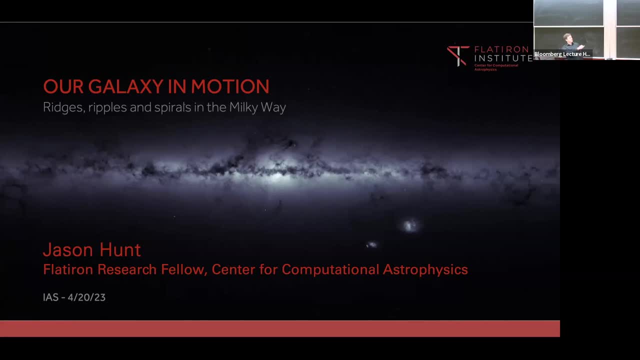 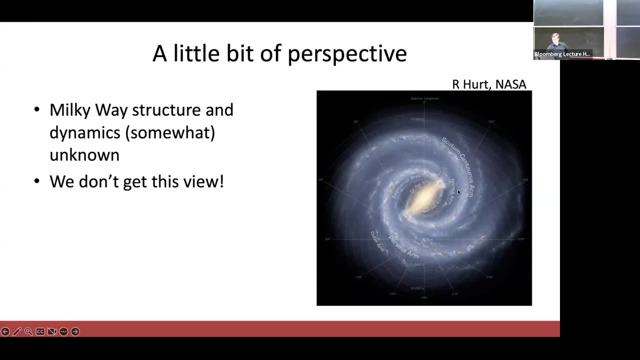 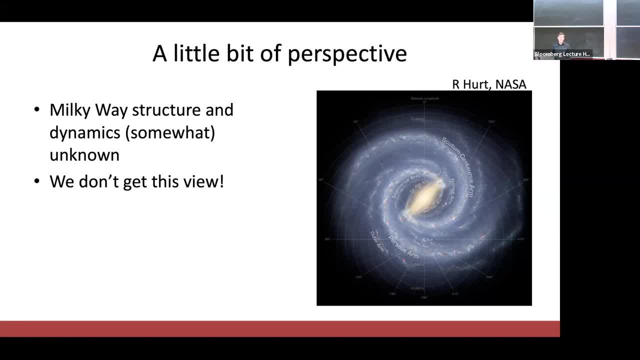 which is based on some real data, but we don't have this global view of the galaxy. We can't look down on the Milky Way's disk such as we can stare up into the sky at the countless other external galaxies. We know we're a barred spiral, but the exact parameters of the bar and the spiral? 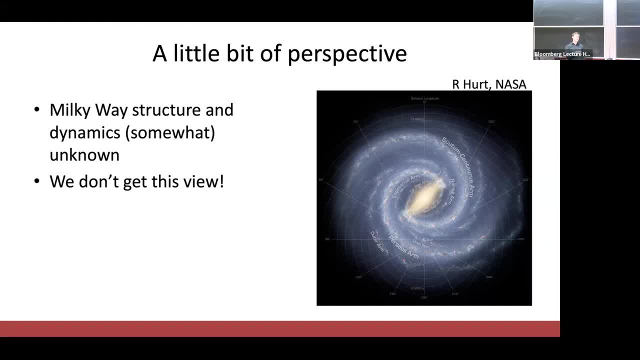 structure, have a lot of uncertainty in them and we already know ways that this picture here on the right, done many years ago at this point, is wrong, even though it still becomes a good illustration for us to talk about the Milky Way. The reason it's hard to get a global picture is: 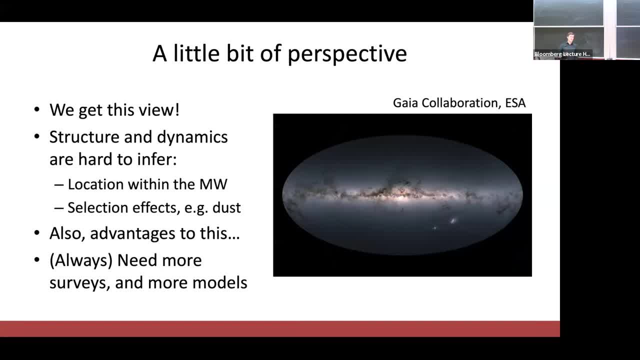 because we actually get this view We are living with inside the disk of the Milky Way. We look out kind of can't see the forest for the trees, type of thing. You see this image on the sky but it's complicated by complex selection effects that are inherent in any survey and complex. 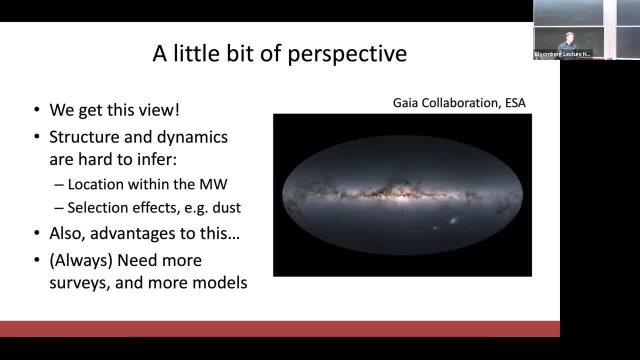 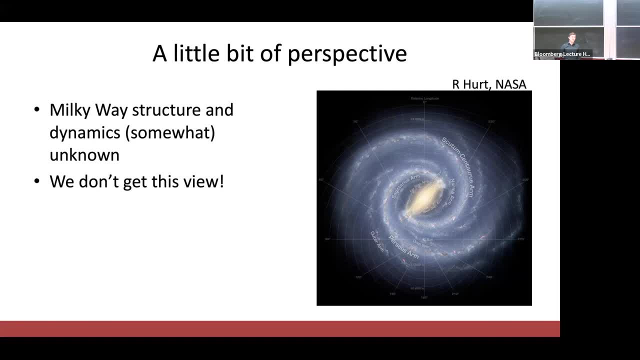 effects, such as dust extinction, which stop you from viewing stars all throughout the galaxy, And so, for some degree, our job is to turn this view that we have here into this view for a global understanding of the Milky Way and what's actually going on in that galaxy, And to do this 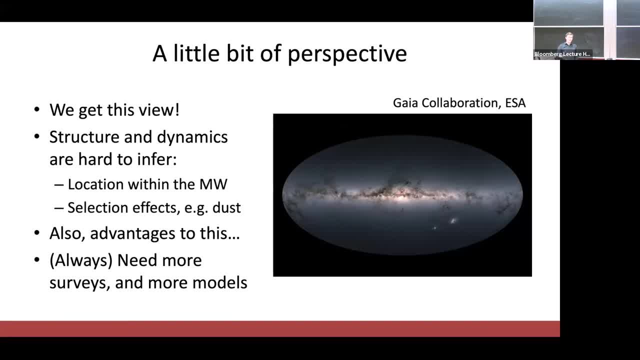 we always need more surveys to give us more data, to map more stars and tell us what's going on. We also need good models to help us take advantage of that data and help compensate for the observational biases and selection effects. However, there are also advantages to this view. 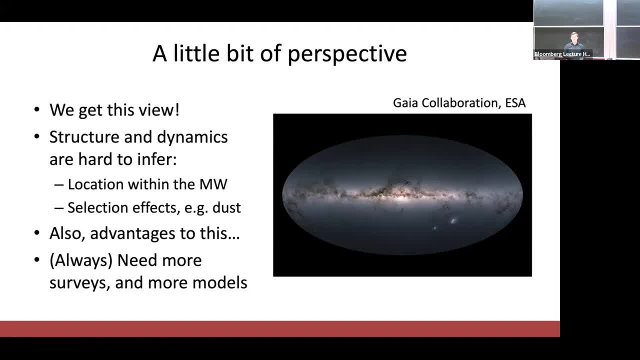 of our position within the Milky Way. It's the only galaxy where we really have a 3D laboratory with positions and motions for billions of stars. We can kind of see galactic dynamics happening up close, not over time scales because we have this single snapshot frozen in time, but in like a fine. 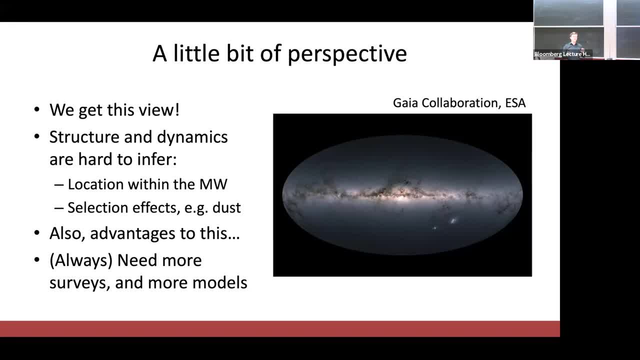 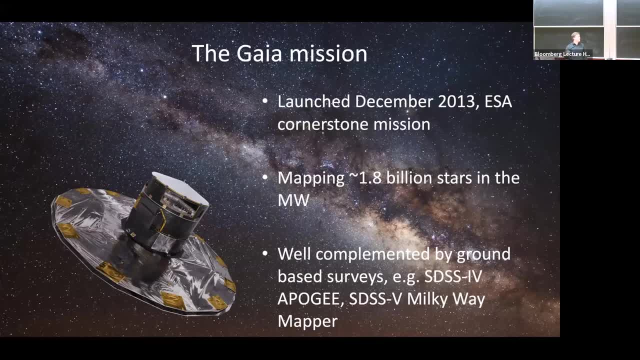 resolution. whereas we look out into the real universe, we only see galaxies, kind of as a whole. So, to give us more data, this is the European Space Agency's Gaia mission, the time I said I worked for briefly launched back in December 2013.. This is Cornerstone mission and the tagline is to 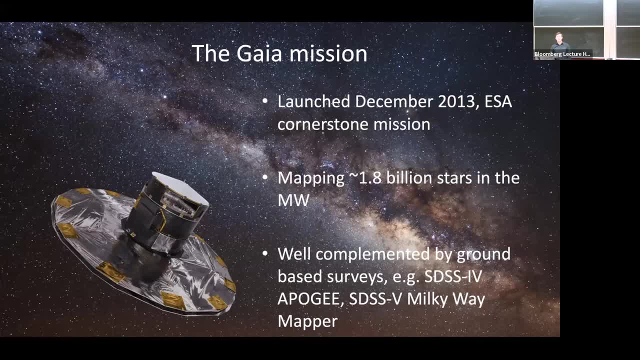 map one billion stars in the galaxy. It was supposed to cost one billion dollars, so every dollar you spent was to give you one star's worth of information. However, in the end it's mapped about 1.8 billion stars at this point. It's doing way better than expected and somehow stayed off budget. 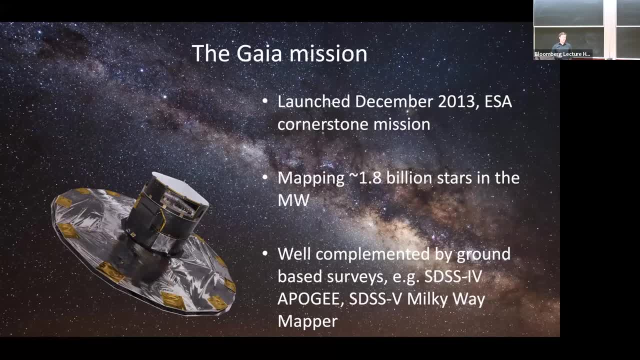 It's primarily an astrometric mission, so it gives us positions on the sky, parallaxes, proper motions, So it's very well complemented by other ground-based surveys that give us vector stopping information, such as more radio velocities or elemental abundances, such as from the 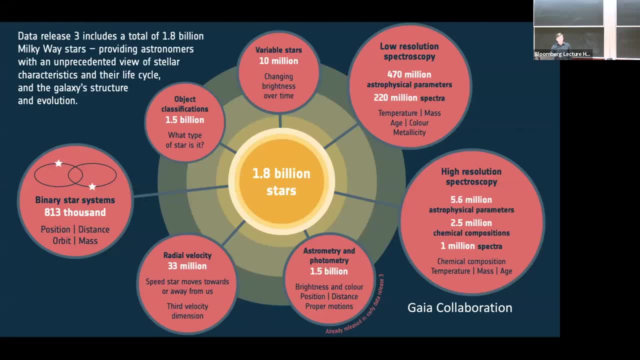 ISS missions, but many others. And yeah, just as a short summary of what Gaia has given us up until this point: 1.8 billion stars positions on the sky, then 1.5 billion, 1.5 billion for the astrometry and photometry. so this is parallaxes, proper motions, brightness and 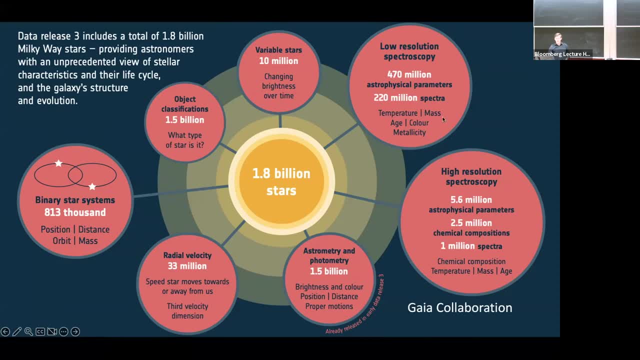 color. then you drop down to a couple of hundred million low resolution spectra and astrophysical parameters- temperature, mass, age and time. And then you drop down to a couple of hundred million low resolution spectra and astrophysical parameters- temperature, mass, age and time. 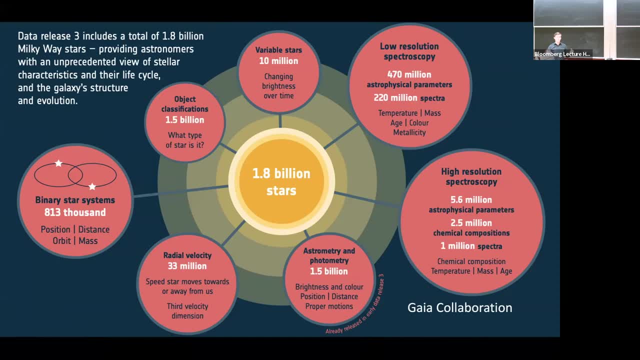 And then you drop down to a couple of hundred million low resolution spectra and astrophysical parameters- temperature, mass, age and time, But they're not particularly precisely measured, but we do have a broad sample- And then down to about 33 million radio velocities which complete the six-dimensional. 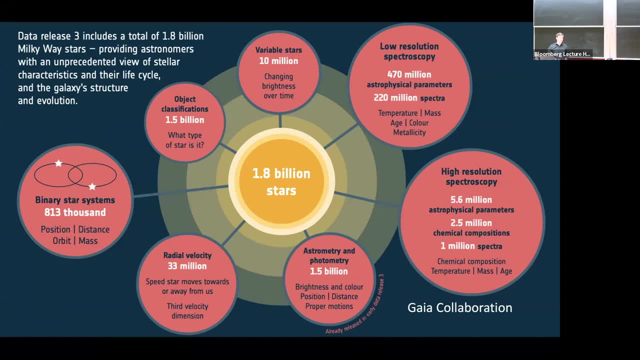 phase-based information of position and velocity. So that's the sample I'm mostly going to talk about today. If you're not interested at all in galactic stuff, Gaia also measures a lot of binary star systems. It measures a lot of asteroids in the solar system and it can find, I believe, 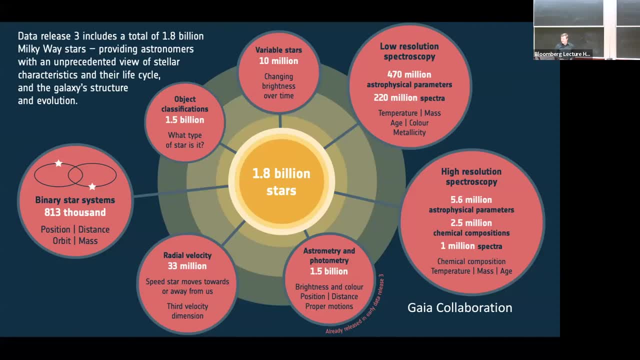 Jupiter-mass planets to meet SpaceX, I think was where they get to. But yeah, this is the current state of the data set. We had data on this three last year And for me as a galactic dynamicist, Milky Way survey scientist, the most exciting thing has been. 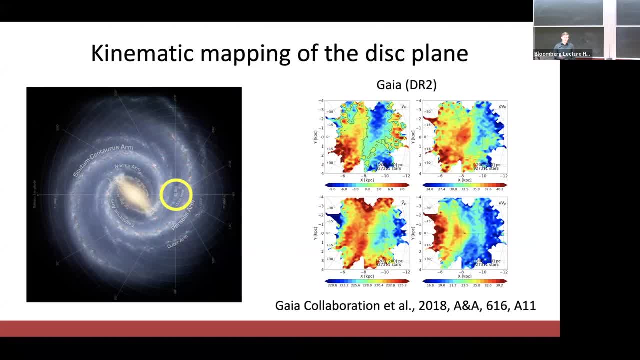 we've started to be able to make large-scale maps across the Milky Way's disk, not so much in terms of structure, because extinction effects really make it hard to calculate stellar densities over large distances, But if you're looking down on the plane here, this is putting. 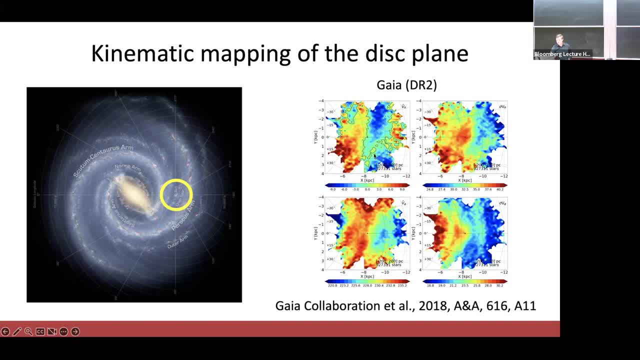 a little ring roughly corresponding to the area of these plots. you can see there's a map of mean radial velocity motion of stars towards and away from the galactic center. This is mean rotation velocity stars moving around the galaxy and these are their dispersions. 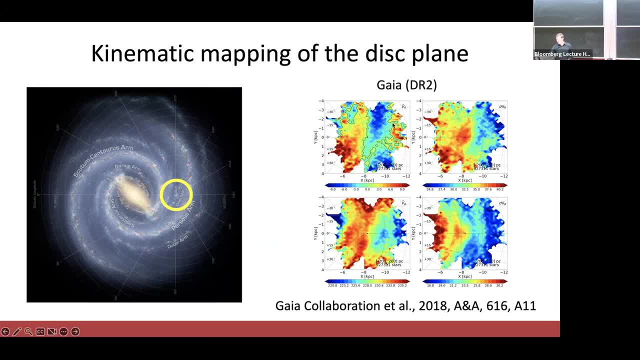 And you can start to see a large-scale structure here. Radial velocity is stars moving inwards, blue is stars moving outwards, And I'm not going to go into too much detail. but basically what you see here is everything is not smooth and stable. If we lived in a perfectly axisymmetric 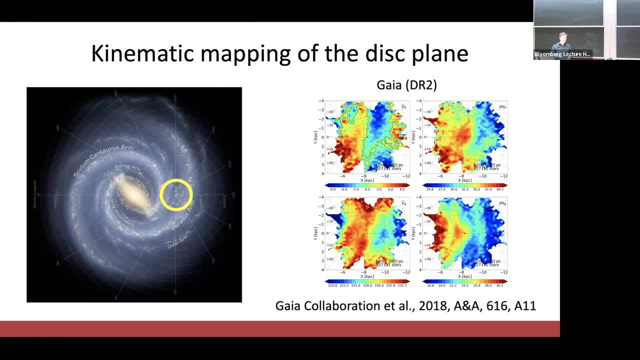 disk. in equilibrium, these would be effectively zero, But no, there's lots going on here. This is not a surprise to us. As we've always known we've lived in a well, not always we know we live in a bird's-eye view of our galaxy. This should be here, But Gaia has really helped us start to push these maps. 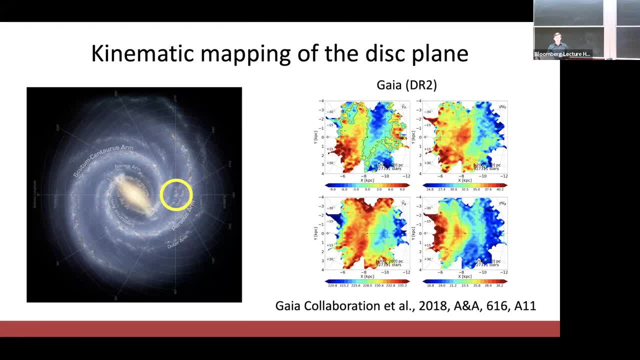 outwards and see what's going on. This is interesting not just for like galactic cartography, but these velocity filters can inform us on what's actually happening in the galaxy and the galactic dynamics that underlie them. And I said, Gaia is well complemented by spectroscopic surveys by 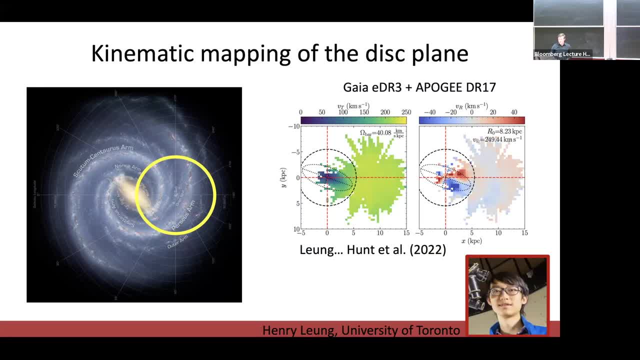 combining Gaia with Apogee and a neural network work from Henry Leung and others, and show that you can make these kinematic maps over much larger distances. And you see now the kinematic imprint of the galactic bar pop up in the middle of this plot. So this is as I move, the velocity. 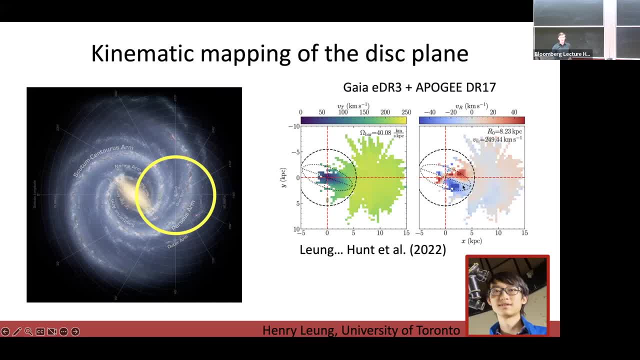 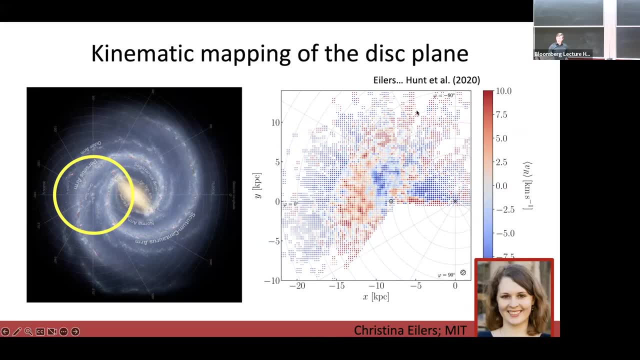 this is radar velocity. you see the quadrupole, which is the next feature of a galactic bar. And similarly, Christina Eilers, myself, using a different technique, mapped this large feature of radar velocity out here, which looks roughly like a spiral pattern which could correspond to one of the 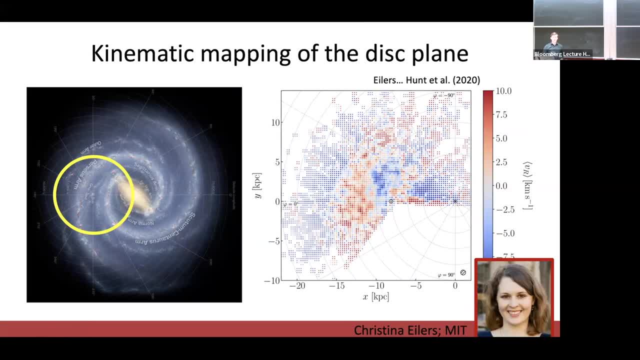 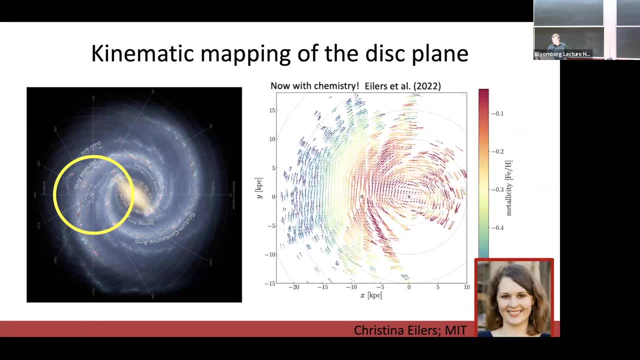 Milky Way's outer spiral arms. Still a lot of debate on that, But we are starting to get to the stage where we can map large scale kinematic features across galactic disks. There's one final one of these which I really like. This is that same selection from Christina Eilers, now updated to: 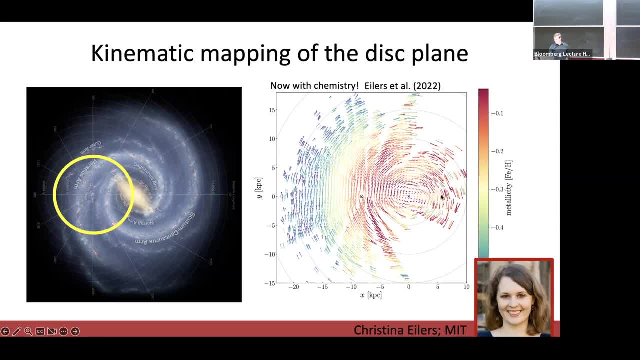 color code by Metalisti. There's iron over iron abundance And you see the Metalisti gradient very clearly as you go up to the disk And each of these little arrows are showing the motion of those stars. You can see clearly the galactic rotation, but also in the middle you can see 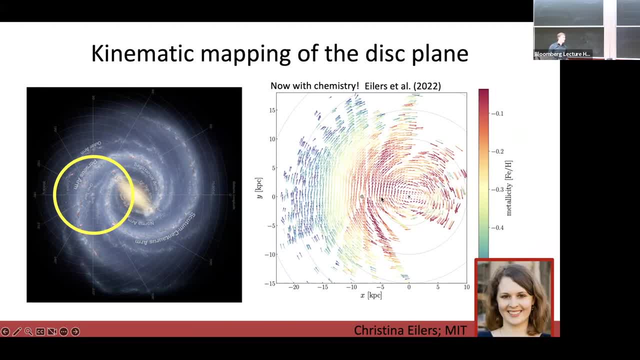 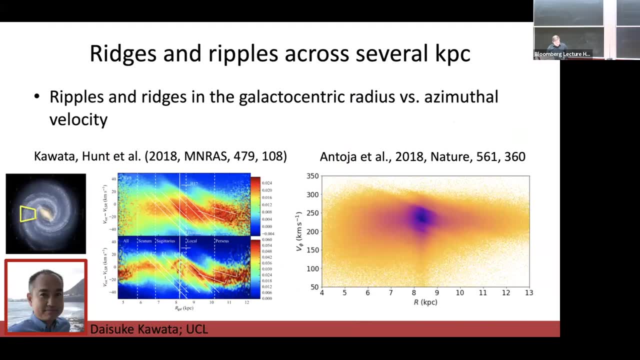 the flattening of these arrows into the galactic bar. So, yeah, we're just getting to the stage where this is doable and exciting and lots of things for us to learn. The other thing that Guy highlighted in DR2 was ridges and ripples in. 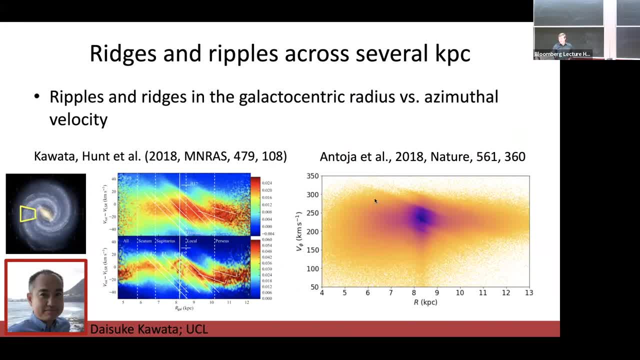 galactic centric radius versus other moveable velocity. So now you're looking at r. this is distance to the galactic center along the bottom of these axes versus v phi. so the rotation around the galaxy And we see ridges or ripples are prevalent in the space. This is two papers that 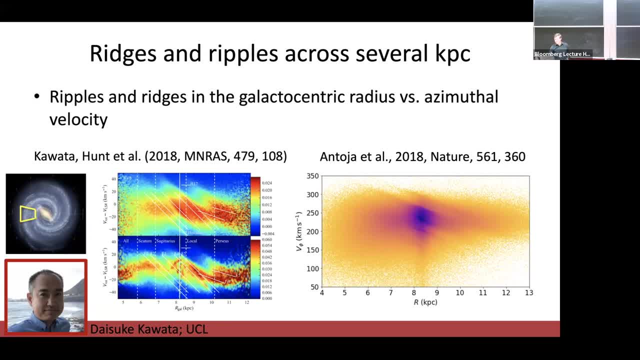 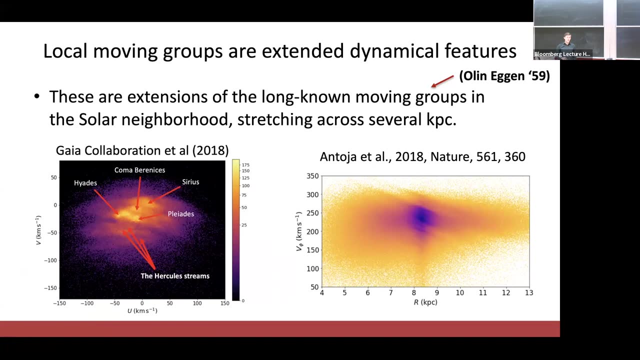 were submitted The same day, a couple of days after DR2, they're showing them both, but they find basically the same structure: these ridges in the galactic disk We have. we know ways you can form these. this is the first showing over large distances, but they're actually extensions of a long-known 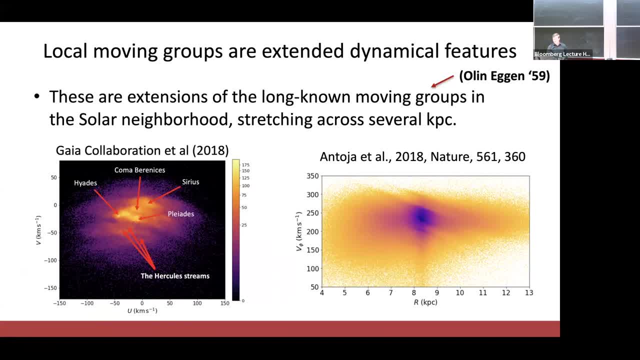 moving group that's consolidated it a fact by Olin Hagen back in the late 50s. So you have here Sirius, Heron-Herenices, Hyades-Plaides and the hyponese streams and the local velocity structure. 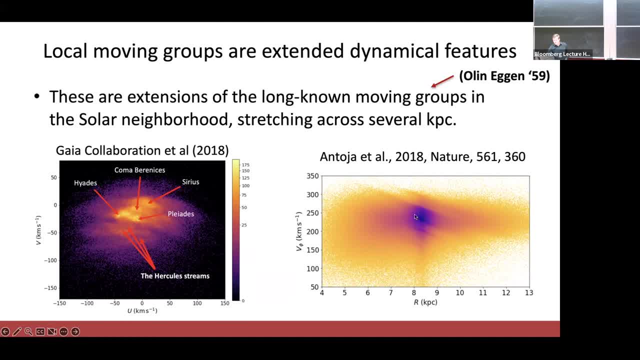 of the disk Radar velocity versus this neutral velocity, and these correspond to Sirius. is this big ridge here which stretches across several kilopassecs. Hyades-Plaides kind of blur together over this ridge here. These two are Hercules and you can see the hint of this thing that's actually called. 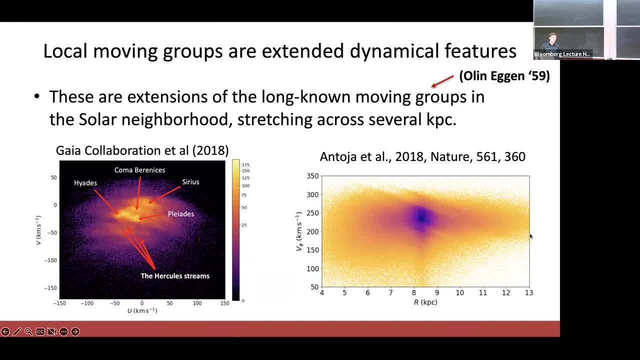 the hat is this big ridge up here. So originally Hagen thought they might be dissolving clusters and people discussed this for a while. There were many other reasons that's not the case, but you can now see just very clearly that these are large-scale dynamical features. 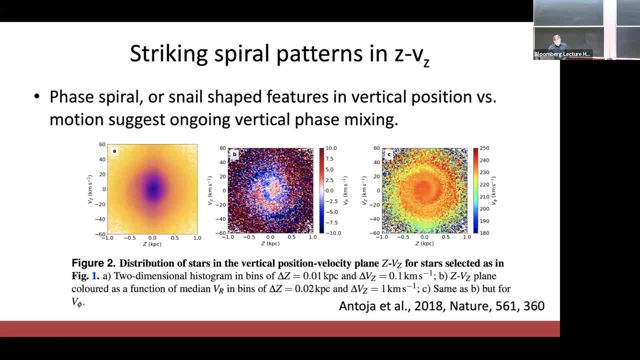 which stretch across the disk. The other thing that was found by Teresa and Toya in that same paper was striking spiral pattern in Z-V-Z- or Z-V-Z depending on where you're from- and this is a, so Z is position above and below. 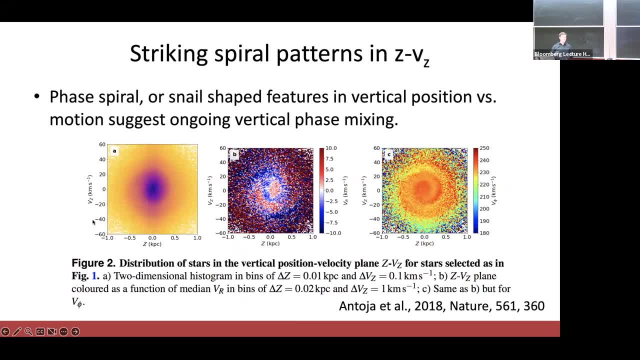 the disk plane V-Z is motion up and down. So this is taking a local volume and plotting vertical position versus vertical motion and you see a spiral pattern pop out just about in the number density of stars. It's kind of faint Radar velocity. you have a hint of it as well, still not very clear, but in as a 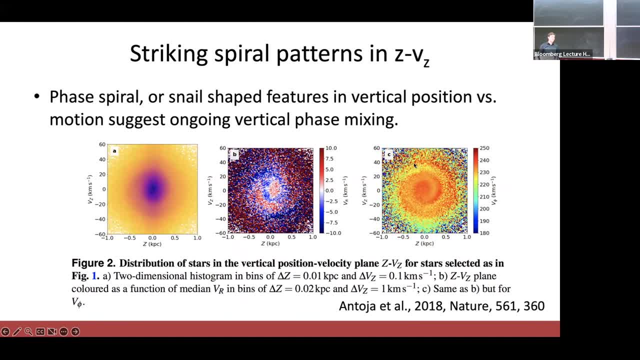 a Moetschler velocity it really pops out and you get the striking spiral or snail-shaped pattern in the position and motion of stars up and below the disc plane And this is some indication that there has been some vertical perturbation to our galactic disc and it's phase mixing back towards. 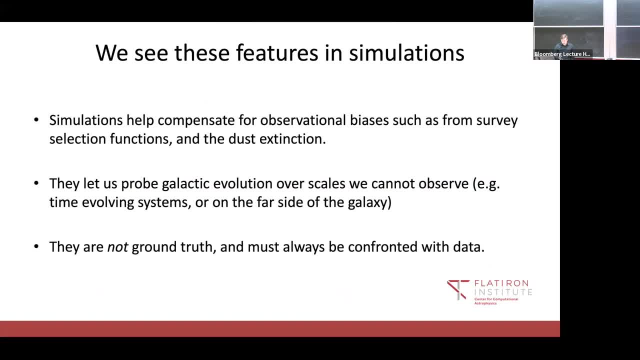 equilibrium. We see all these features in simulations. we see large-scale spiral arms patterns, but also the ridges in the radial position versus as a mo cual velocity, and we see that the snail spirals in the vertical position of motion, in the vertical position of motion, and it's important to look at these in simulations. 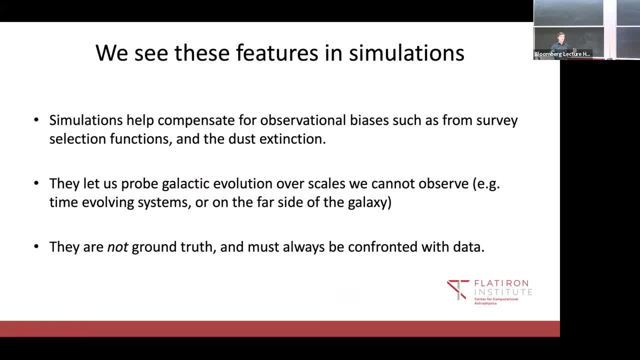 because they help us do two things. firstly, they let us look across the global that state of the disk to get around the selection effects from dust extinction survey science tricks. actually, you can see how they propagate across the galaxy. they also let us explore how they form and evolve. 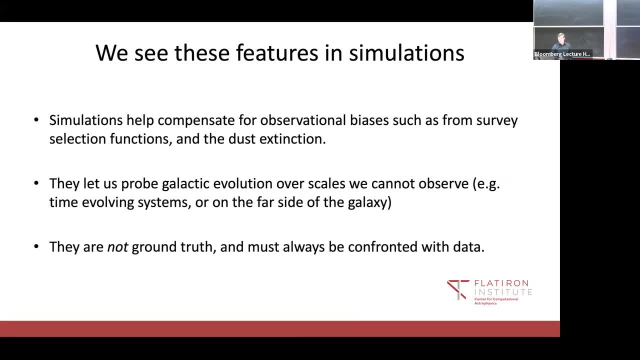 with time. so you're getting into another dimension you just can't do in an lqa. however, simulations are, of course, not ground truth, and you must always come back to see if what you're doing that does appear to be sensible. and just in brief: uh, these ridges can be made by bars. we 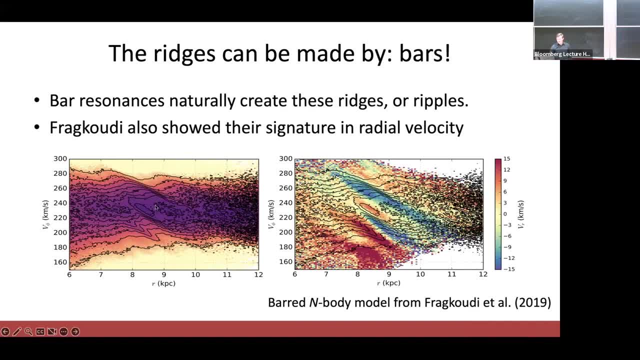 know, bar resonances leave, uh, the imprint of the space. the different um. this is, yeah sorry, rv phi in density from a bar and body model from francesca franguti, and the ridges also pop out in radio velocity, so you can make them with bar resonances. i'm not going to talk. 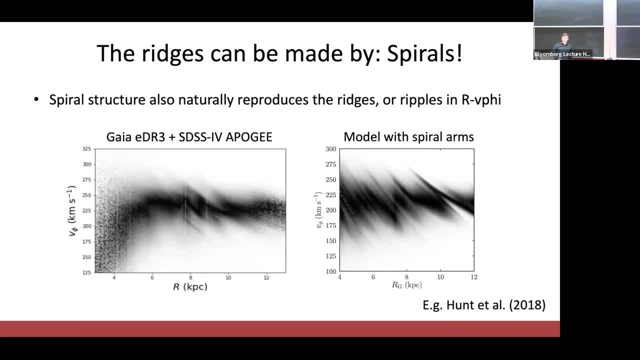 about that too much today. um, you can also make them with spiral arms. whether you prefer density rate spirals or transient winding material arms, they both leave ridges in the same space, basically any departure from equilibrium in this distance. there's another image of the guy data from me, combined with apogee and one of my models with spiral arms. you see the same rich. 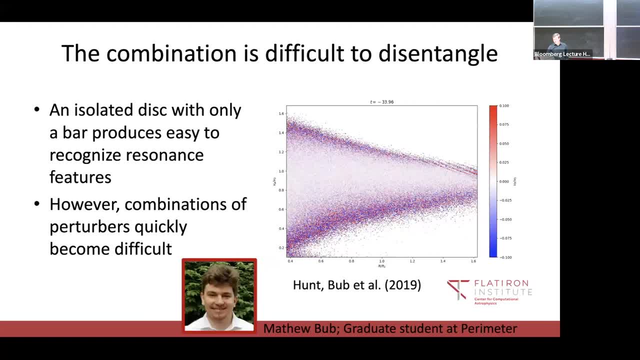 features appear and if you have just a bar and a smooth test- so this is a test particle model run by matthew bub, who was an undergrad when he worked with me, now grad student perimeter um, an isolated disc when we grow the bar here. so you start from this smooth distribution. this is 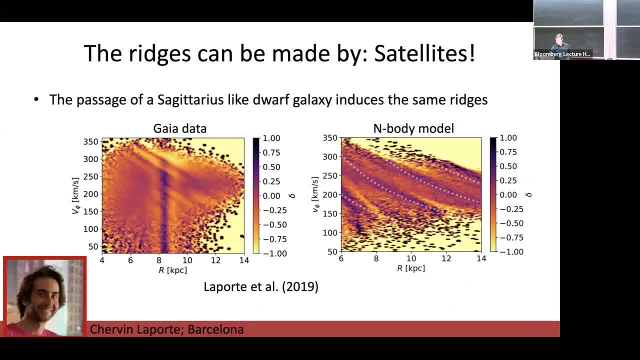 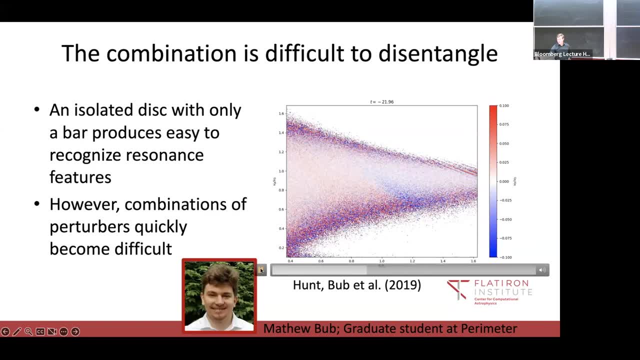 what the galaxy would look like if absolutely nothing was going on. oops, and then you grow a bar smoothly and slowly. you'll start to see this red blue pattern appear in the middle. so this is known as the outer, but it's caused by the outer limb line resonance of the galactic bar and if you know things such as your galactic. 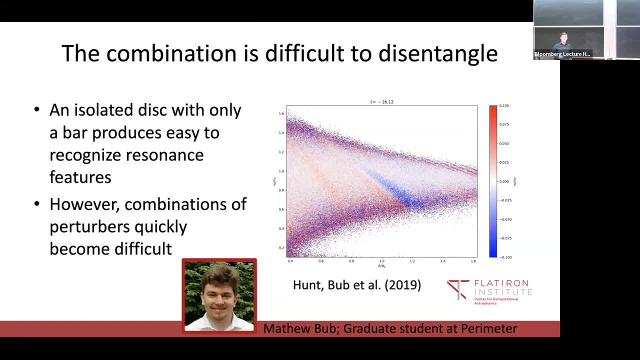 potential, the rotation curve. you can use these features to measure the pattern speed of the bar, because that affects when this falls in this place and the amplitude of the box affects how strong this feature is. if you have just a bar and nothing else going on, you can do this. however, if we then turn on some spiral structure, 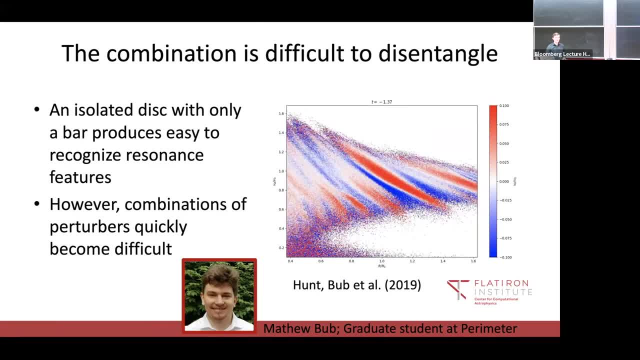 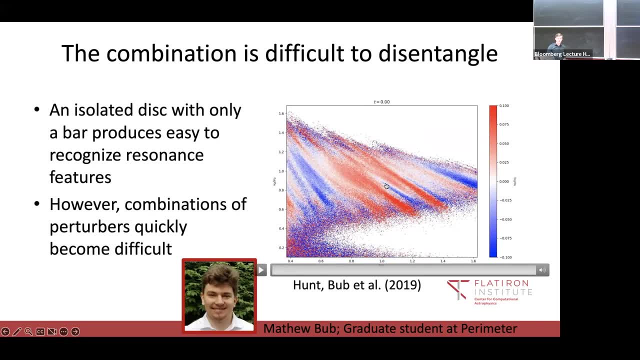 you see, this space actually then becomes quite messy. there's a lot going on. it's a lot of these red, blue features, a lot of these ridges in this plane. so we know, because this is a model, we have complete information. this ridge gap here is the one that corresponds to the bar resonance. 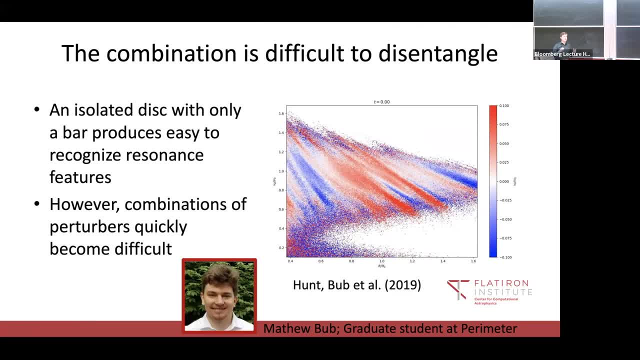 so you could measure it. however, you come just looking at this: yes, go ahead. can you say a few more words about the simulation we said so. you monitor the potential and then you have ways to mimic the presence and then these are really test particles. yes, that's it. this is a 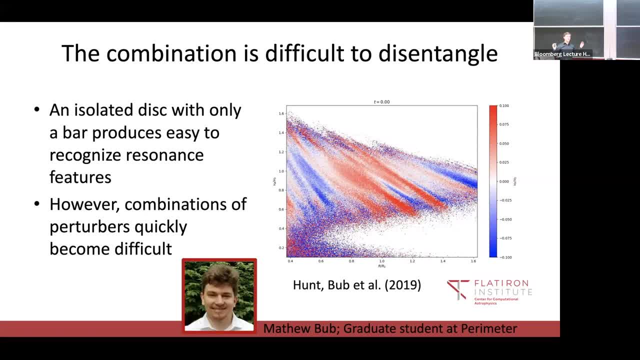 relatively simple simulation. so it's a test particle just just sampling from the equilibrium potential. we impose a bar potential in the middle, which is um. it's like a modifier that increases the density of the inner disc along the bar axis and decreases it. off it and we grow it. 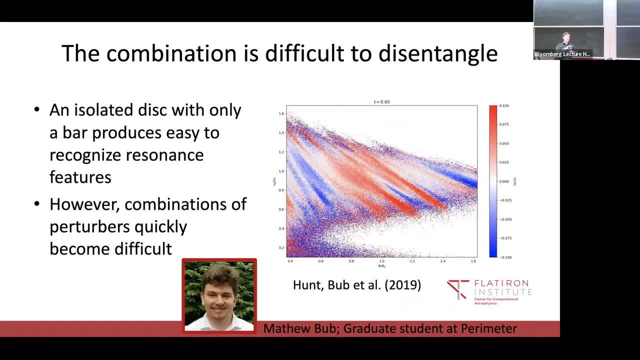 slowly in amplitude and length over time to not just shock the test particle distribution. then we on spiral arms, which are also grown slowly in the same way- this particular instance has transient spirals that are extending from the end of the rotating bar that grow and decay repeatedly. a 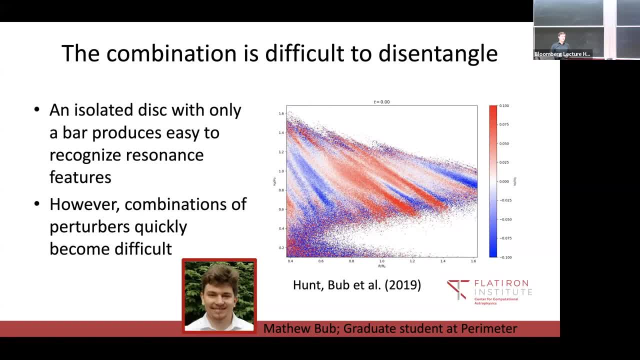 couple of times. you get the same bridges if you have a variety of density wave spirals as well, but the exact patterns will be different. but the broad combination of bars and spirals leads to a messy set of ridges in the space. i'm sorry if i miss this, but the particles they talk to each. 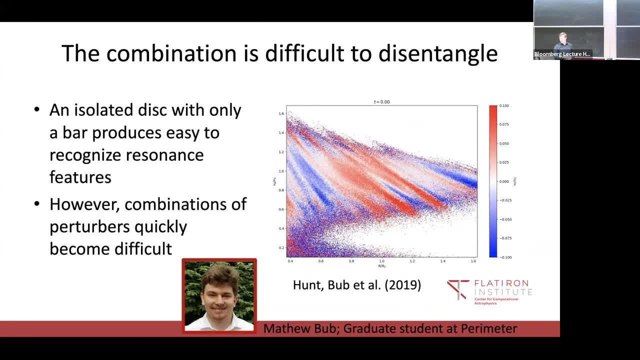 other or just read this part, not in this instance. so the i showed before. this model from francesco franguti is live self-gravidating. they all interact. this one is a toy model to show the. to show when everything is clean, with just the bar, without the soft gravity. 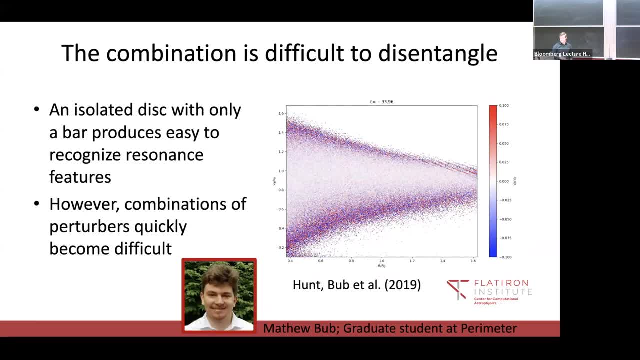 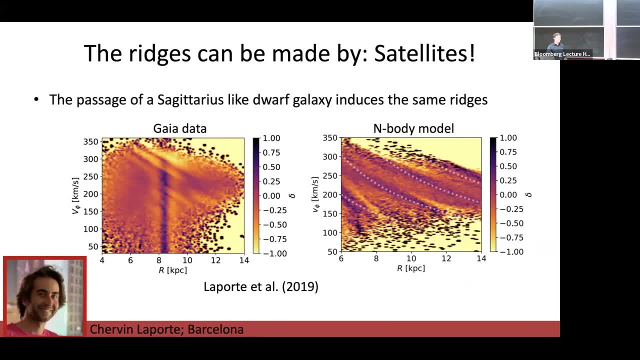 but yeah, we'll come back to self-gravity models later. and yeah, and just to add further, these ridges in the space can also be made by the impact of satellites on the galactic disc. this is a another live and body model from sherman. he has another projection of the 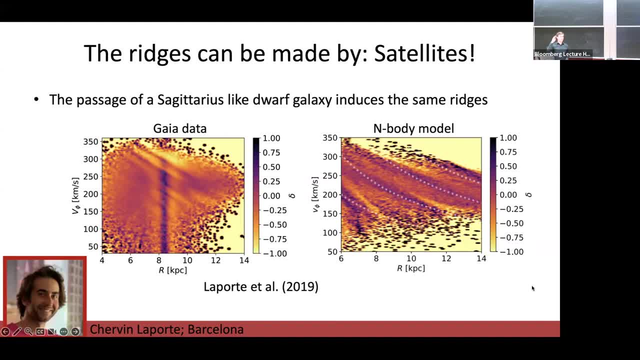 candidate on the left and these ridges are here, and when he drops a dwarf galaxy into a body disc, you make the same ridges. however, in this instance, you're really making spiral arms with the impact of the galaxy, which then make ridges. so how you disentangle it as a bit more of a gray area, but 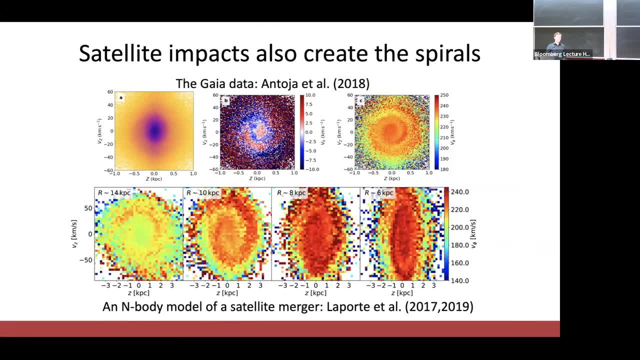 the advantage of the satellite impact model is that it also makes these phase spirals instead, which don't necessarily arise in the other models. so you have here again the guy: data from teresa and toya, on the top, the spiral in density, rate of velocity and azimuthal velocity. then in chauvin's model, you 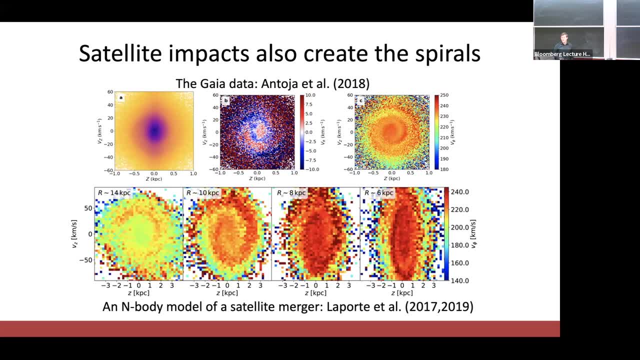 can only see it in azimuthal velocity because there's just the resolution of the model is not good enough to sample a local volume and recover the spiral in the density space. you just don't see it. however, this is from 2017 and with more advanced computer hardware and like more um. 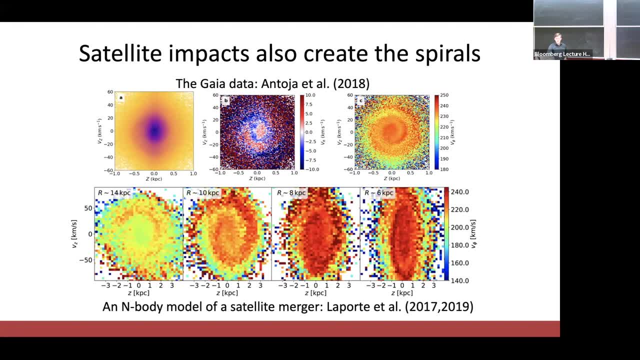 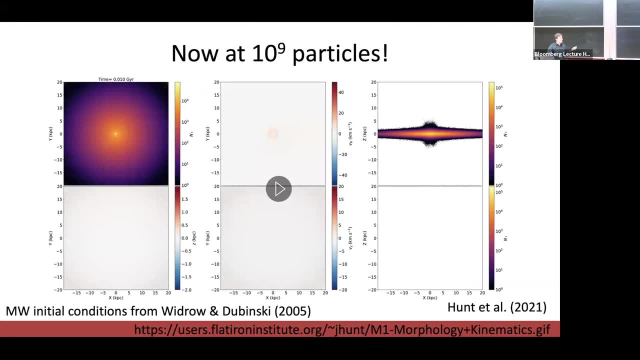 but developed m body codes, you can now get up to much higher resolution. so sherman had about five million particles in the disk, i think 50 million overall, and so i've run this new model: um a billion particles overall, 200 million in the disk, which starts to give you the resolution. 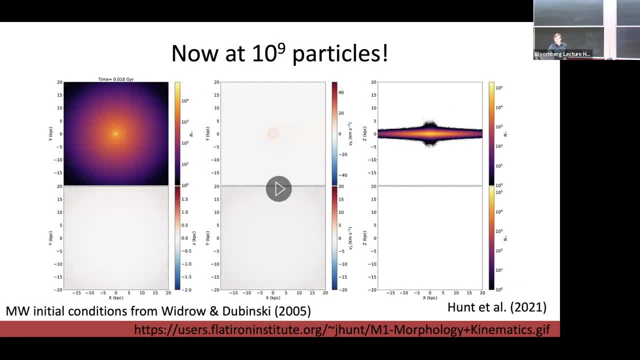 necessary to resolve features over local phase space. so this is? this is a self-permanating model. it's still to some extent a toy because the disc is very warm. it's very stable. it's not meant to perfectly reproduce the milky way. this is supposed to be a laboratory for an 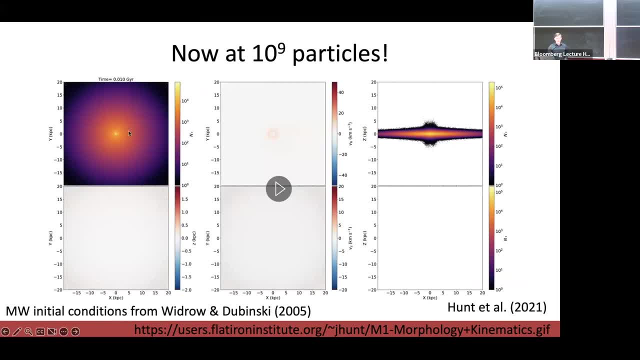 investigation you have here on the top left surface density of the disc. this will be the radial velocity motion of stars inwards and outwards. this will be the mean height above and below the disc plane. this will be the mean motion of stars up and down. this is the edge on. 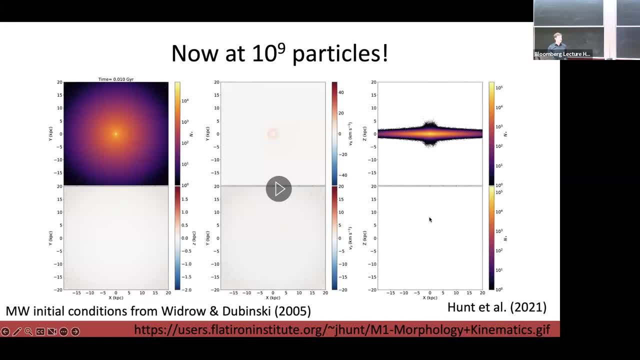 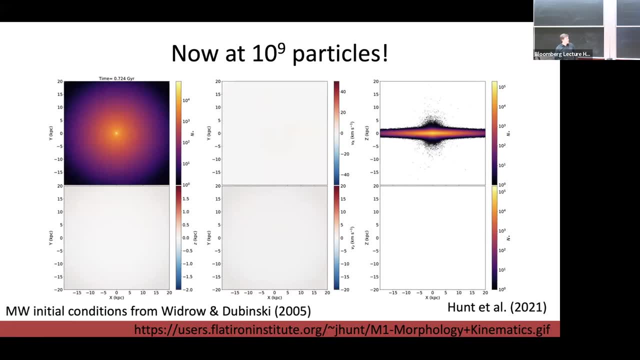 view of just the galactic disc intensity and you will see just the satellite in this bottom panel when it comes through and official conditions taken from widge and the davinci's 2005 paper where they set up this very stable disc, the dynamicis in the room. it has a high tumor cube. 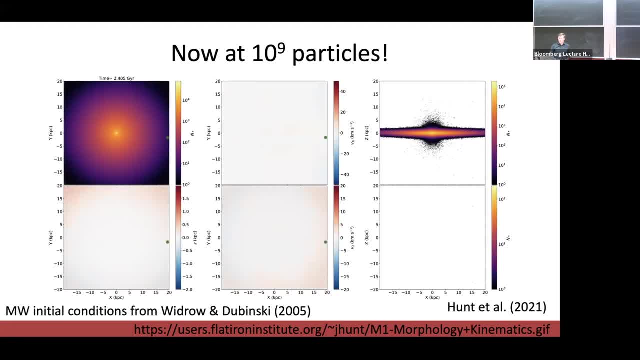 and the disc correction is light. so, yeah, it's not particularly milky way realistic. but then you see the satellite go by, you generate a lot of spiral structure and the density generate a lot of coherent motion in the rate of velocities. uh, the vertical position and motion, and as the 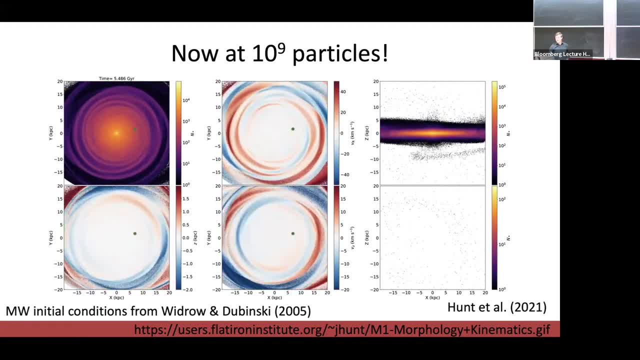 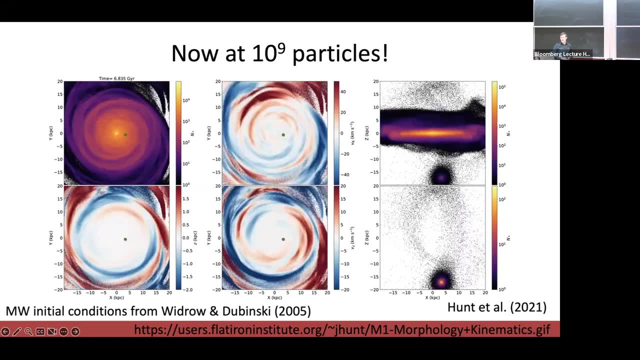 satellite comes through again, you induce structure on top of structure, you start to pull material up off the edge of the galaxy, creating these feathers that you see in the outer disc. and just as the satellite gets further and further in, um yeah, you get more and more dynamics and at the end, this bar starts to fall in the middle of the. 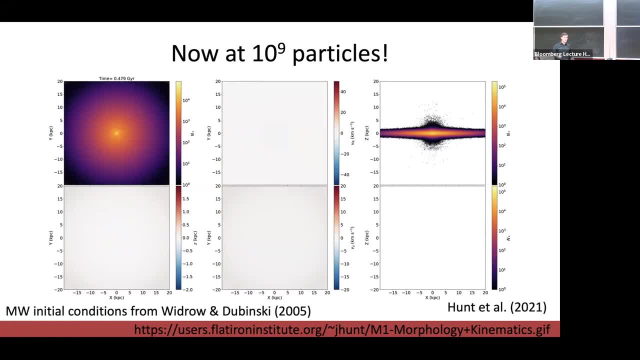 galaxy, so plenty of people can run these kind of n-body satellite merger models. the thing that makes this interesting is the local phase space resolution once you start to investigate the spirals and and. to be clear, this is not the milky way sagittarius system, but we're still going to. 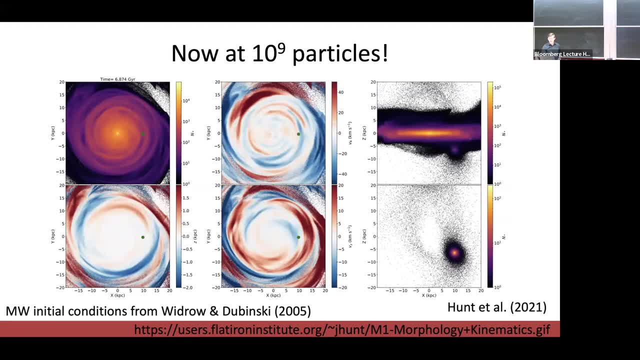 choose a present-day snapshot and look at it and prepare for the guy data, and we choose the moment when the dwarf is about to punch up through- uh, the far side of the galaxy from our chosen solar observer to put it in a more dynamic position, and then we're going to start to look at it from the 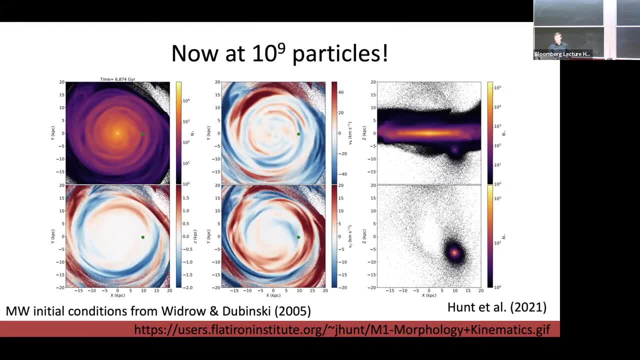 same place as the sagittarius dwarf. today, however it is, the dwarf is more massive and the disc is too far. we shouldn't expect to perfectly reproduce the multi-way system. we also choose this snapshot because it's before a bar has formed in this galaxy, so that we don't confuse future kinematics. 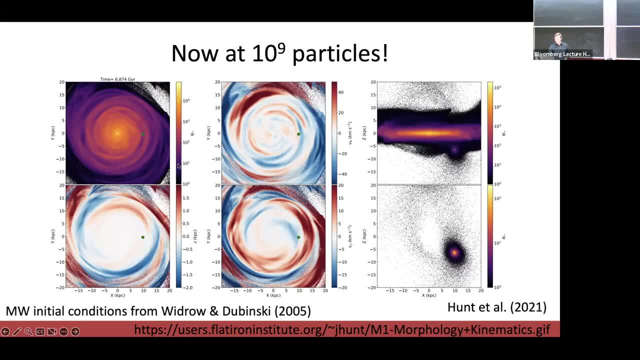 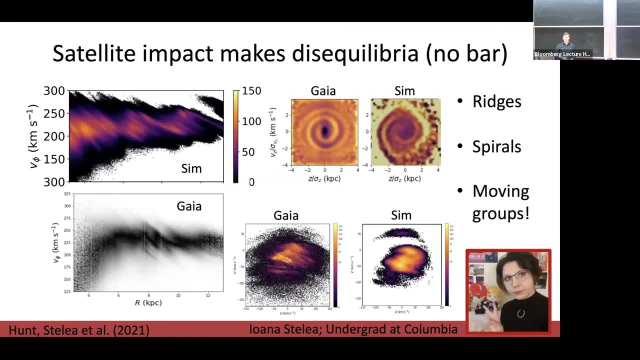 that we're looking at to erase from the bar. of course the multi-way would happen and, interestingly enough, satellite impact makes all the disequilibria features that we see in the disc um. again, it should perfectly reproduce the in the disc um. again, it shouldn't perfectly reproduce the. 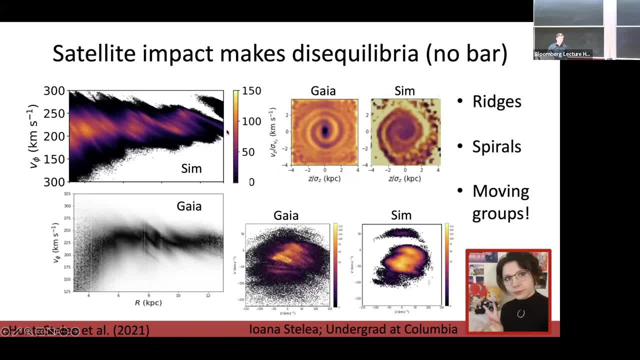 produced that. this is the guy data. this is the simulation. you have all these ridges in galactic radius as a move for velocity. we have this phase spiral in z versus vz. the guy data simulation is not quite as well. wound doesn't match morphologically but again, it's not the 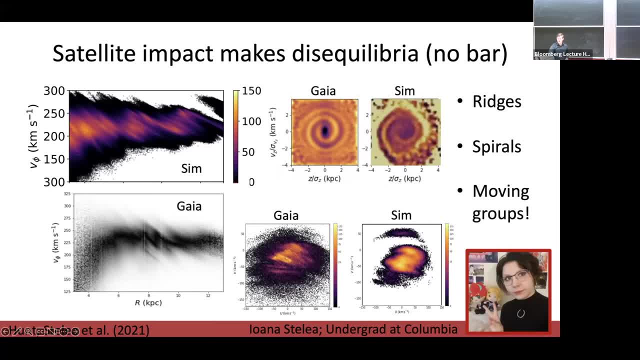 same system. it's qualitatively right. but the thing that was interesting, and we totally didn't expect, is you actually do a really good reproduction of the local solar neighborhood. uh, classical moving groups. this in gaia. you have again hercules, heidi's bodies, cranberry, c's syria. 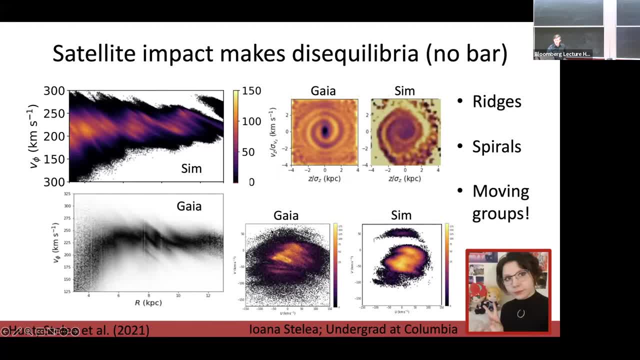 this in this like trimodal main mode at the bottom and the- the faint hat feature on the top. we actually got all those out without trying to. we have the trimodal uh main part of velocity distribution with the correct vertex deviation. we have our separate hercules moving group and 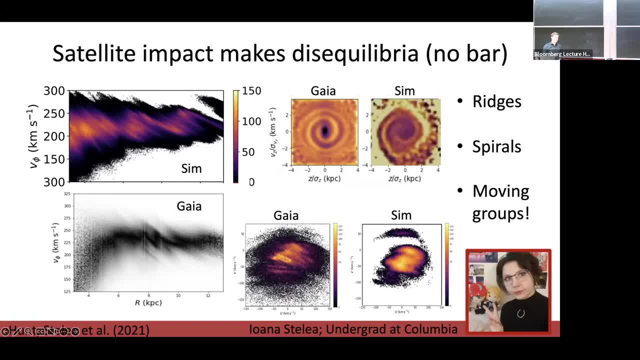 we have our hat on the top. i'm definitely not claiming that we have found the origin of the solar neighborhood moving groups. that's definitely not true. this is just a complete coincidence. however, my point is that if you were to look at this distribution, people would frequently use hercules or the hat to measure parameters of the bar, both strength and pattern. 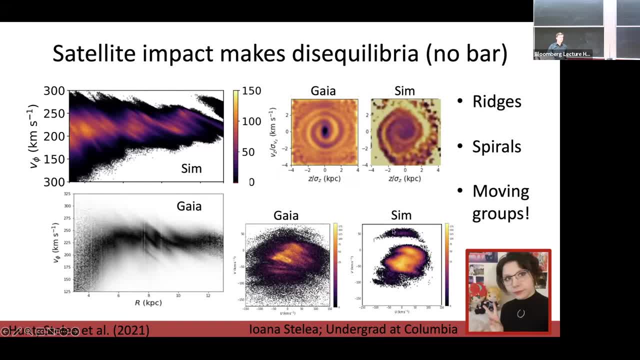 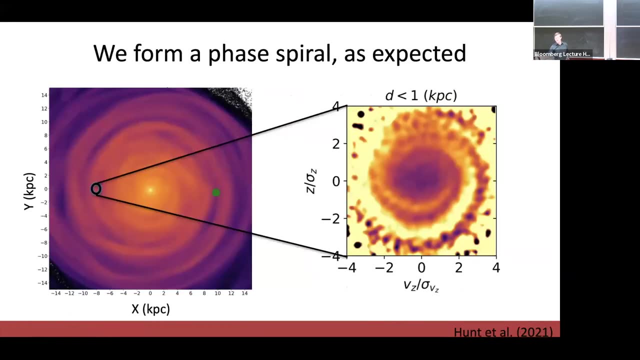 speed. if you made that measurement from this simulation, you would be measuring essentially nothing because there is no bar. if this model just happened to reproduce the kinematics which are often associated with and with that, i will leave the radial and planar stuff mostly behind and start to focus on the phase spiral. so again, in this model we can select a little local volume. 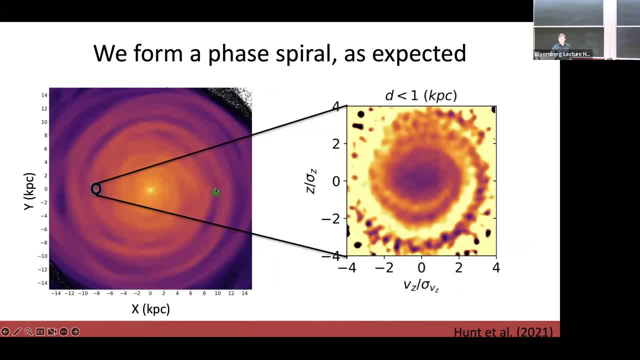 this is going to be our solar neighborhood. in the simulation it's on the far side of where the star is today, which is the green dot. we make this a nice one-armed face spiral, similar to we see on the guy data not as finely resolved, because even a billion particles are still far short. 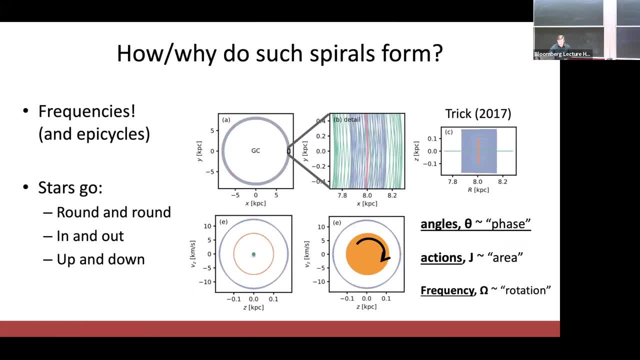 of the reality of galaxy and i'll do a brief digression on how and why these spirals form. if you're not a galactic dynamicist, it's all to do with frequencies and epicycles. so you have this image from wilmot trick's phd thesis on a galactic orbit. there's an 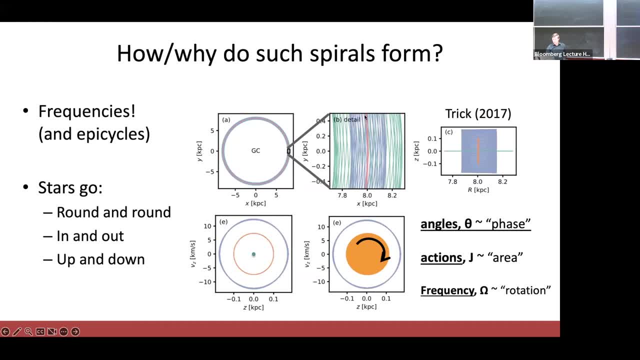 orbital track of stars. they're fairly close to being circular, but not quite. you have this orange orbit here, which is perfectly circular, blue orbit, which has a little bit of radial eccentricity- it crosses multiple radii as it goes around the galaxy- and the green one, which has a bit more radial eccentricity. we are interested in the vertical direction. 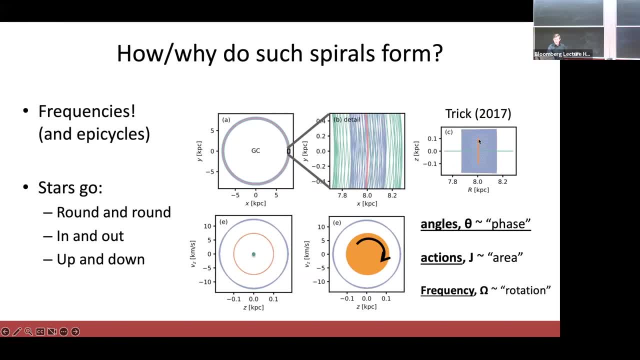 so here this orange orbit. it may be circular in the right direction, but it has vertical extent, oscillates between about 100 parsecs up and down. the blue one has both radial and vertical eccentricity. the green one has a lot of radial but no vertical eccentricity. and so if you map these, 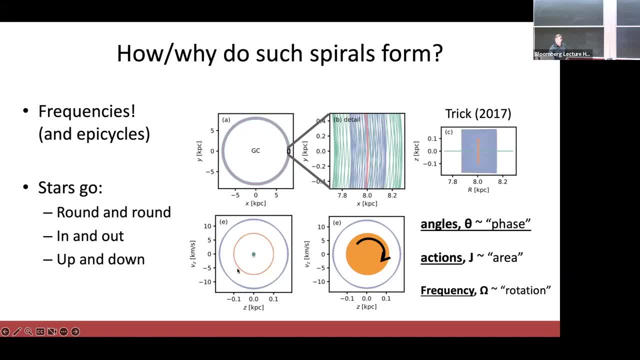 onto the zvz plane that i've been showing. the green orbit, the one that has no vertical eccentricity, would just be a point in the middle. the orange one, which has a bit more vertical eccentricity, would be somewhere in the middle of this and the blue orbit, which has higher vertical. 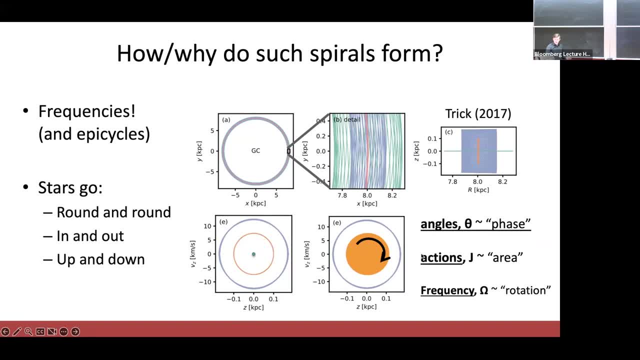 eccentricity, will orbit around the outside. if you're not a galactic dynamicist, you can roughly call actions, angles and frequencies. so the phase of where a star is around its orbit, the action is the area. so the further it is from the center of the orbit, the higher it is from the center of the 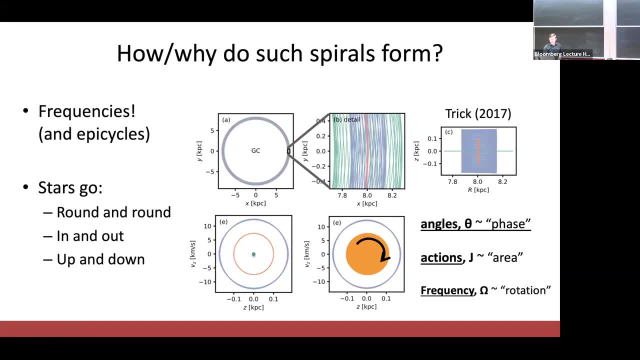 more area it sweeps out, the higher the action, and then the frequency is how it would rotate around this orbit, and stars in the middle will have much higher frequencies that complete the epicycles much quicker than stars towards the edge. so sorry, yes, would i get the rough features of the 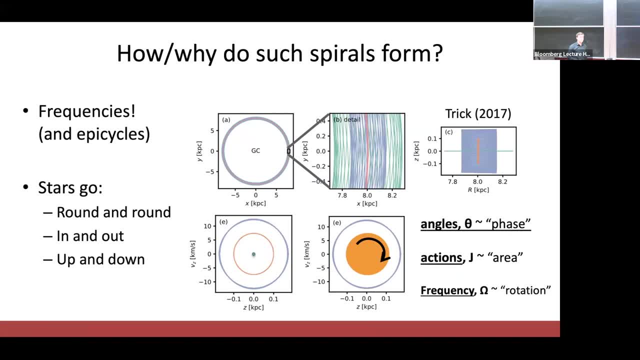 spiral. if i don't, if i only want about that, you can get that in a shooting box or you can answer what part of the global dynamics actually are critical to get this. people have done it in the, the sharing box. all you, all you need to make the phase spiral is some perturbation away from. 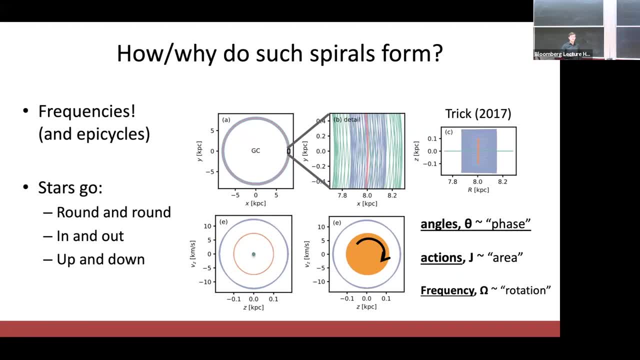 equilibrium and it will wind up into a spiral. so reproducing the correct spiral- the milky way- is much more complicated than that, but reproducing any spiral, it's a pretty natural consequence of any perturbation away from equilibrium in space. so i have a little illustration of that um. 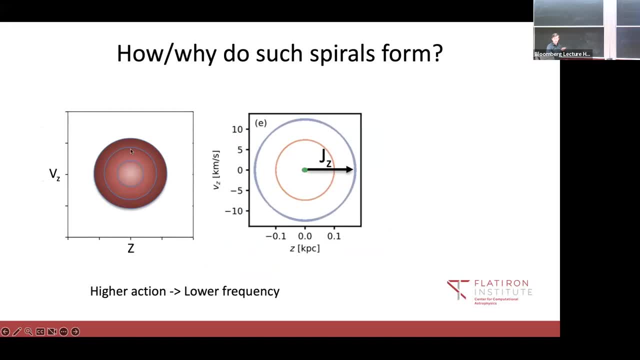 for example, if everything is in equilibrium. this, this distribution, is not quite circular here, but close enough. it doesn't matter that the frequencies are different, they will still look like a smooth, uniform sphere until you distort it. if you pull everything away from the center of the potential, then the stuff in the middle goes around the 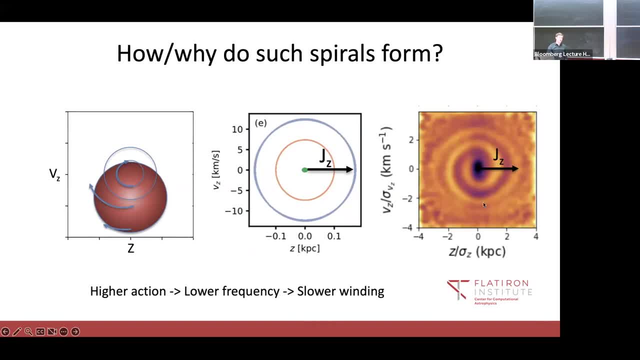 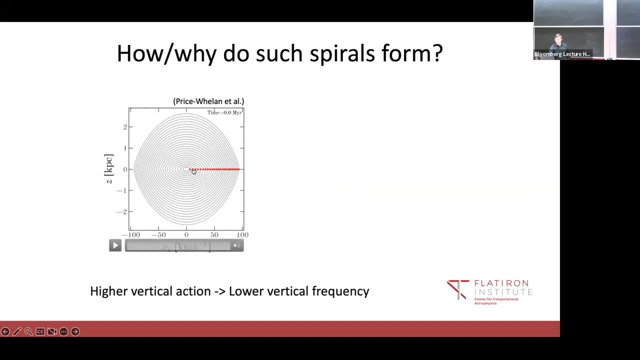 space faster than the stuff at the end and you smear it out into into a spiral. and that's really what's going on here, as, like a basic illustration, you have this nice animation from agent price whalen, but if you have essentially a full um shift of stars off from the center, 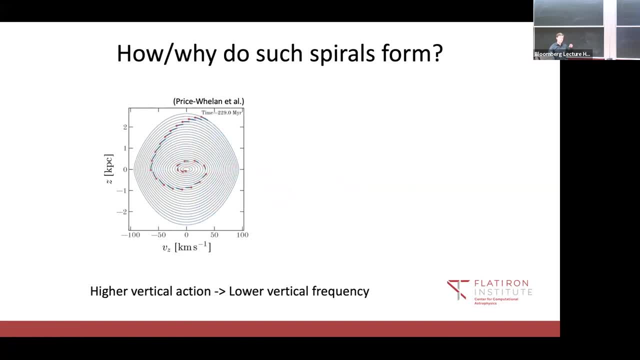 they wind around like this just because the frequencies of stars, in this the vertical frequency of stars in the middle of the space, are higher than the ones at the edge. so making any kind of phase barrel is pretty straightforward and should be a natural consequence of any vertical disequilibria. 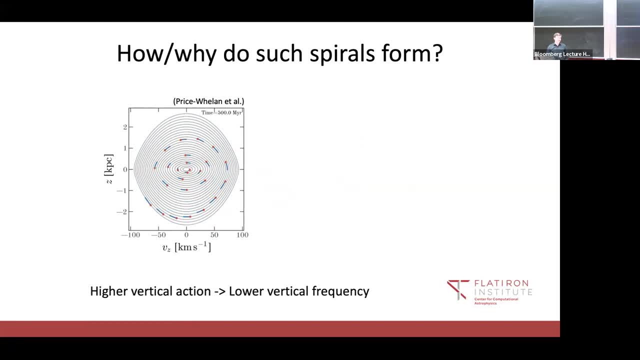 and working out exactly what happens to the guy ones is much more complicated, and that's what i'll be talking about. and yeah, and so over time these wrap into these face barrels and just as an aside here you will notice as i show dots from different groups some people put 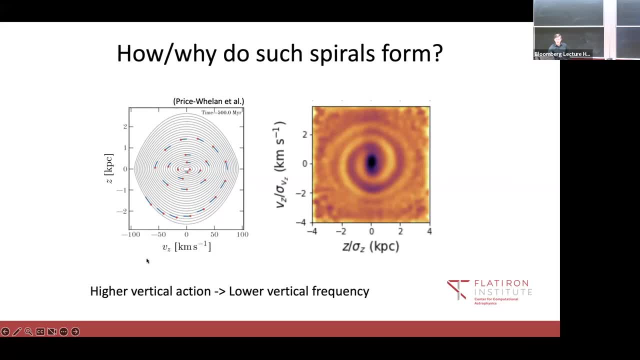 z on the x-axis and d-z on the y-axis, and some groups like vz on the x-axis and z on the y-axis and they feel very strongly about this. personally, i don't really mind, um, but the point to watch out for is that in this instance, you'll get a spiral that's moving clockwise, and this you'll get a. 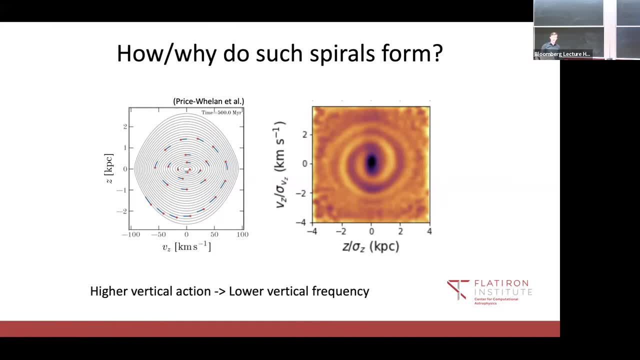 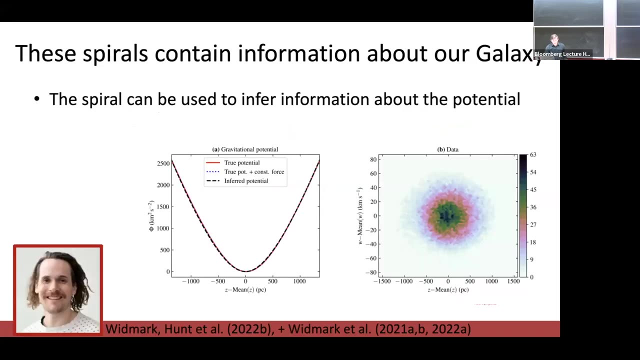 spiral that's moving, anti-clockwise. they're all the same, they're all trailing spirals, they're all phase mixing in the same direction, whether you see, clockwise, anti-clockwise is just the choice of the coordinate system that people use, or not even coordinate system, projection um. and the reason we're interested in these spirals is because they contain information. 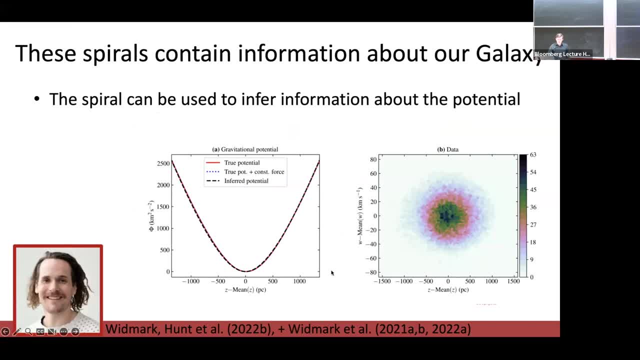 about our galaxy. so it's the study of four papers from excel widmark showing that you can use the shape of the spiral to constrain the local galactic potential. because you know the, the orbital tracks in that space. um, you know how stars should move and if they're shooting out. 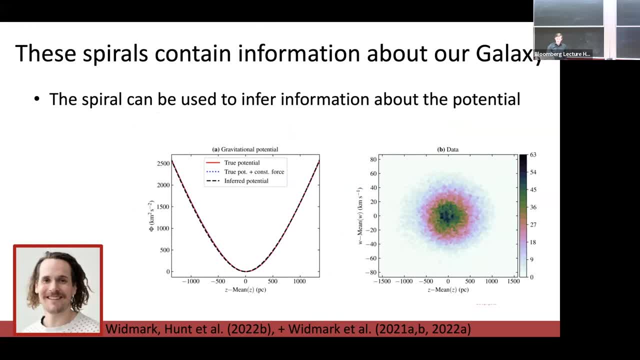 into a spiral. you can kind of back out the potential information. i'm not going to talk in detail about this project. i encourage you to look at its papers if you're interested. but this is the um illustration for the paper we tested on the simulation i just showed you, and even from this: 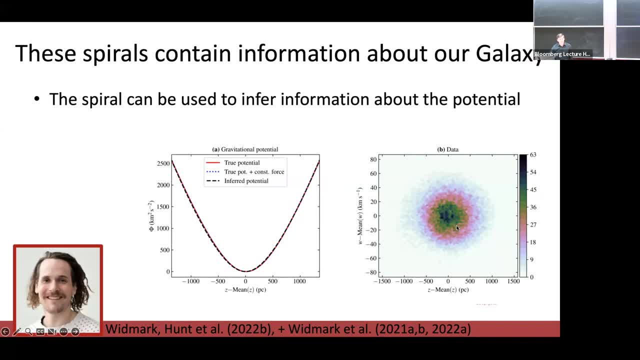 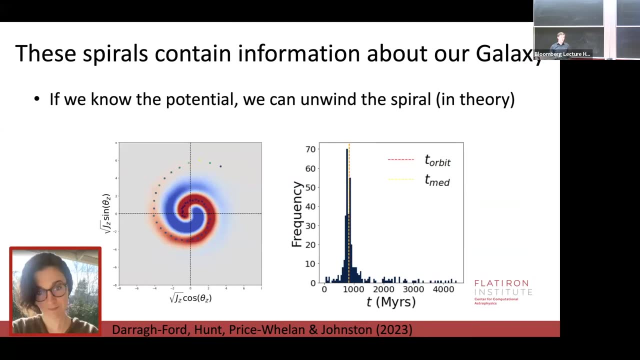 very, almost not a spiral that you can perhaps just about see on there on the right he gets effectively the correctly recovered particle potential in a local area and then if you know the potential you can theoretically unwind the spiral and get information about the origin originating perturbation, such as how long ago it was. 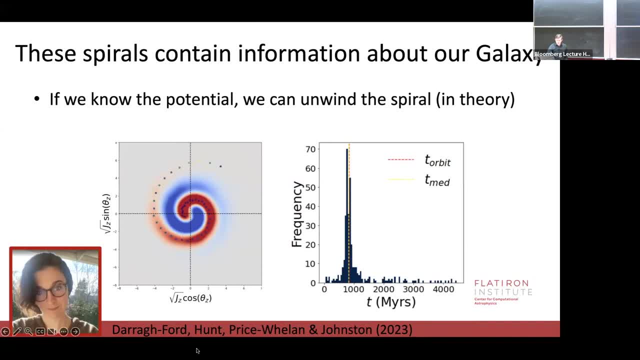 so we have this pilot study from a grad student that leaves direct food where, from this very clean, simple spiral, um, we can then, within a known potential, we can unwind it back and get an estimate of the time when we first perturb that distribution of stars, and she recovers it very well. i think it's 844 million years and the truth is 850.. however, 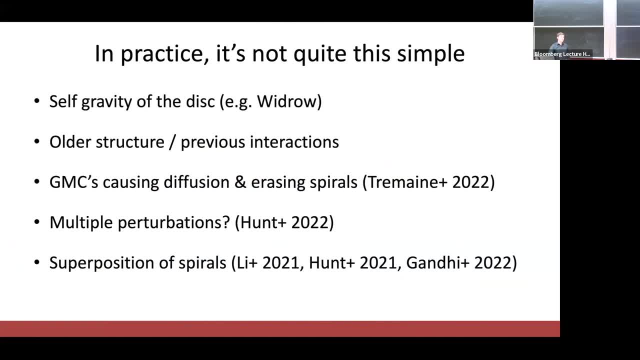 in practice it's not quite this simple. firstly, the disc has its own self gravity. if you distort a bunch of stars away from the mid plane, some of the potential comes with that, because they are creating the gravitational field. secondly, you probably aren't starting from a perma-. 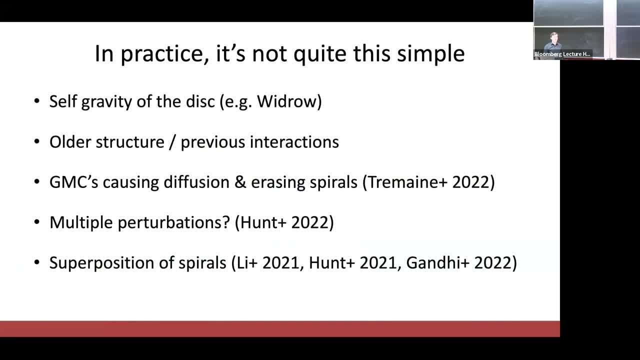 perfectly smooth distribution. you will have had older interactions, whether it's another satellite perturbation or anything else going on, So you don't start from a uniform field, so your spirals can be kind of lumpy. Thirdly, we have the recent paper from your own, Scott Tremaine, showing that 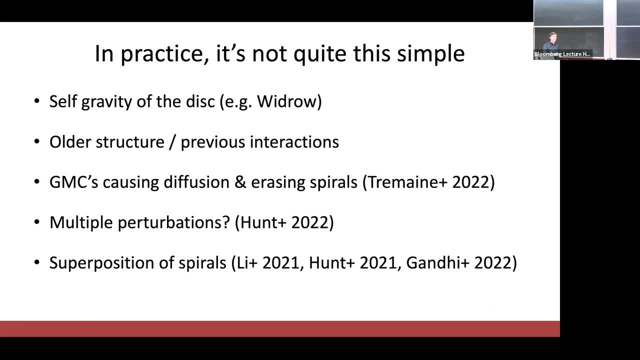 giant molecular clouds can cause diffusion in the action and actually wipe these spirals out earlier than if they were left to wind up by themselves. Fourthly, you can have multiple perturbations going on at the same time. I'll talk about this paper a bit later. You can have multiple spiral patterns. 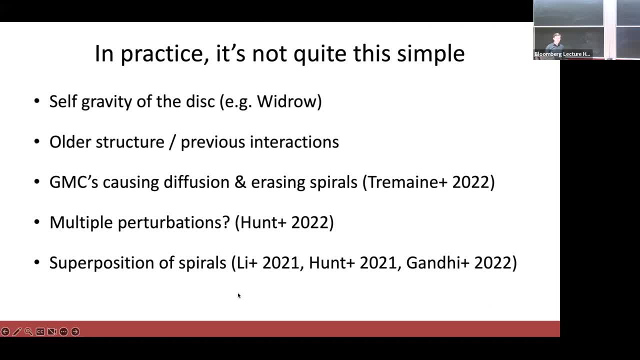 interfering with each other. And then finally, even if none of those things are the case and you have a nice, clean, single perturbation and no GMCs and no previous interactions and no multiple perturbations, you still actually are left with a superposition of phase spirals. 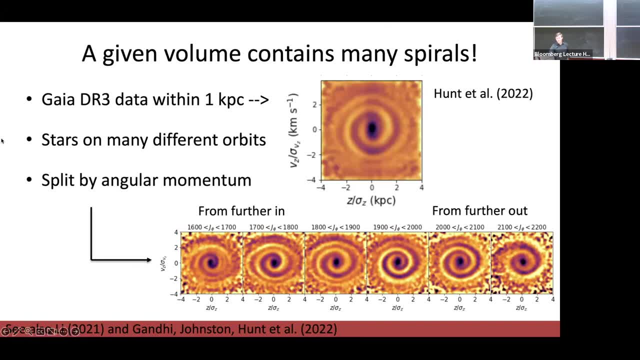 in a local area And that's because a local volume. so this is again the guide. now DR3 data, you see in the density, already pops out within one kilopascal of the sun. this actually contains stars on many different orbits. You have a. 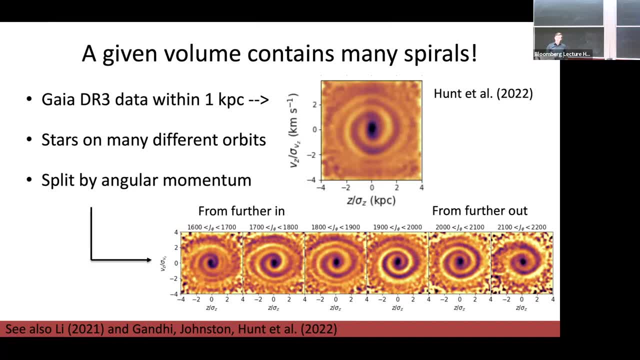 population that are close to circular, which will dominate. You also have many stars that are visiting the solar neighborhood from the outer galaxy on the inner part of their radial epicycles, Many stars with lower angular mentor that are visiting us from the inner galaxy on the 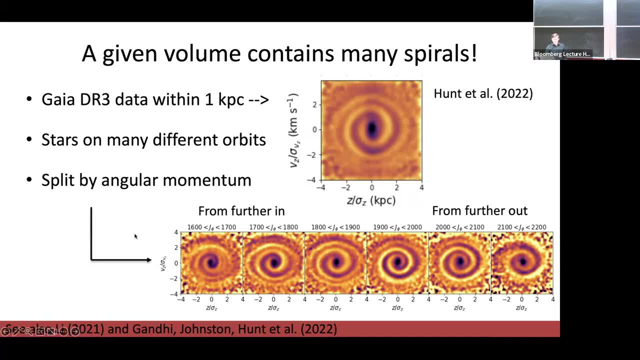 outwards part of their epicycles And if you split this main like local phase spiral by a function of angular mentor, you end up seeing different phase spirals. So in this this is left to right, inner to outer galaxy, split by angular mentor. 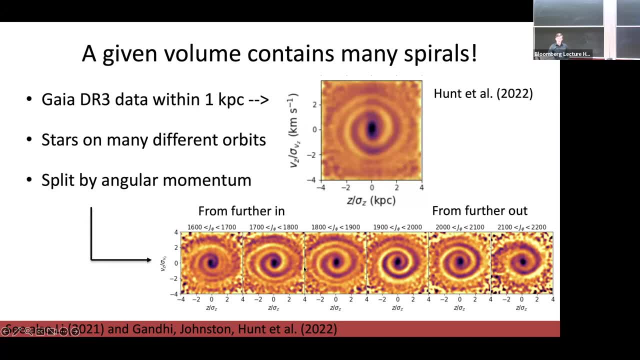 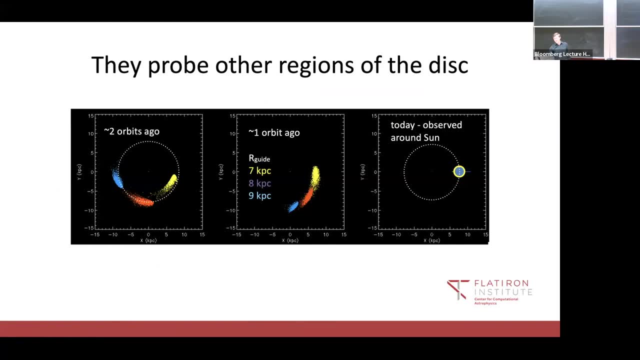 you may not be able to tell much difference between panels directly next to each other in the middle. If you look from the left to the right, you end up with quite different morphology. This is actually a feature, not a bug, because it lets us probe the interaction from different. 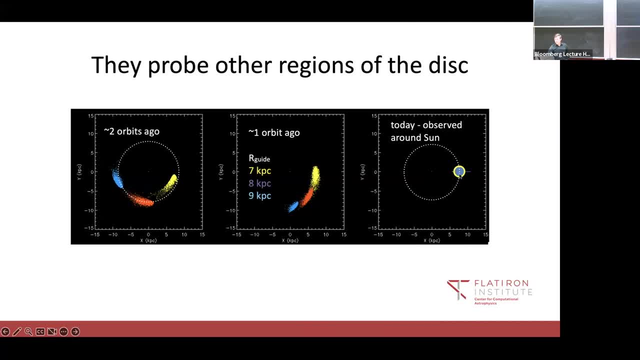 perspectives. If you imagine today, on the right you have this local group of stars. If you track where all of those were one orbit ago or two orbits ago, they can end up spread out far across the disk. If it happened to be some kind of 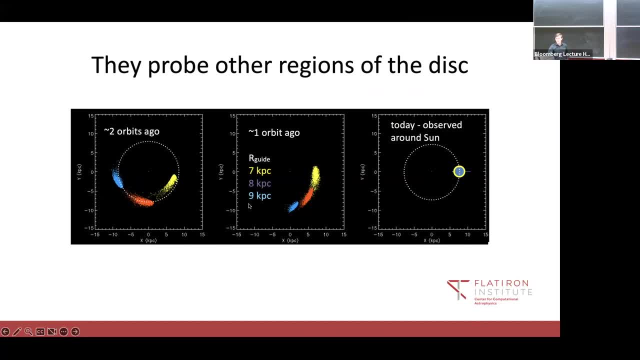 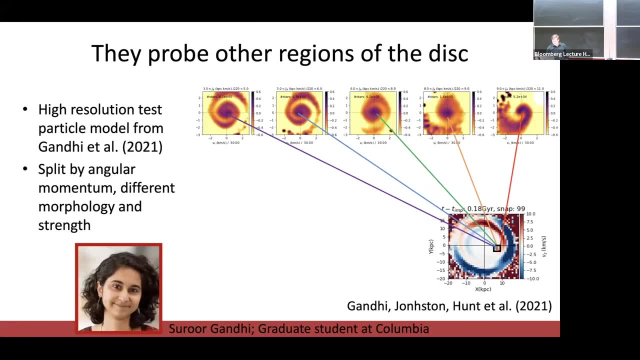 perturbation two orbits ago. you'll be carrying different information depending on what that perturbation was, from a different data perspective back into the solar neighborhood for each day. So here's an example of that. So the model from Surakendi, a Columbia grad student, test particle model. 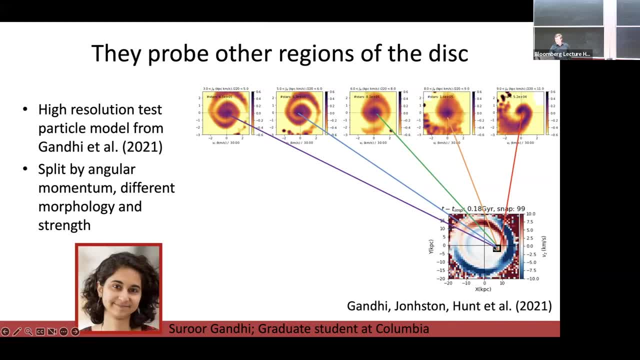 doing the same thing. So this is looking down the face of the disk, selecting a local solar neighborhood and splitting it by angular mentor. You see these spirals have clearly different morphologies: tighter wound from the stars with low angular mentor. less wound stars with high angular mentor, The other. 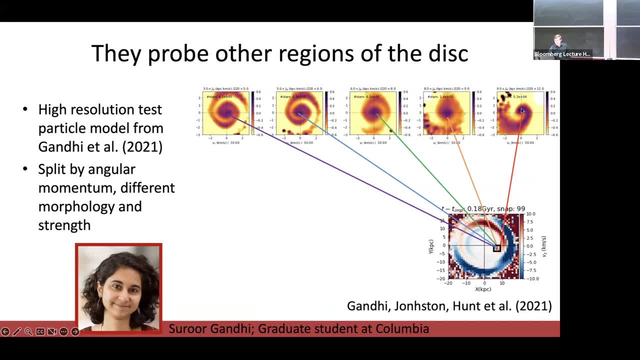 thing to note, this one on the right. it's a little hard to tell in the color bar. this is the strongest amplitude of the spiral And these two are the weakest and these two are the somewhere in the middle. And then, because the simulation you 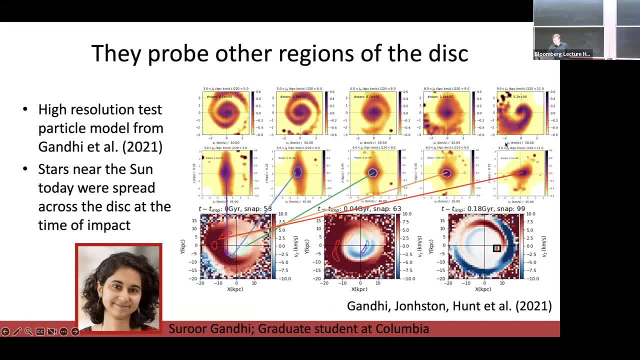 can trace back where they were in the past And we see that this group on the right, the high angular mentor stuff, was indeed further out in the disk It's also pretty much exactly where a satellite passed through the galaxy, So that's where this big 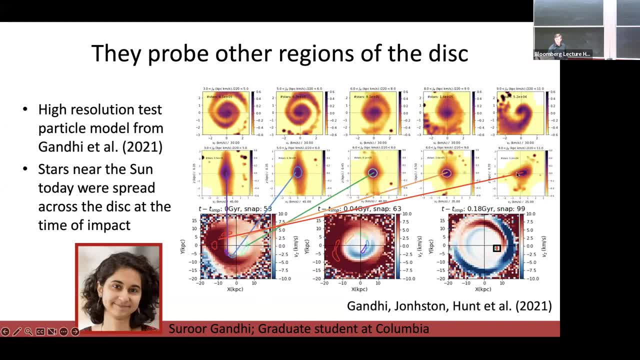 red blob here and this red group was almost perfectly on top of it. Conversely, the green and orange groups are actually at that point on the south side of the galaxy. they had less, less amplitude in the perturbation And they result in a less strong phase spiral And the purple and 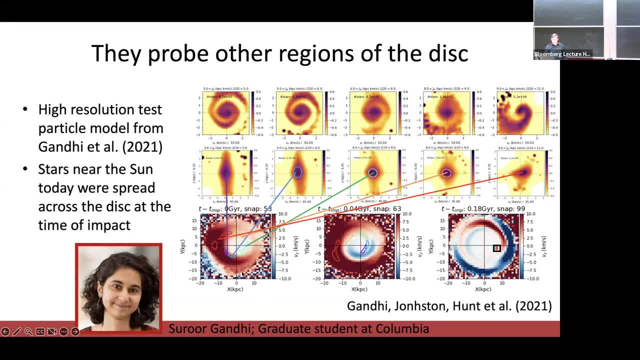 blue ones are somewhere in the middle a bit closer. So that'll kind of make sense. And this is a nice illustration of how, even from a small volume today, you can potentially get information about a perturbation spread far across the disk. The other other 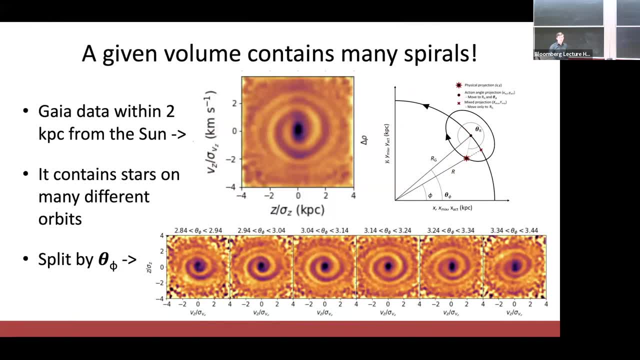 things. as well as splitting by angular, mentor, you can also split by saying the dynamicis, azimuthal phase angle, the conjugate angle to the azimuthal action. For the non dynamicis, this is saying splitting stars by whether they arehte or behind the sun, or beyond the sun on its orbit. So 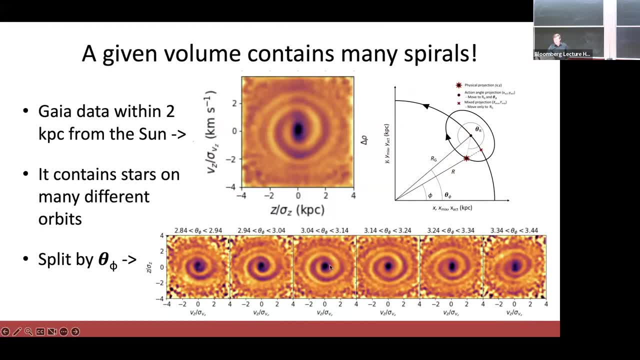 if you do that same, split again panels next to each other, very similar, but going all the way from the left to the right, you see clearly different morphology. So there's also that, that dimension that you can split by And you can do them in the. 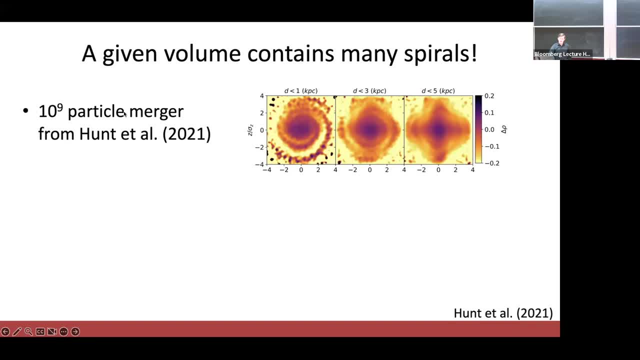 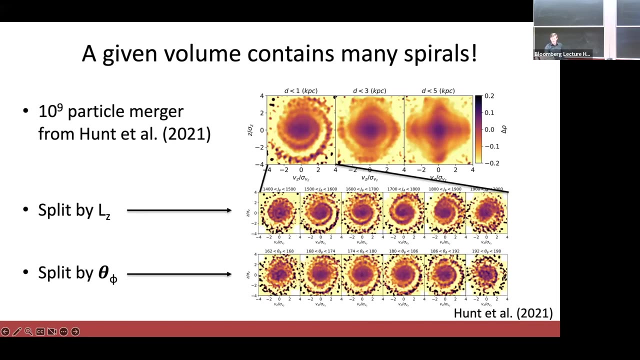 simulations- illustration. So again back to my main big self: consistent merger simulation. one kiloparsec, you get your clean phase spiral. If you go to the further distances it all blurs together more. but even within one kiloparsec you can split it by an angular momentum and as a neutral phase angle and get out spirals of different morphology. However, now we are starting to run into the particle noise from the simulation. even a billion particles is still not enough. 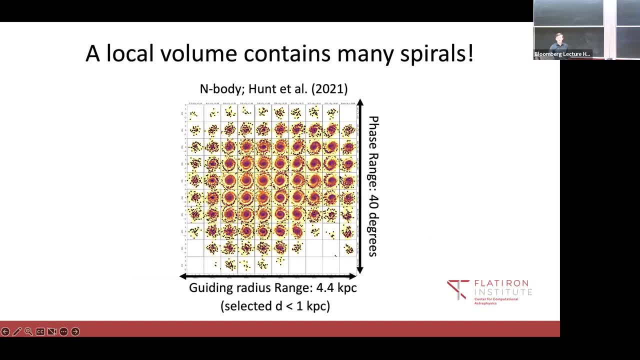 However, if you split by these at the same time, you can start to make these 2D maps of how the spiral varies across. and it's not quite physical space, it's more orbit space. but even from a local, one kiloparsec volume, you can sample phase spirals that have guiding radii of about 4.4 kiloparsecs or a phase range of about 40 degrees, which is much further than you can get when looking in physical space because of selection effects. 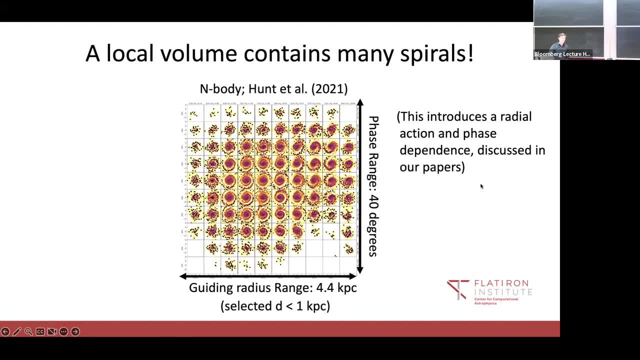 Again for dynamics. this induces a radial action. that phase dependence discussed in the paper I won't go into today. And all of these spirals in this grid that have significantly different morphology in different areas are all contained within this one phase spiral in this one region here in the simulation. 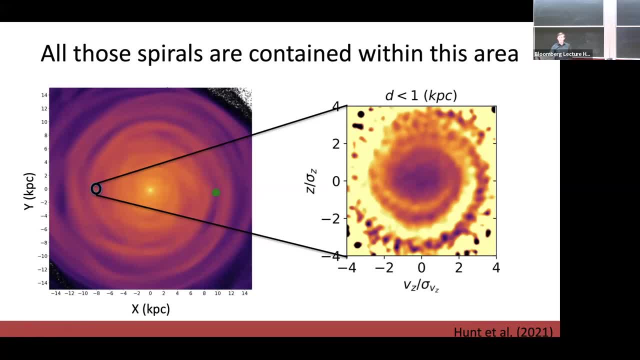 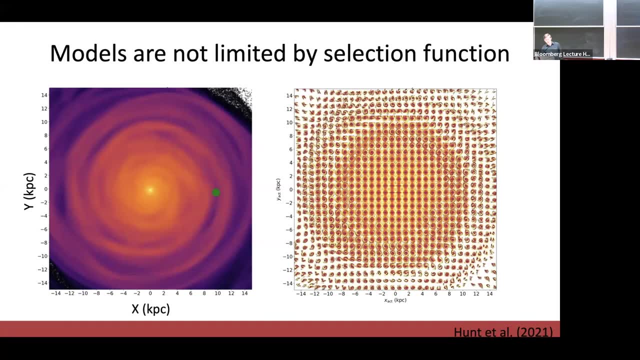 However, the advantage of the simulation is that we are not constrained to the local volume. We don't have selection effects. we can look everywhere, and so you can do this. So what you have now on the right, each of these little tiny spirals, is the phase spiral that you'd get if you took a one kiloparsec box in that area of the galaxy. So this is a 30 by 30. 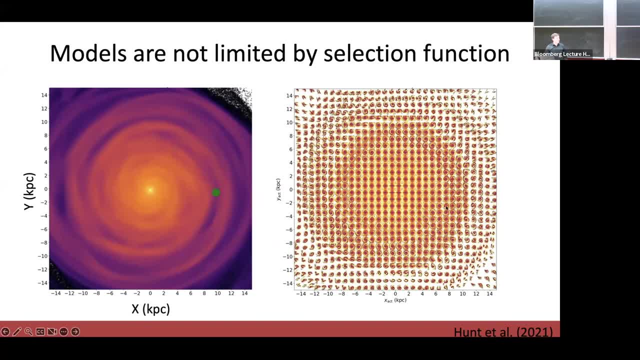 grid of what we call a phase spiral, And this is a 20 by 30 grid of one kiloparsec box sizes and the spiral that you'd see in all of them. This is quite a busy plot. also, I don't know how well they come out for the people in the back, but the three things to take away here. 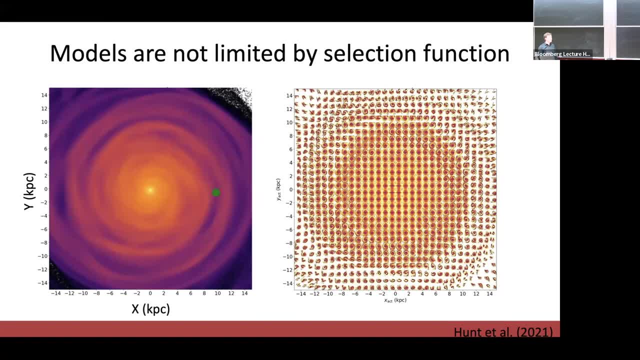 One is: these phase spirals are ubiquitous. The whole galaxy has been perturbed. We're not living in some special area by the sun that just happens to have one. they're probably quite common if you've had any kind of interaction history. Secondly, phase spirals that are near each other look very similar. 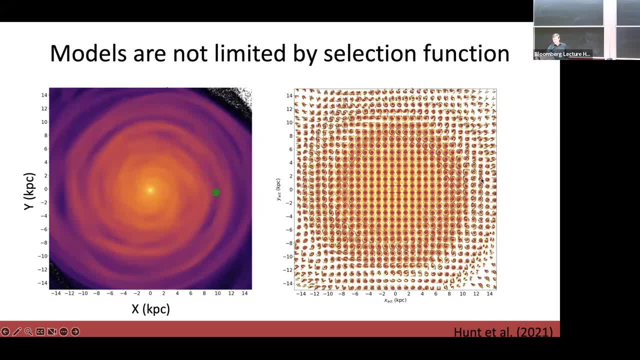 You may have to take the word for it if you can't see them, but phase spirals over the opposite side of the galaxy have a very similar look. So the phase spirals are ubiquitous and they're ubiquitous, So the phase spirals that are ubiquitous look very similar. 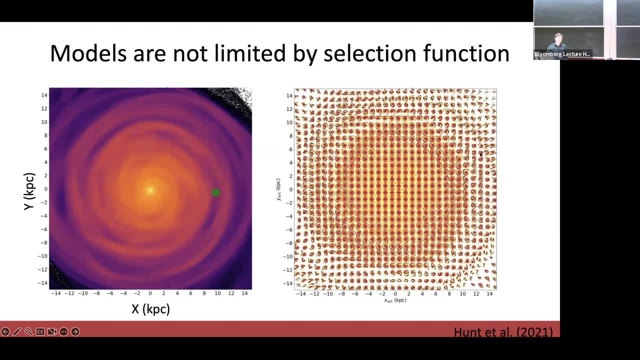 galaxy look very different, although similar to each other in their groups. And thirdly, that if you kind of squint a little bit, the whole thing looks like one big spiral. Why for the big spiral? Yeah, so actually this is a. this is a simpler case. 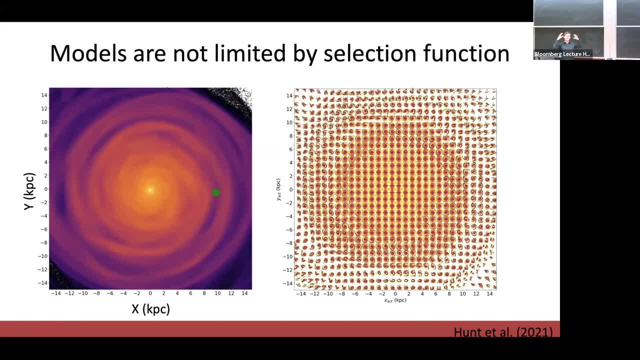 So this is Z versus VZ. So when you're having, say, the entire distribution dragged away from the mid plane, you're going to leave white space behind where there are no stars. So in this image it's the offset of the spirals from the center. 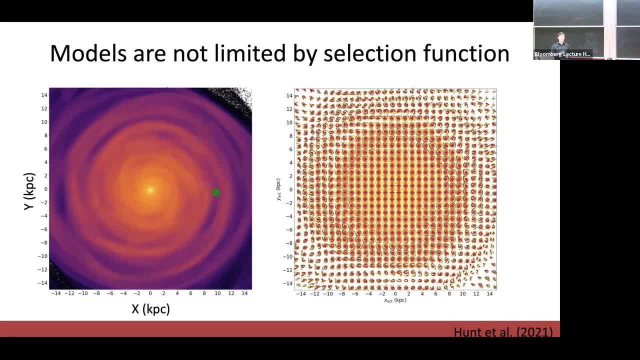 In a coordinated fashion. So if you look at this map compared to a global map of vertical position of velocity, you see the same kind of structure because the big spiral is just offset from the central point of that ZVZ panel. it's departure. 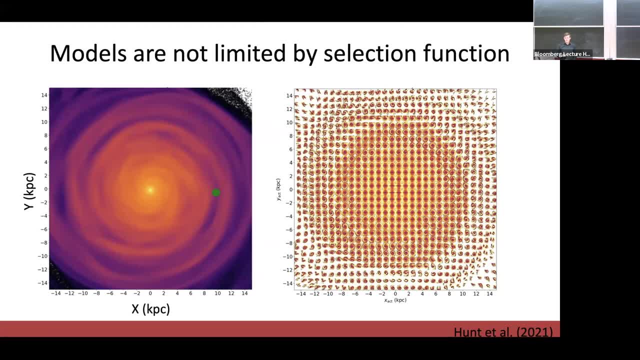 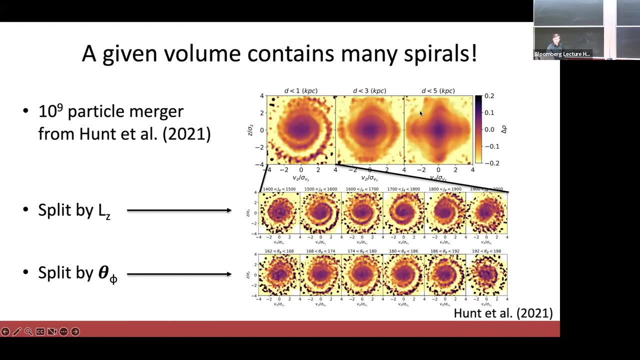 from like the equilibrium state. What would you get if you were to consider the entire galaxy as one? Um, that's an interesting question. I think you'd get something Closer. I think you'd still see some kind of structure, but it will be very messy. 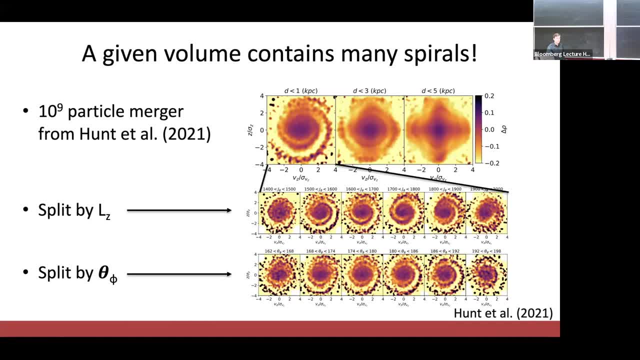 because you'd have a large amount of stuff superimposed on top of each other. I don't think it would go back to just being a uniform ball, but I actually I haven't done that test, I'm not sure. Um, and then, cause I can. I can see everyone looking at this and deciding. 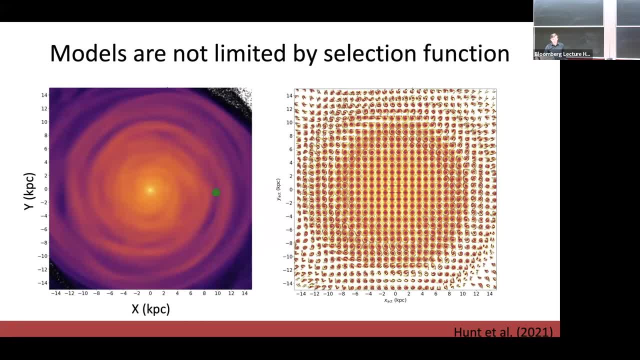 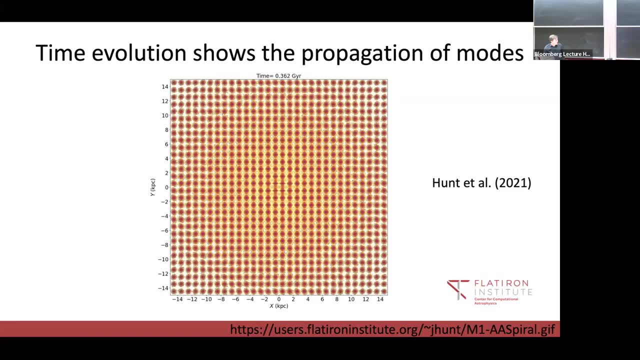 there's really not enough information in this plot and that you'd like more panels. I've added 750,000 more panels in the form of tiny values, So that's the other thing that these simulations can do. So this is that same grid, starting from the beginning. 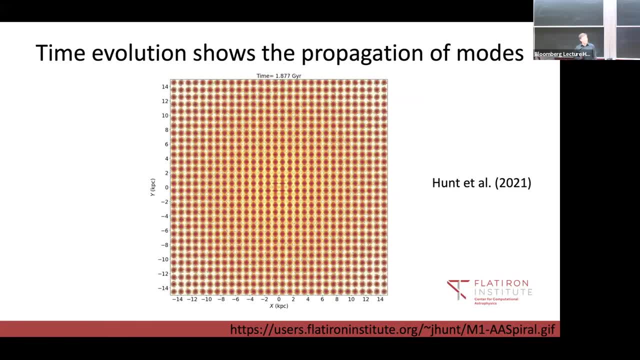 Nothing's going on. It's very smooth, It's very stable. It's lags behind my laptop, So I should watch this one. Um, this is what would happen. is this thing? absolutely no vertical elevation of your disc. Here's when the satellite goes through, you see the entire plane be distorted. 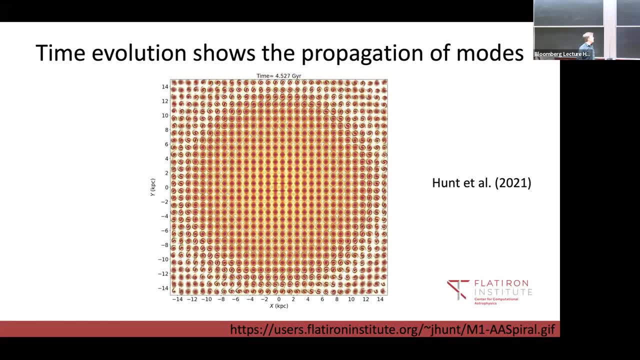 as barrels are pulled away from the mid plane, Stars are pulled away from the mid plane, and then you see them start to wind up into these phase barrels. It's going to propagate across the disc. That's the second Second interaction. Then, um, I think the zoom is struggling with it a little bit. 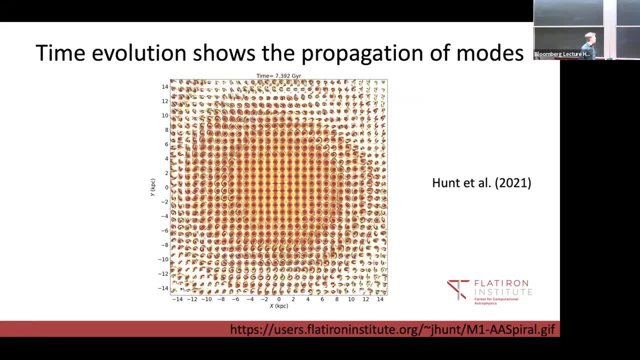 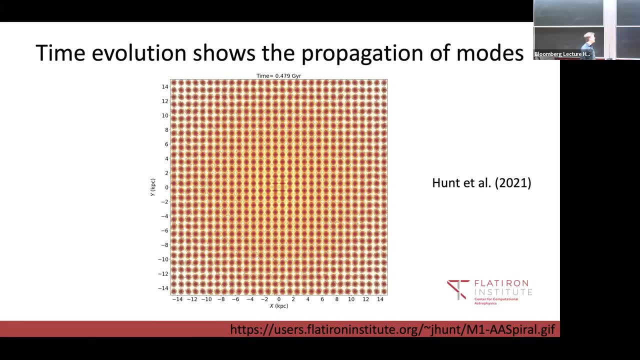 If you want the smooth version, I can pass the link later. but you see, over time more and more spirals are induced on top of the existing spirals. Everything gets kind of messy, Um, but they become your backwards. You know it's the whole galaxy run through once more, because I particularly 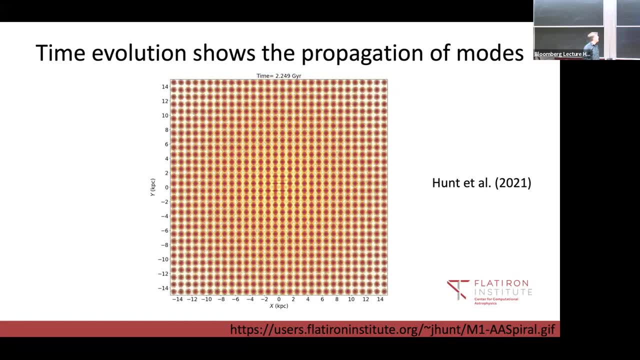 like this, and I have a couple of things to point out. So what is the point of this exercise? I mean, given the position Of the galaxy, I mean, I don't think there is any hope for visiting other places. You'll certainly never be able to make this either in terms of the 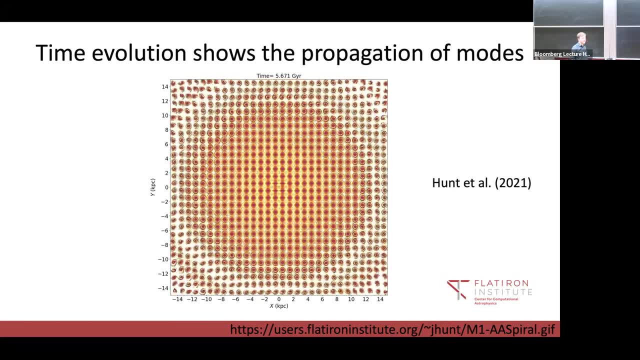 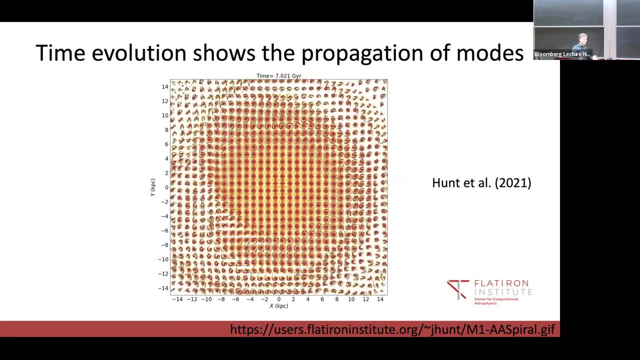 entire galaxy or through time. there I would argue that's entirely the point, because we in our local volume will only have one little sample, or eventually we'll get a little further. we'll have some small regions of sample, but seeing the way that they change, or the properties, 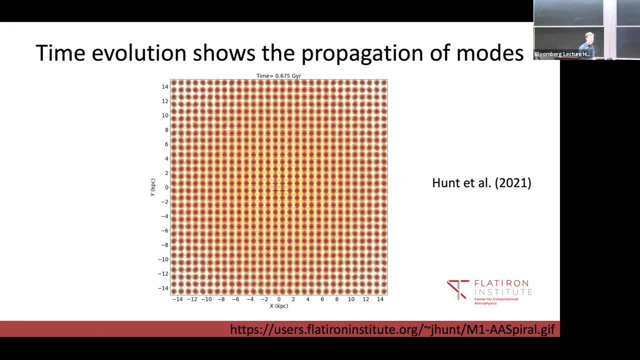 of them in a local volume and actually relating that back to an origin is hard And so having simulations where you can, you can track how these things evolved over time and how they do change. This particular animation is mainly just for fun. It's quite hard to interpret, but the individual panels and how the like 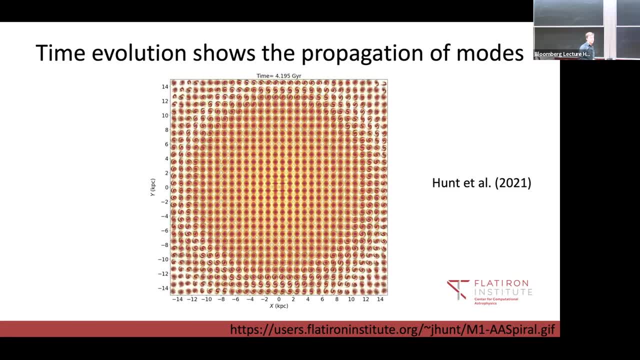 statistics you can do on the spirals over time, I think are quite important because you can't be, absolutely cannot do this with the real data And it's a freeze. on a couple of points to show what we did learn from this ridiculous animation. 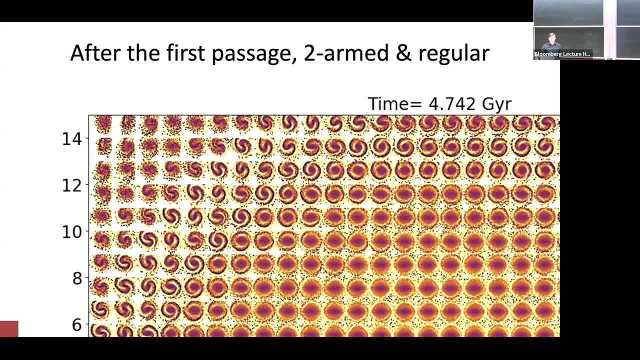 I guess after the first passage you get this ring of phase spirals which are all very regular and they're also all too odd. So this is a little band and not quite the fully out of desk but further out from the sun and and all very regular, very similar. 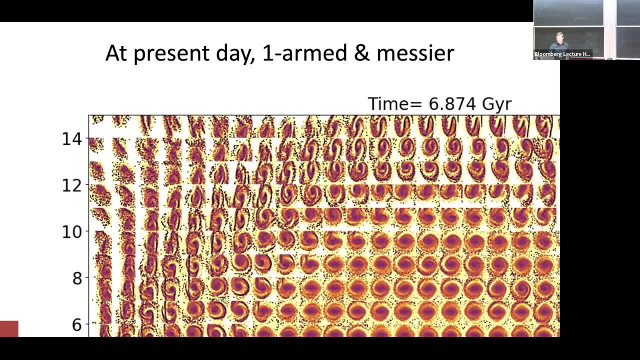 And then later on towards the present day snapshot that we chose. then you end up with these one on phase spirals close to the solar radius, Like we see in the actual data, and the outer galaxy has become a big mess, And we know why this is so into the nature of the. 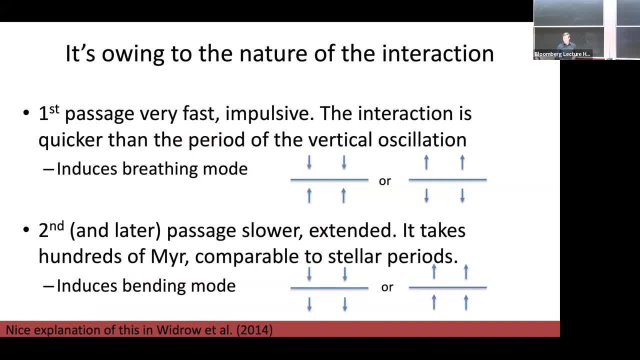 Interaction. that first passage is very impulsive, is very fast. It's impulsive. It's: the satellite goes by the edge of the desk really rapidly- faster than the vertical oscillation period of the stance- that we have a chance to go anywhere. Basically, just inject energy into the space and it induces what's called a breathing. 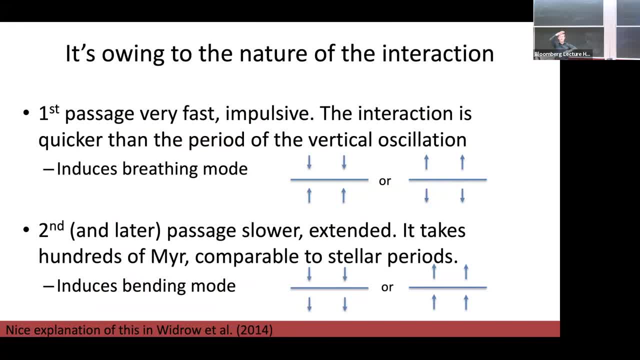 The stars above in the desk are going oscillating up and down like that with respect to each other, And then the second passage and later pastures, again slower than we're, extended like sweet under the desk, take a few hundred million Years. 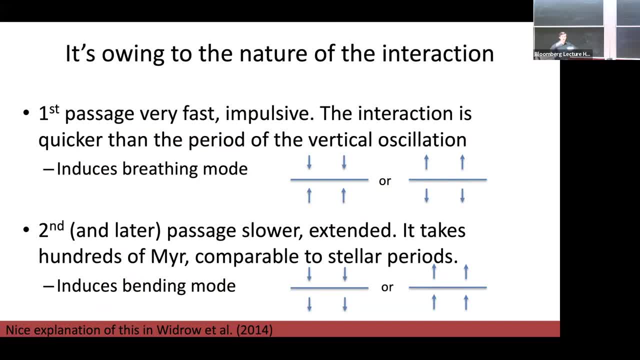 And then do something that's called a bending mode, where the stars are moving down and up like that together. Can I ask? Yeah, So what would be the if you were to have a read to her? consider the gas galaxy. how would this play with the energy dissipation when you? 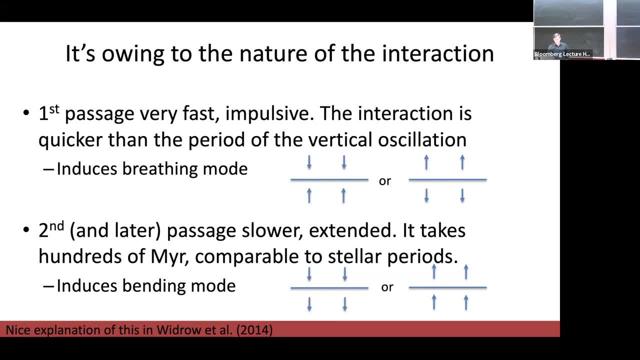 Yes, that's a good question. At the moment we haven't been able to include gas, primarily just because of resolution questions. If you want to resolve lots of local phase spirals with simulations, it's difficult. Um, But two ways. One, I think the thinner, the thinner gas potential will give you a small like. the extra little thin layer of the potential will change slightly the inner regions of the face barrel and how they mix, but also stuff like the giant molecular clouds and other 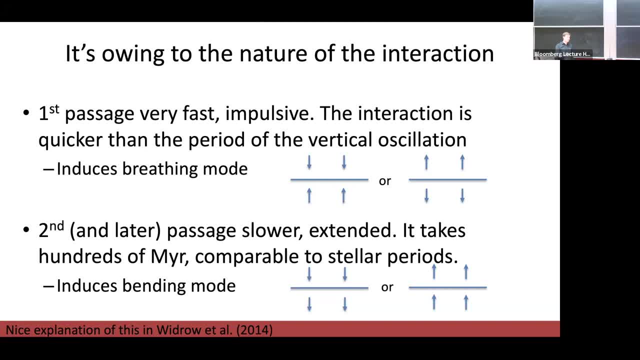 Real physics that we don't have incorporated into the same bodies will do stuff like a special type of shows. do act diffusion help like these acts sooner? I think so. The behavior won't be exactly the same, but I think it should be qualitative. 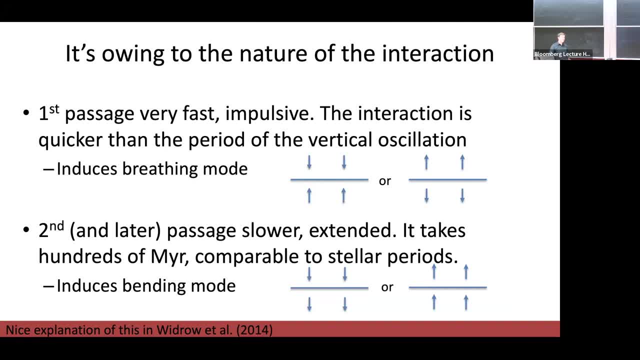 qualitatively the same, but we're working towards that. I have um. I have a hydra simulation running at the moment which has 100 million particles in the disk, so we should be able to compare, but it's taking a long time, as it should do. 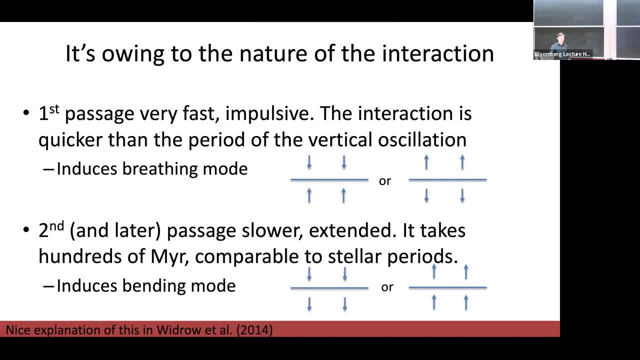 So I might be able to give you a more satisfying answer next year, but not right now. Is this a high QQQ galaxy? Yeah, this is. this is very um, this is very hot. We have run the same models and mergers, et cetera, with reasonable Milky Way like. 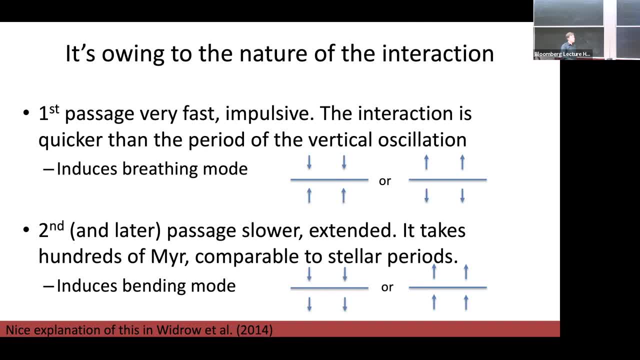 disk galaxies and you see qualitatively the same structure. The reason I show this one is because this is the only thing that's going on the satellite, whereas other galaxies- as I'll talk about later, when you have a bar and spiral arms that generate. 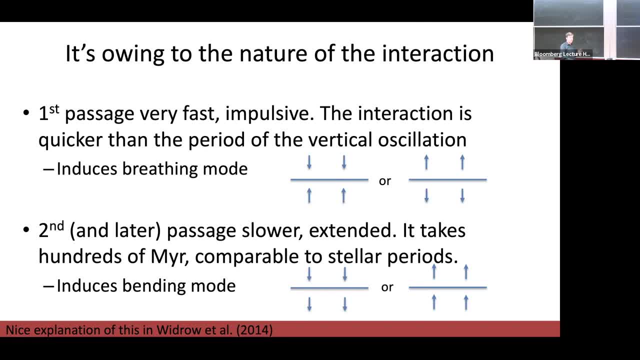 breathing modes, self-consistently with bi-internal dynamics, also make phase spirals, and that's what I'm talking about when I say multiple perturbations can perhaps interfere with each other. So this is a clean laboratory for looking at one origin, but it's not. 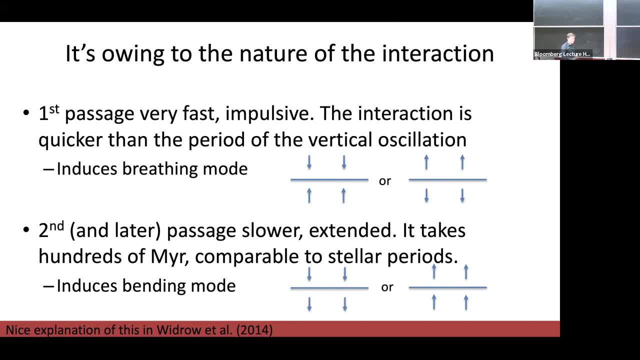 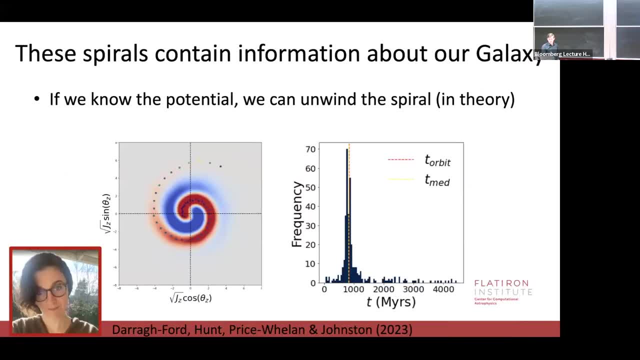 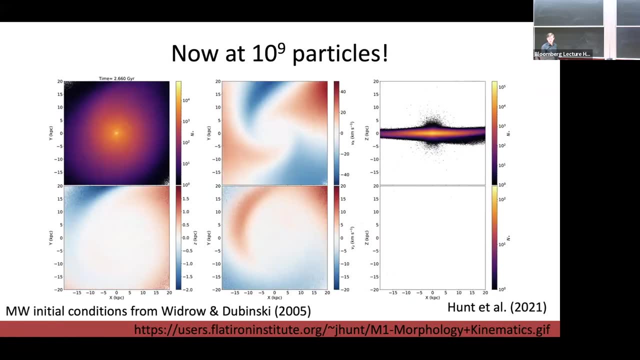 as realistically Milky Way-like as other ones. The response: this response probably depends on too much QQQ. It does, and you can see it in the. I might jump all the way back to: yeah, this one. You see, from that first impact, as you have the spiral arms induced and they propagate out, it's very clean, nothing's clapping under itself. it's very the same as the true of the. 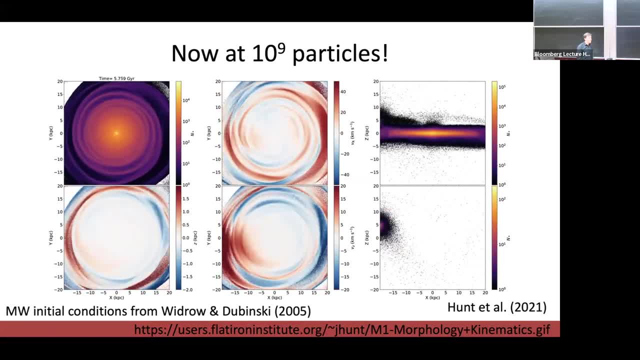 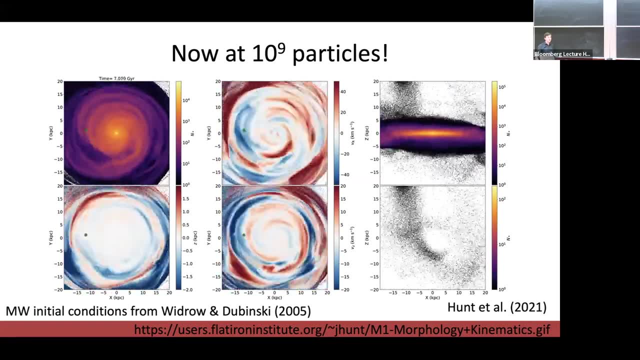 the vertical position of motion until you get later on. So, yeah, it will change things, But like, qualitatively, the grids of spirals, you can get in more realistic Milky Way galaxies. they still show the same behavior. So it depends on exactly what question you want to look at. 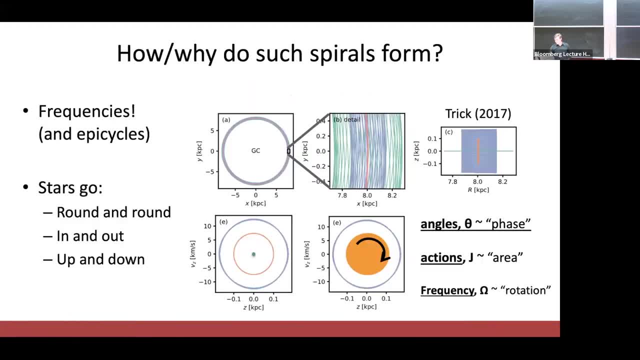 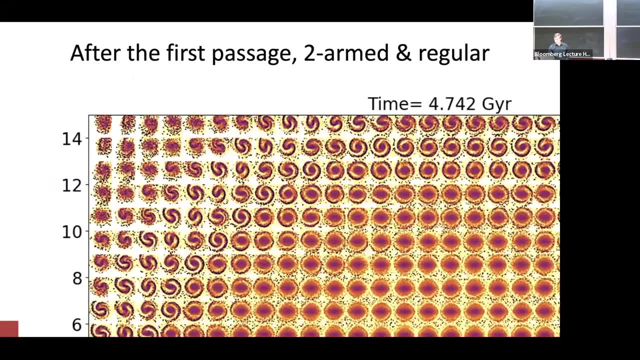 I guess I'm sort of telling the question about the addition of gas, because the addition of gas typically does lower tumor Q, so that will amplify these effects. I guess, Yeah, gas should be included. it would be more realistic. it's just computationally difficult. 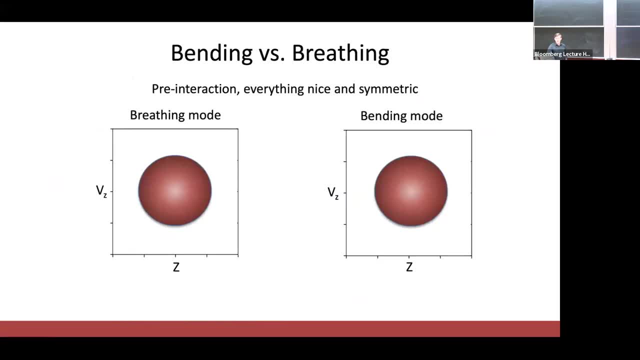 And yeah, for the breathing and bending modes, just again going back to this cartoon of how they form: Bending mode is essentially dragging stuff down, the breathing mode is essentially stretching it out and then they wind up into one or two armed face spirals as they are departing from equilibrium. so that's. 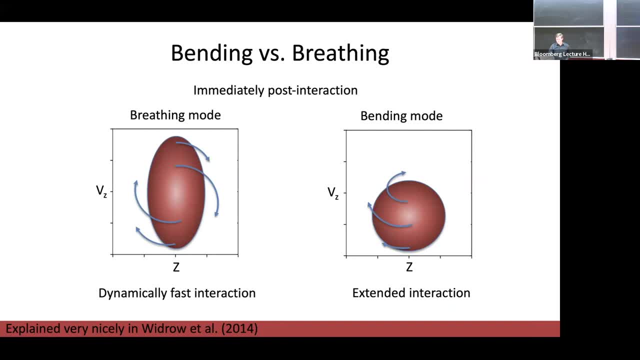 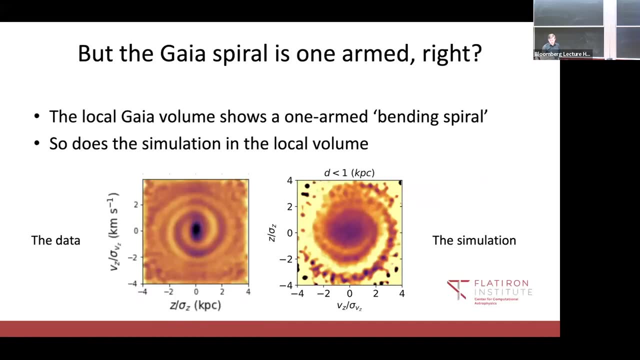 effectively how that happens. There's some nice papers by Udupan and Banach that show this in more mathematical detail. This is just a but. why am I talking about that? Because the gas spiral that I've shown you so far is one armed. 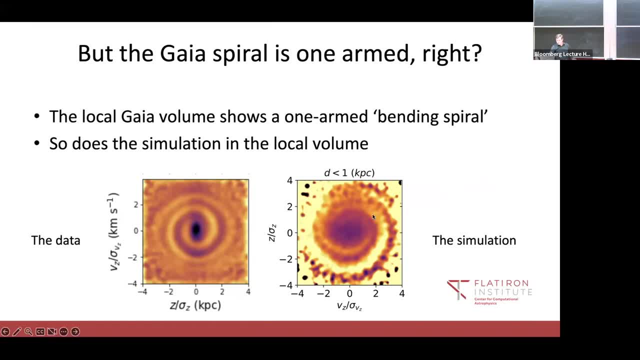 This is the spiral in the local Gaia volume. Well, this is also the spiral in the local simulation volume that we chose to be in the solar neighborhood and generally for the radius of the Sun, regardless of the chosen neighborhood. And so 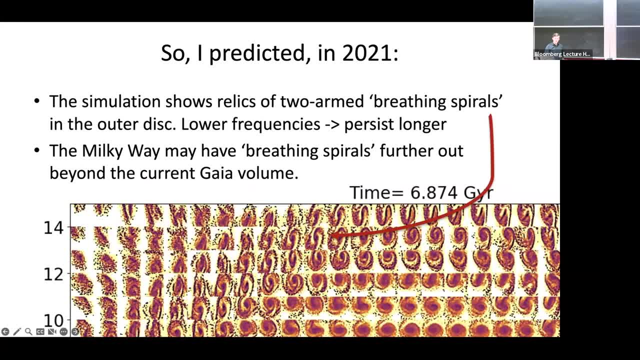 in 2021,. I had a version of this talk that ended predicting, because actually the simulation shows the relics of these two armed breathing spirals in the outer disk. They're messier, but they are still there. you can just about see them. 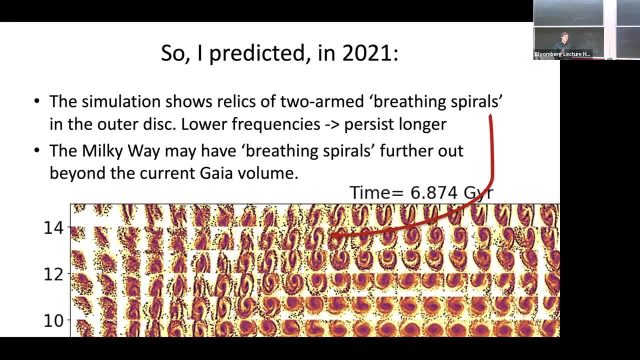 So I predicted that perhaps you would be able to find relics of these old breathing spirals. But in the real Milky Way, once we had data, that goes outside. I'm no longer sure of that because after Scott's paper about the diffusion- and they should probably wipe them out long before they get to this point. but in any case, in this case we can't check. They're still far beyond the observable volume. However, in Gaia DR3, we did actually discover these two armed face spirals. They're in the inner disk, which was the opposite of where I was looking for them. 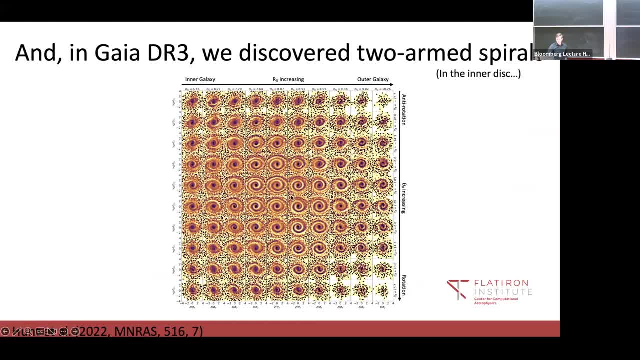 However, this: if you make this map from again splitting in the actions and angles, it's not a true physical map, but it's splitting by angular, mental or guiding radius and the azimuthal phase angle. you see essentially an overlap between two-armed spirals caused by breathing mode and one-armed spirals caused by a bending mode. The blue box is breathing mode in the inner disk and we could actually have predicted this because there are older papers by EG Mary Williams or Ivan Prolog which say detections of a breathing mode in the galaxy. 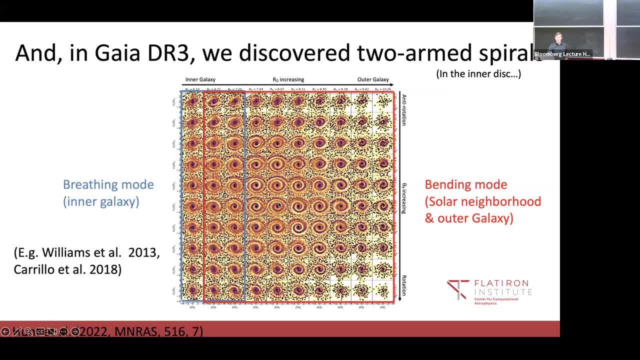 And then the solar neighborhood of the spiral that we'd seen before is one-armed and going out as far as we can see. This is actually still well short of the prediction I showed on the previous page, which will be somewhere off the right of the TV screen. We still aren't anywhere close to it. 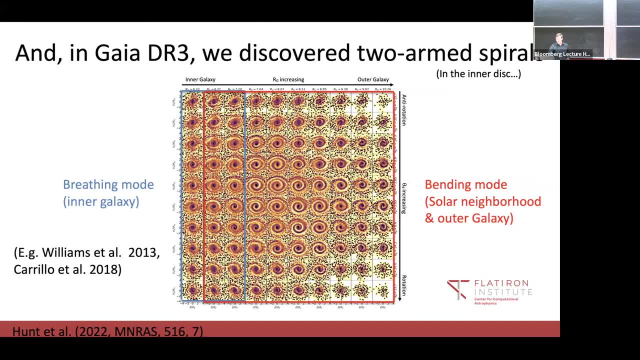 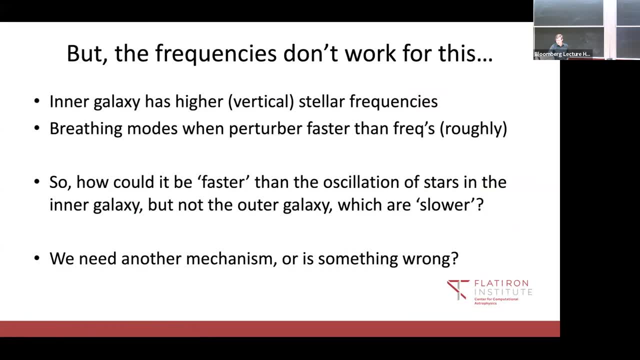 So we could be out there. but I'm not confident. but it is interesting that we see even in the local volume there's apparently two different types of face spirals And the picture I just gave you doesn't work for this. 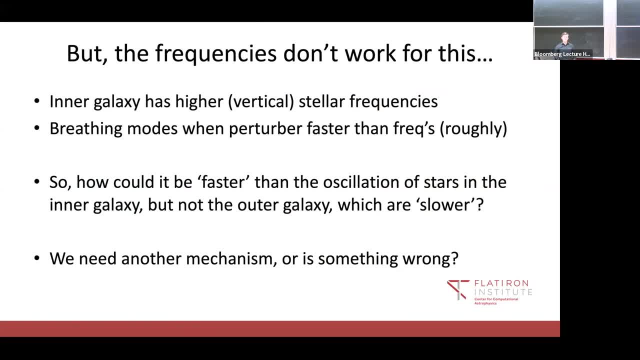 I said that when you have a really full, fast interaction. if the satellite goes by faster than the vertical frequency of stars, then it will induce a breathing mode. If it's slower, it will induce a bending mode. But you can't be faster than the stars in the inner galaxy, which oscillate up and down much quicker. 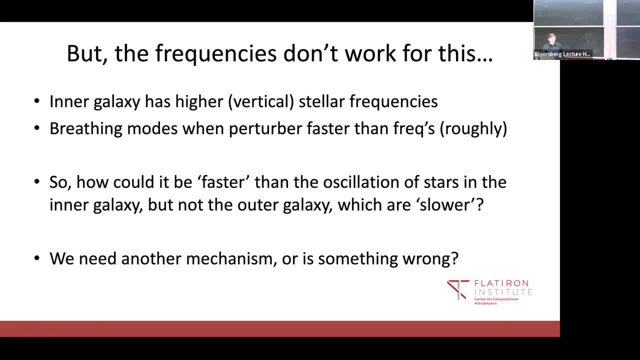 than the stars in the outer galaxy, which is slower. So this little kind of toy hand-wavy model doesn't work. So we need another mechanism, or our understanding of it is just completely wrong in the first place. But luckily there is another option which works quite well. 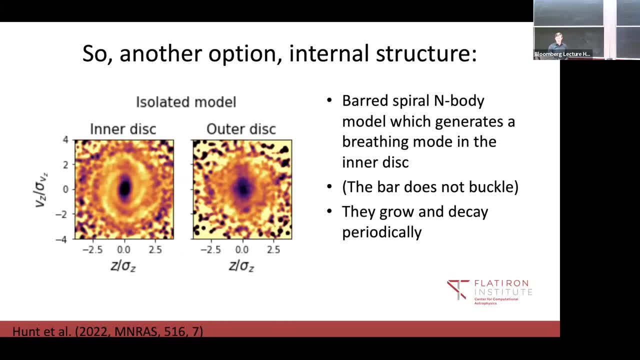 So this is now a much more realistic Milky Way-like disc galaxy, showing you a two-armed face span on the inner disc that arises self-consistently from either the bar or spiral structure. We still need to do more work to determine exactly what is the formal origin, but this galaxy just forms a bar and a spiral arc by itself. 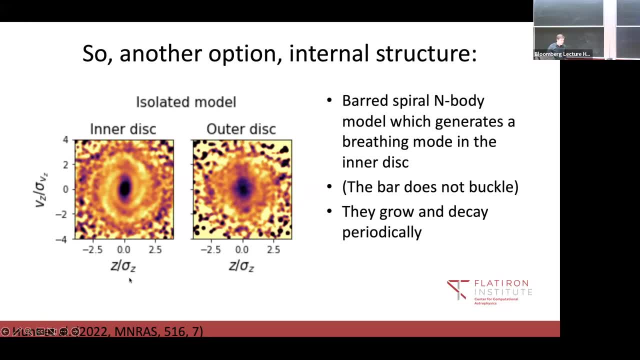 It forms a breathing mode. in the inner disc, Other works- Giacomo Minari or Victor de Bautista- have talked about transient spiral structure creating breathing modes, so that's not entirely a surprise. But in the outer disc there's nothing. We see no face spirals at all. 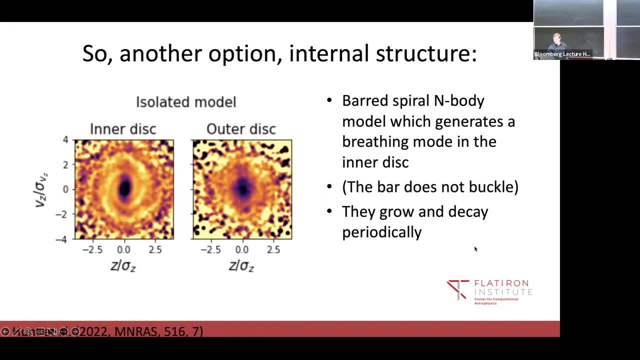 Unfortunately I don't have the movie for this one. It wasn't run to the same resolution. We should go back and re-simulate it now that we know that it's interesting. However, if you take that same galaxy that has two-armed face spirals in the inner volume, nothing in the outskirts. 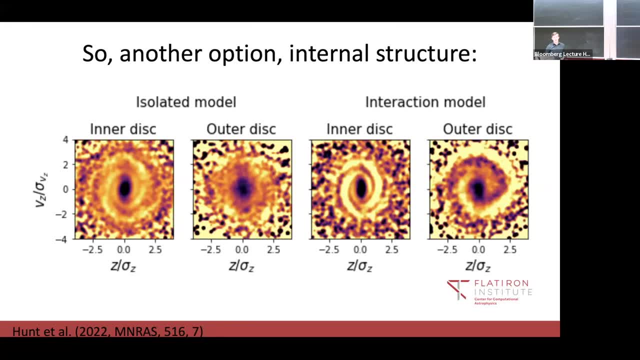 and then you throw a satellite at that one. you actually reproduce what you see in the guide at a point. well, You retain the two-armed breathing mode, spirals in the inner disc caused by diode spiral arms, and now you have one-armed face spirals in the outer disc. 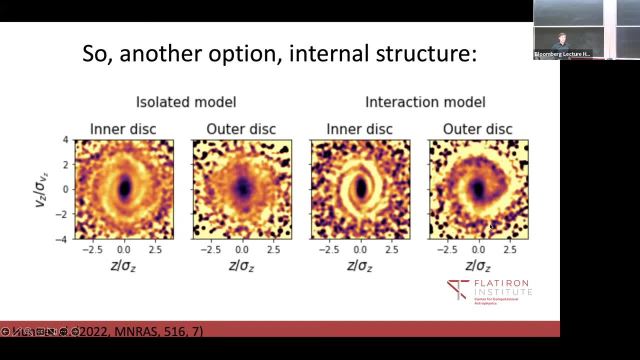 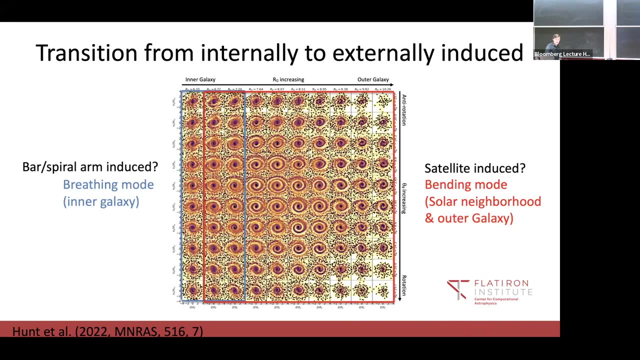 Again, we totally do not match quantitatively the face spirals that we see in the Gaia data. not as tightly wrapped, the amplitude is wrong. but quantitatively you can actually reproduce the split quite nicely by a combination of internally to externally induced vertical disc equilibrium. 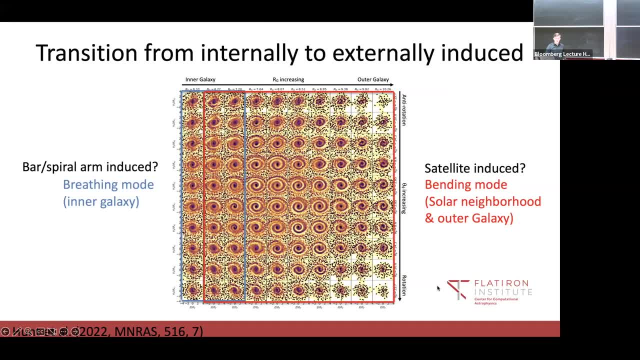 So I suggest that that is what we are seeing here in the real Gaia data: the two-armed face spirals, the breathing mode from the inner galaxy, being generated self-consistently by a Milky Way symmetric structure, and the one-armed face spirals in the outer disc being induced by the passage of some external perturber. 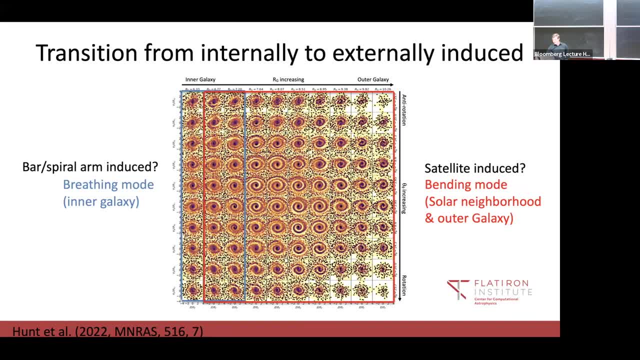 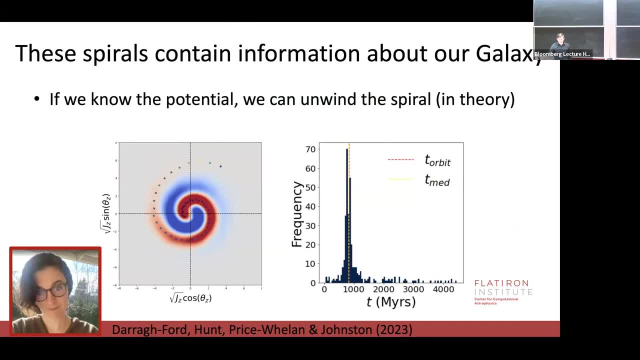 However, that is half uncertain. And as I don't have too much time left, but in brief these, I remind you of the. I think I mentioned, from at least right forward, that if you know the galactic potential- which of course we don't- 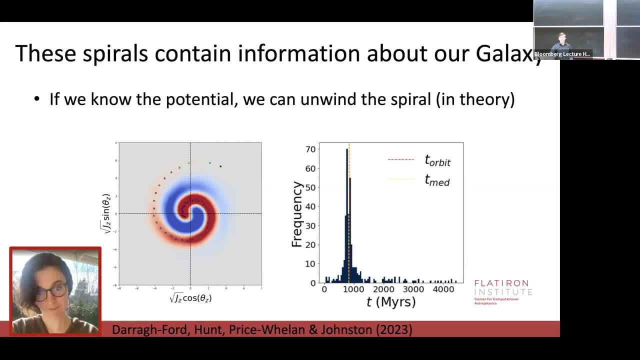 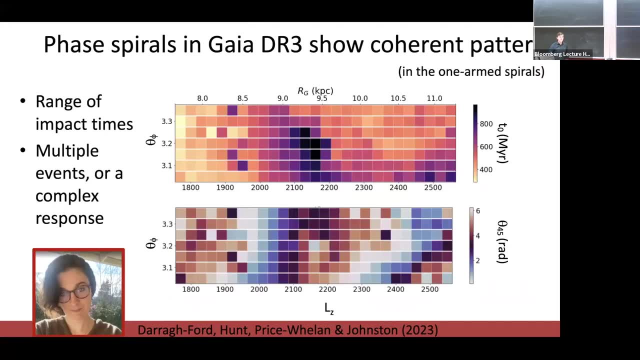 you could unwind the face spiral and learn about the timing of whatever perturbation has caused these things to start wrapping up, And so we can take Elisa's algorithm and we can apply it to the face spirals from Gaia DR3 and make measurements of the time that the interaction would have happened, if this model is correct. 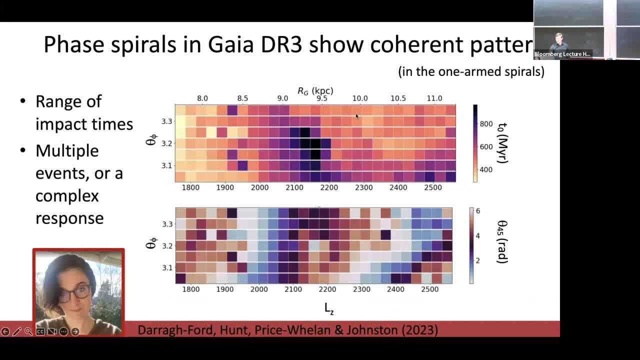 So here we have again, split by angular mentor or azimuthal angular mentor or guiding radius and azimuthal phase angle on the y-axis, And what we're really measuring here is the windedness of the spiral, And we're confident that we're quantifying the windedness quite well. 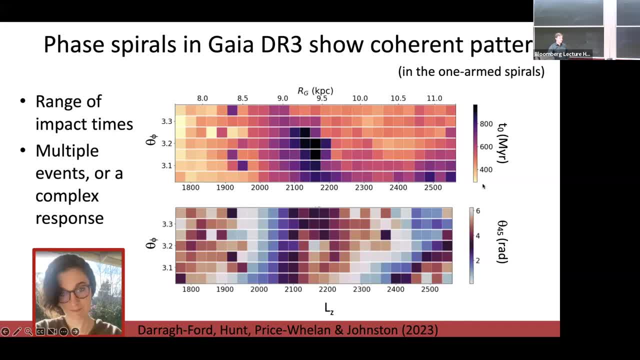 If you use the simple model to go to time, we find a range of perturbation times from about 300 million years to about a giga year. However, this is heavily model-dependent and all the stuff that I mentioned before- self-gravity, other effects, et cetera, et cetera- can make this. 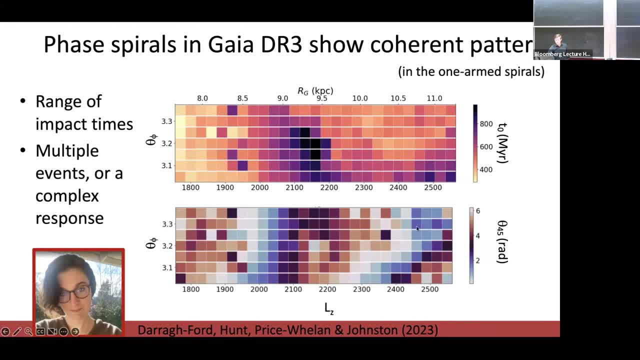 the times not be correct, but the pattern appears to be robust And there's also a similar structure in the phase of these spirals. And the question here becomes: so you have this range of times or the range of windednesses, and is this: 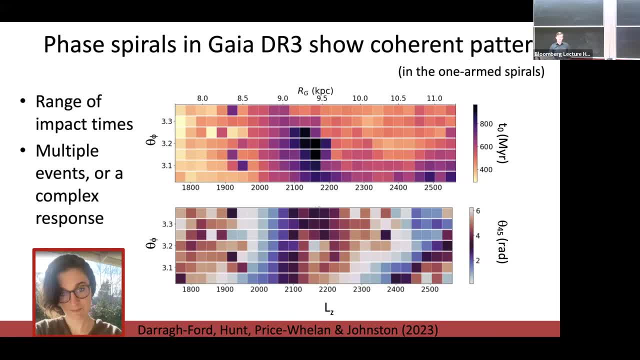 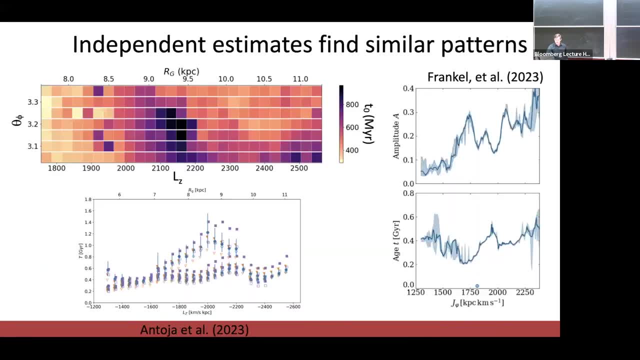 from multiple events, or is this from like complex or full of how these like wind up? And we haven't really solved that yet. However, independent estimates find essentially similar patterns. We have again. this is our same grid here. 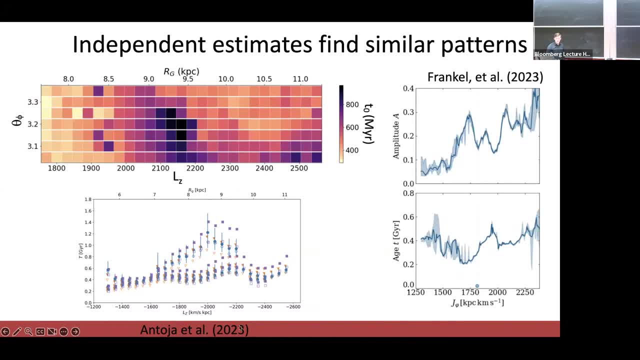 We have angular mentor versus time, found by Teresa and Toya using entirely different spiral, unwinding time measurement-y code, And we have here, on the right from Nege Frankel and Jeroen Scott-Germain, another version of it. You have age. 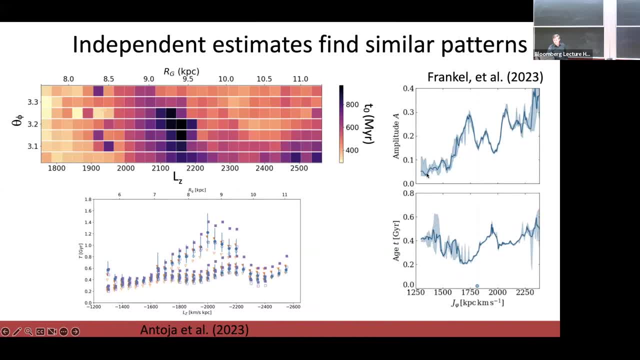 Here versus angular. mentor. A nice thing from Nege's paper. she also quantified the amplitude of these phase spirals And we see basically the same structure. So whatever it is we're measuring, it's nice to get the same, the same structure out from three independent algorithms. 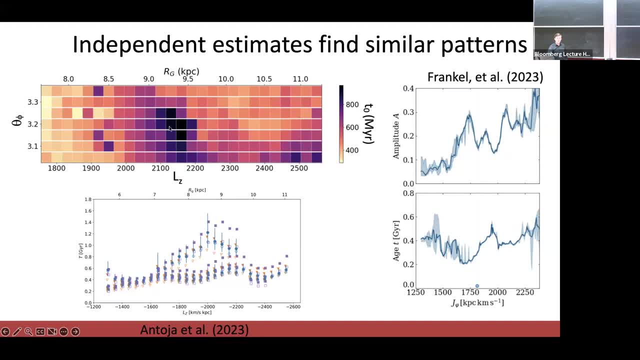 You have this spike of high wear- means high time thing- kind of just outside the solar angular mentor. You have lower times inferred slightly inside and globally a trend upwards. Note that we cut hours off at 1800, so we're missing the left half of the plots on both of these. 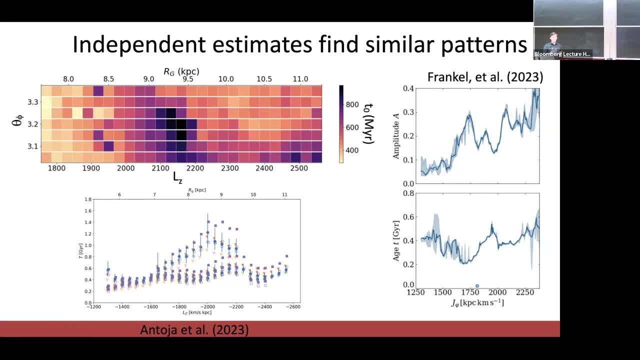 That's because that enters the area where the one and two-armed phase spirals overlap and we've got very high errors in our fits. We just spliced it off. However, if you go through that area where they overlap to the area where you just have clean two-armed phase spirals, we recover a very, very low time. 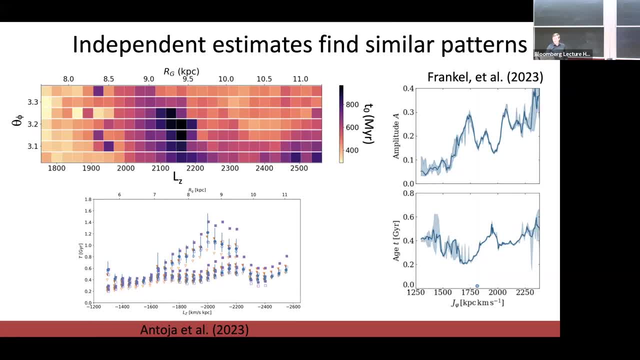 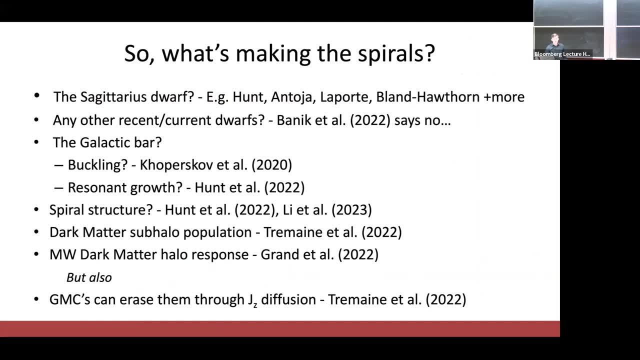 I believe, from talking to Nege, that's the same that she found, but I don't have the plot, And so that's what I've mostly ignored so far- is what's actually making these phase spirals? We have to measure them, we can map them, we can model them, but what actually causes them? 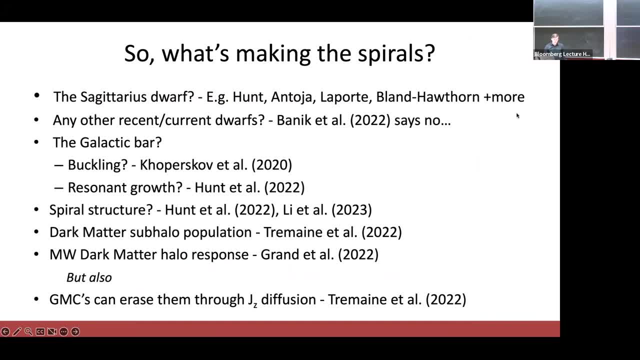 Well, one of the leading contenders at the first time, when we first discovered it, was the Sagittarius dwarf galaxy. We know we have this dwarf that's merging into the Milky Way. It's been doing it for years. Myself, Therese Artaud, I've run simulations of this. 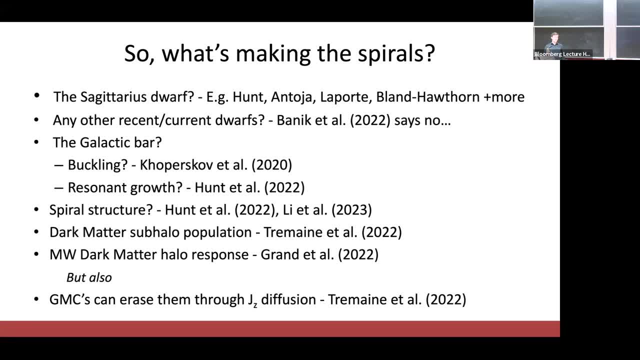 The difficulty is the present-day mass of the Sagittarius bremen. It's pretty huge. It's like four times ten to the eighth solar masses, And that's not enough to do what we see with this, However, of course, it will have been losing mass for its previous pericenters. 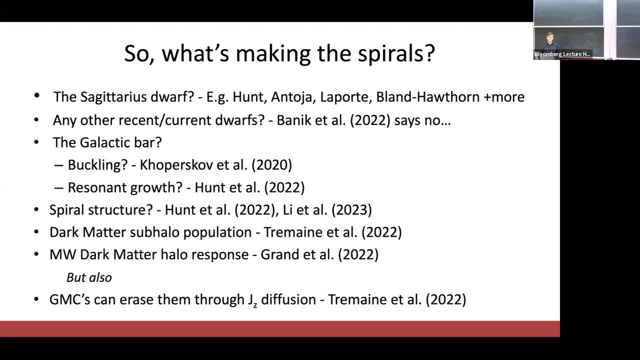 So it's possible. there's a way to reconcile recent mass loss with degree of distortion, But no one's managed it yet. Other options: Are there any other recent current dwarfs? Because we have the Magellanic clouds for this one. On the first info, it's not time for the phase spirals to break up. 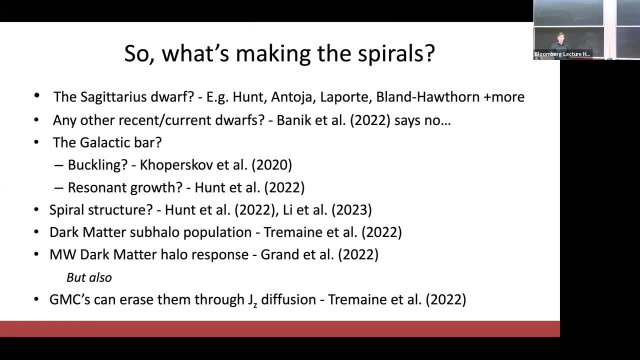 Magellanic clouds should eventually make beautiful phase spirals. Of course the Milky Way will all be long gone And other dwarfs are too recent, But I'm betting it doesn't expect the looks of the effects and rules out other things. 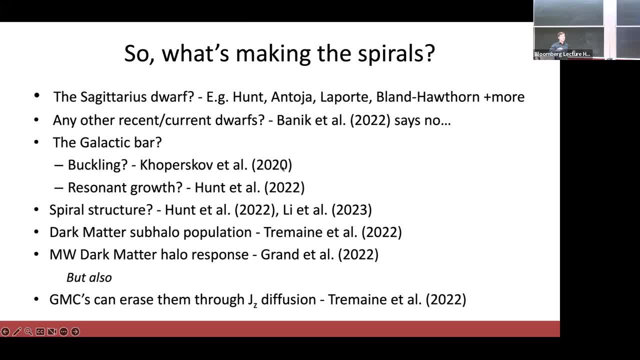 Other options: Collective bar. So I gave you a couple of stuff to show. If the bar buckles, it creates a variable disturbance that creates one-armed phase spirals. And then myself, my bar, in the model I showed you, does not buckle. 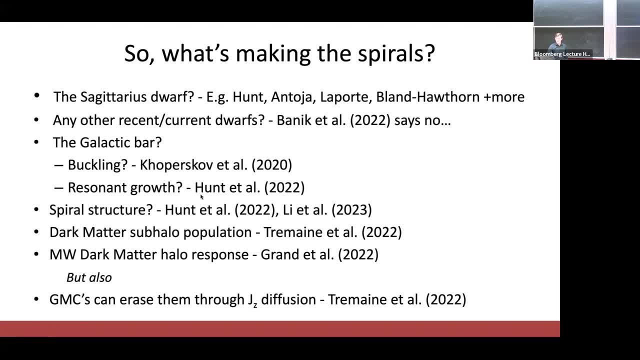 It grows slowly and resonantly and also makes spiral arms. So between them the combination of the resonant growth or spiral structure, you can reproduce these. Scott Germain had the recent papers showing a series of smaller perturbers such as dark matter. subhalos can also generate these phase spirals through, instead of one large perturbation, a series of lots of smaller ones. 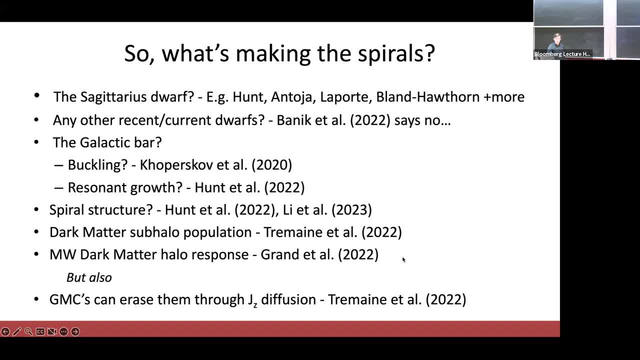 And Robert Graham showed that actually the Milky Way dark matter halo response can be enough to perturb the disc vertically to the degree that you see. So if you have an older satellite come in, make the halo significantly triaxial and out of equilibrium, then the halo effect on the disc is actually dominant. 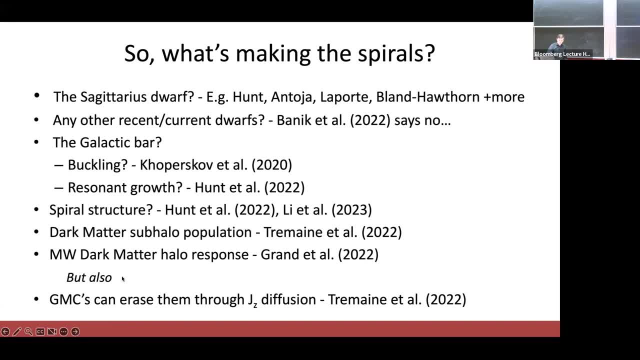 And that's what causes it all. So wind up, And then also in the other direction. Scott's paper on GMCs can actually cause them to disappear sooner through action, diffusion, through interaction with the giant magnetic clouds. So, given all that, what's the answer? 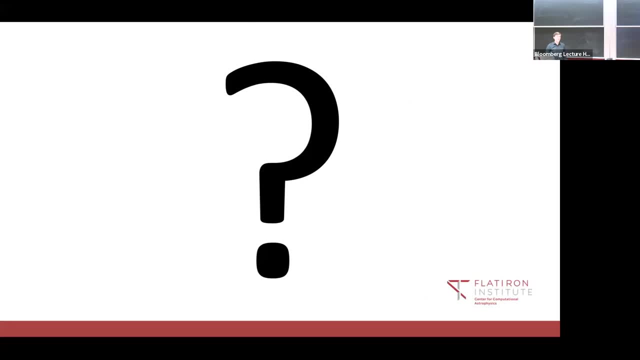 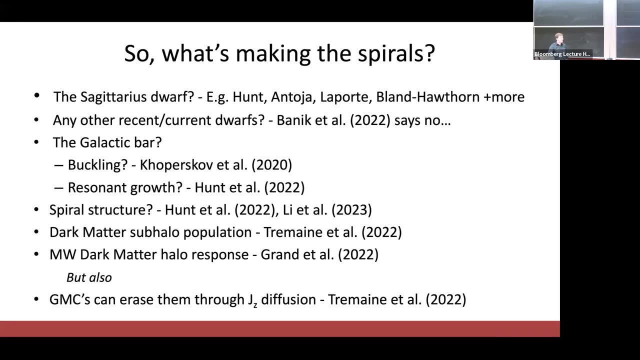 What's actually making these phase spirals? And, yeah, we don't know. I leave you instead with a mystery for today, but you have many groups working on it, So I think we should be able to come to some kind of consensus over the next few years. 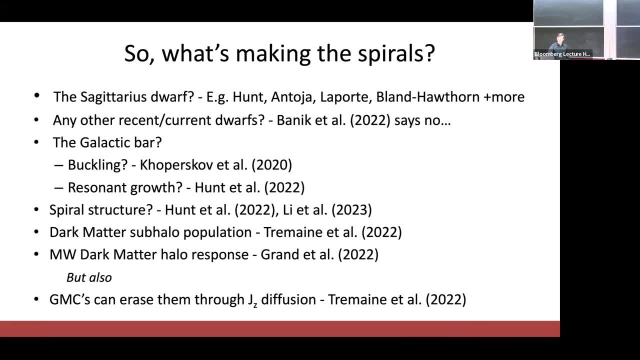 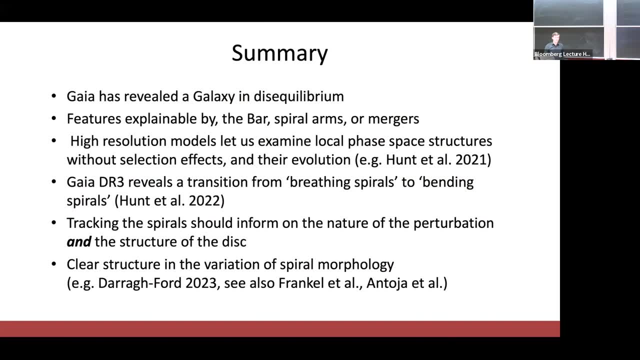 But at the moment it's still fairly fresh And yeah, and that is the end for me, Thanks to all those collaborators who are featured, I will leave up the summaries and take more questions. Thank you, Jason. I think we have about 10 minutes for questions. 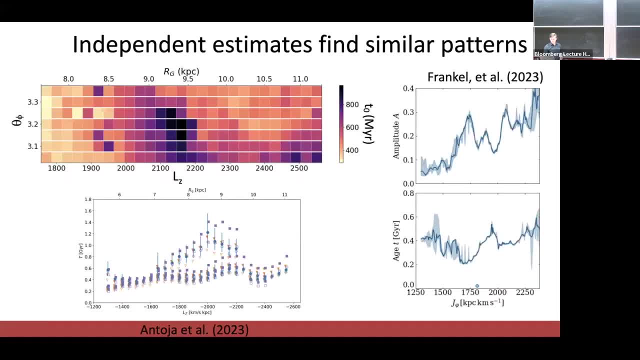 Yeah, So we go back to the time estimation of the impact. So the next one is wonder: how should we interpret these different age? Does it mean that if you pick a particular part of the way, then you expect like the impact at some time and then choose another region, then that means it's another time? 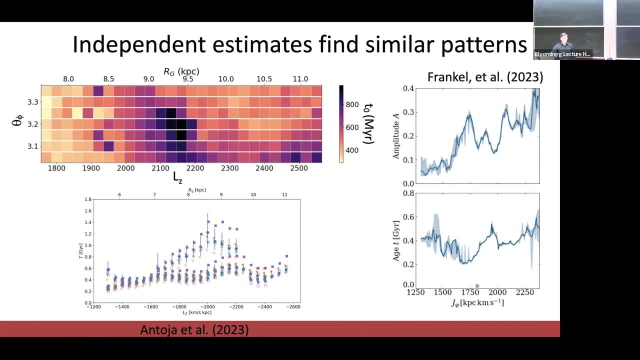 So that shows that these like single impact is in this scenario. It's not, incidentally, stated, So this is the question that we are discussing at the moment. I think actually, like I was saying, I'm interested to talk to more of Scott about while I'm here. 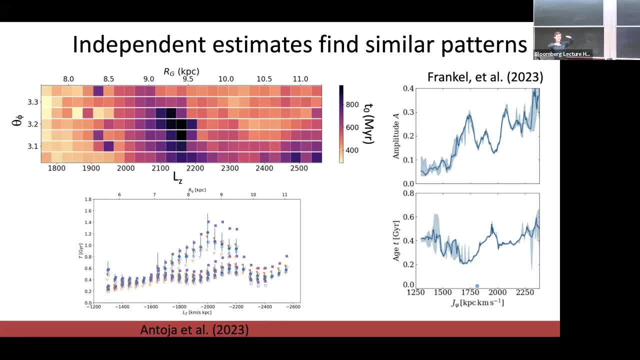 But we have. if you have a long, slow interaction with the satellite, like loops under the desk, the time when the stars are different parts of the galaxy experience the perturbation, but maximum perturbation and start to wine is different, So you can create these kind of stripes with a different timing from just a single interaction. 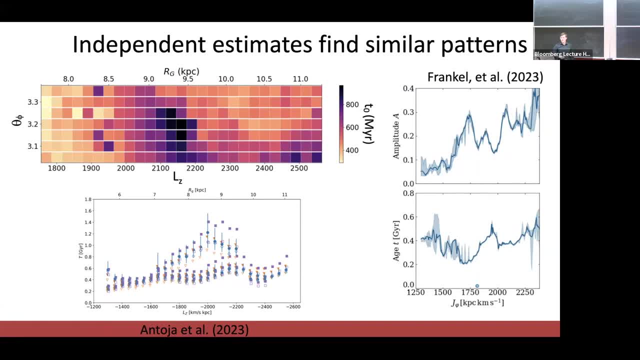 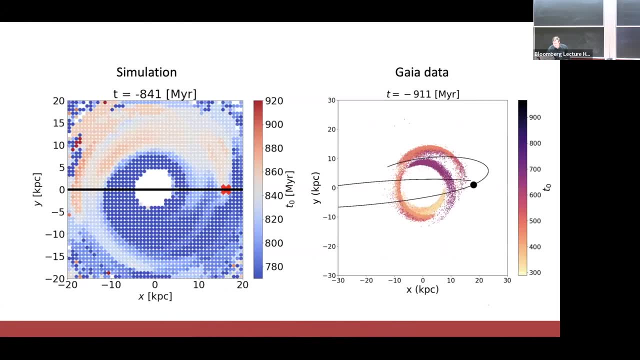 But the like: if you have one very incredibly rapid passage, that's not so much the case. I have somewhere in the slide It's this picture. So this is from the test particle model from Elise that shows If you have this satellite that goes by, then you measure all the face panels of the present day. 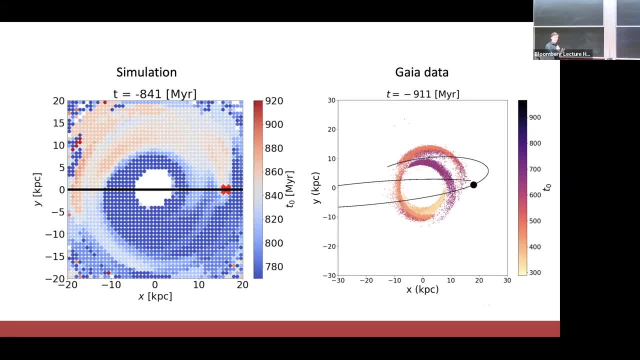 And then you wind all those volumes back to where they were when the satellite crossed, which is not quite fair Because the crossing thing is slightly different. Then you get close to a dipole in the times during third. Listen, this isn't that big a difference. 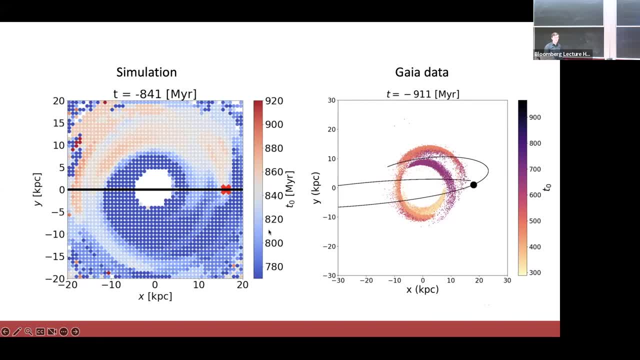 Okay, This is 880.. That's 820. So still within a hundred years, just smaller from the range We see in the guy data. But the length of time spent doing the crossing and the mass of the satellite changes how different you can get. 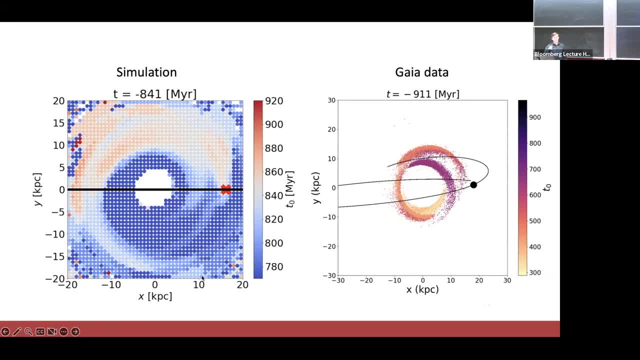 And then, when these features will start to wind up- because the inner Galaxy rotates faster than the outer Galaxy- they can start to cross and leave bands of different face spirals. So you can do it with a single elevation to make different times. I'm not saying that's the right answer, but it doesn't rule it out. 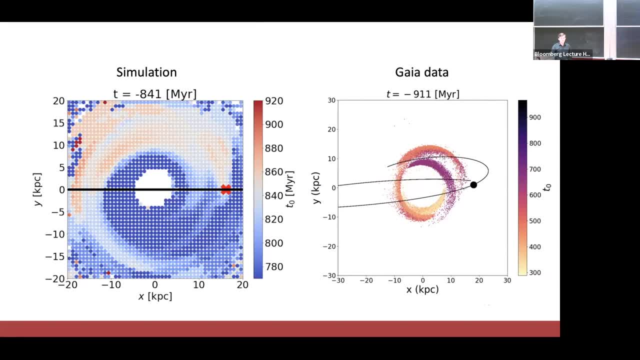 Okay. So then I also wonder: um, so it seems that, like, like with one spiral, basically probably only have two things to can strike right. One is likely: you have the single arm and double our strengths Basically probably also have the face of it. 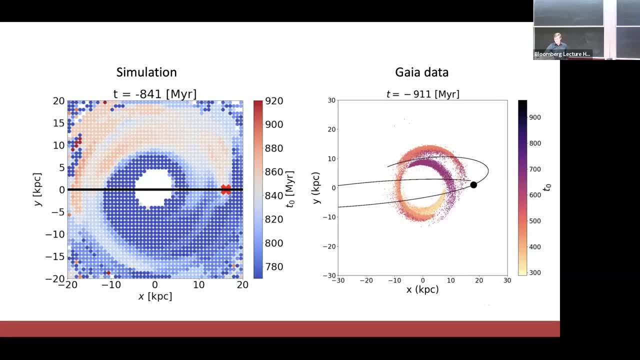 So so. so from one spiral you can can strike basically for numbers, And now we have many different actions. So what we'll do, Say about the degree of freedom of models You can construct that, given the current guy, because like, yeah, you still have noise, right? 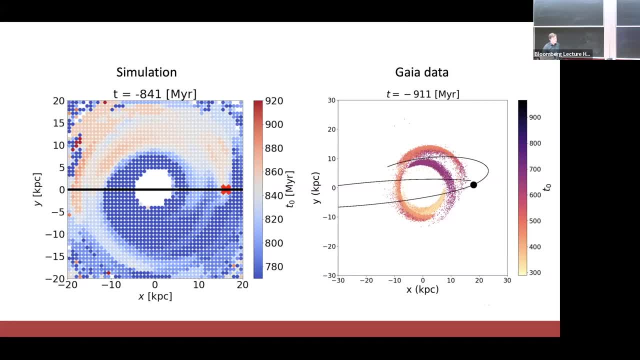 So exactly, You don't have infinite number of degree of freedom. It's a good question. I don't. I don't know the actual answer to that, But if anything we've given us, we've given ourselves too much room to fit things with. 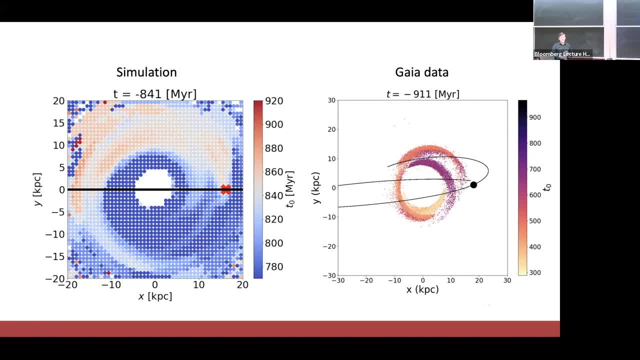 And if it's like for one passage or two passage, I suppose Don't have many degree of freedom, but given the data, I have a lot of things to constrain. So basically I have to say very strongly, like whether the data is consistent with some order or not. 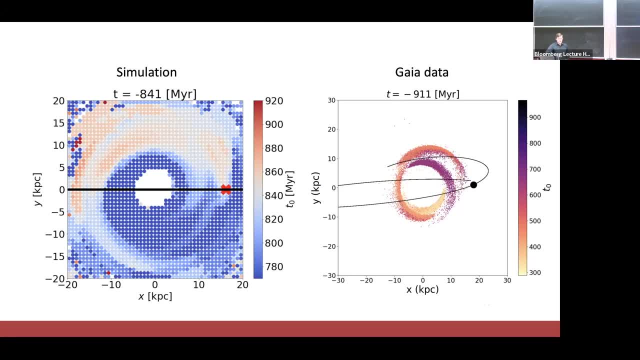 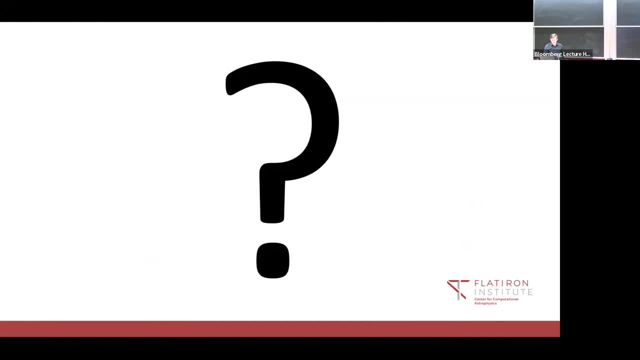 It's. yeah, you can certainly check consistency against, like the simple models. I think the problem Problem is that this one, basically all of this, is going on right. We have a Sagittarius, We have other dwarfs that are affected. 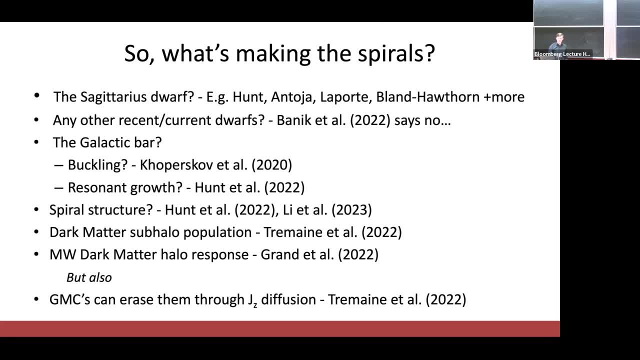 The minimum. We have a galactic Far. We have spiral structure, Probably, depending on who you talk to, probably have dark matter subhalos, depending on your preferred theory of dark matter. We again, that's dark matter. 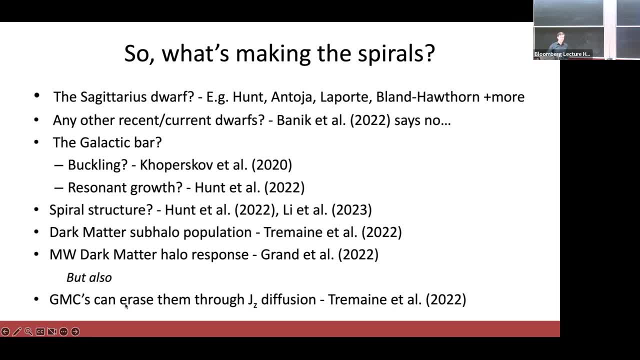 Halo probably responds somehow. And yes, we also have GMC, So we. the question is: is one of these things dominant, in which case we can probably unwind and get the answer, But it could also be a really complex combination of all of this stuff, because the galaxy does have all of these things. 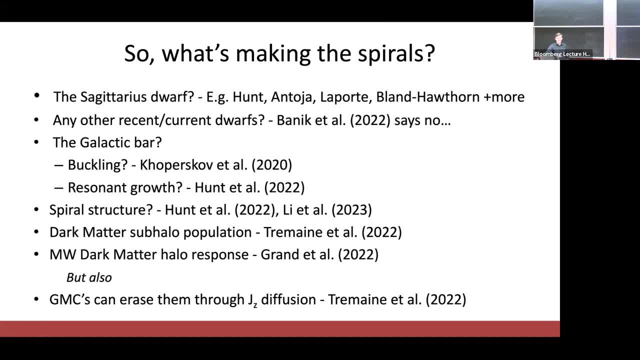 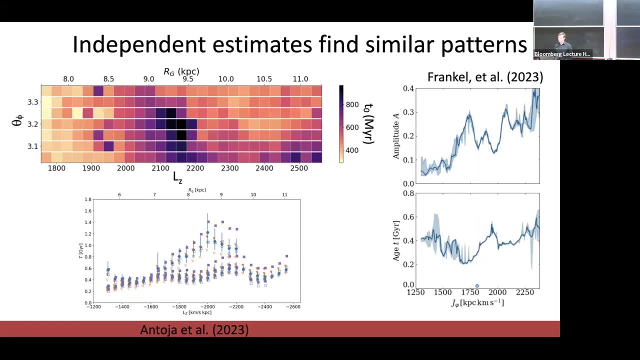 And then how are you decided? I don't know. Yeah, Actually that's a follow up question. If you can go back to the side of the time panel We'll be showing here Each pixel. here is a single highest likelihood time for unwinding. 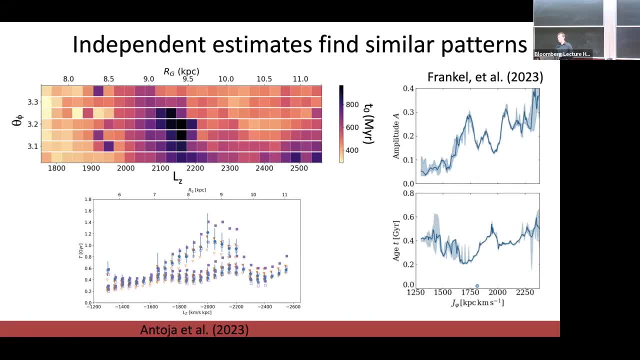 That's in theory. You've got multiple patterns and you could certainly have a two-armed and a one-armed spiral superimposed. Have you decomposed? Is there any way you can decompose it to say there's one big global thing, that kind of spread through with a certain time in their local things that have a different time scale? 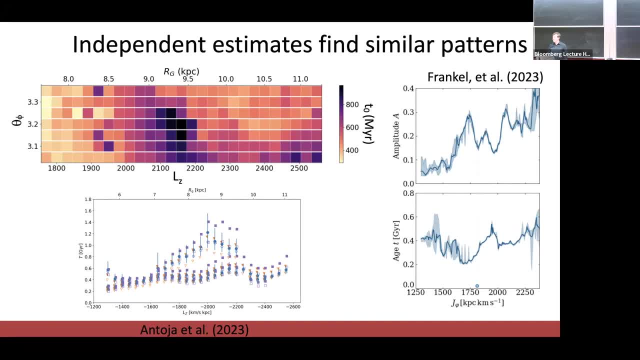 So that's actually what we're trying to do at the moment. I haven't put it in here because it's still too early days. It's Kian's project, if you know that, But for other people. we are trying to take those individual phase spirals and decompose them into the different modes using various basis function expansions of that space, and then correlate that. 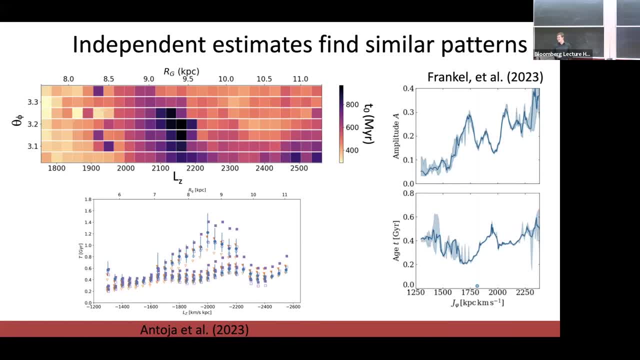 Both pull apart the different modes in the same spirals but also correlate it to global spiral patterns. Currently his results look really cool and kind of complicated. So yeah, It seems to be working, but we don't have any answers out of it yet. 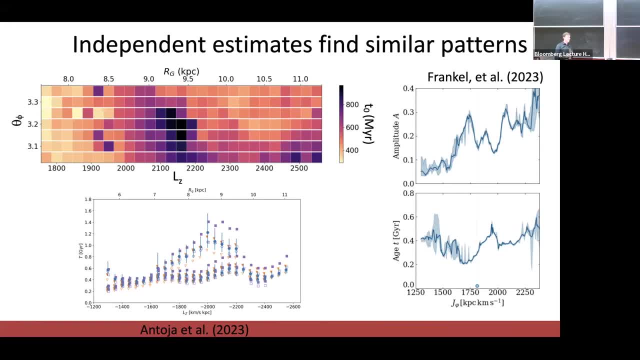 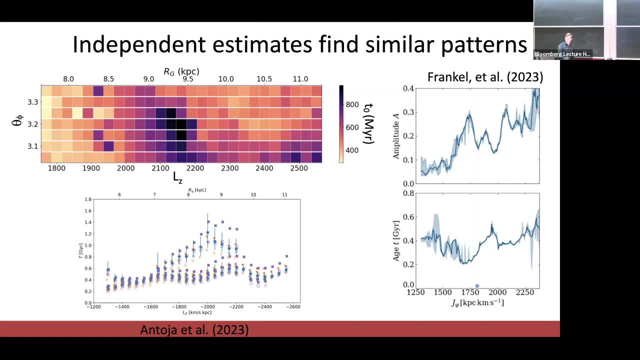 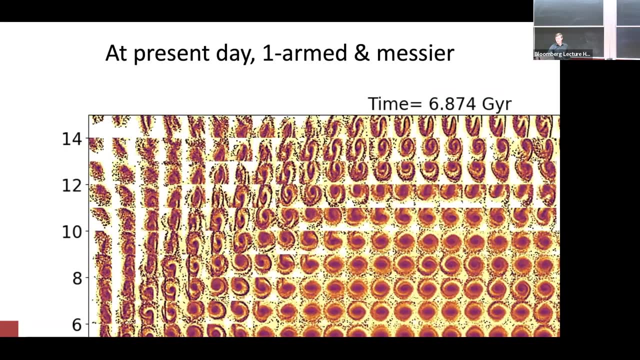 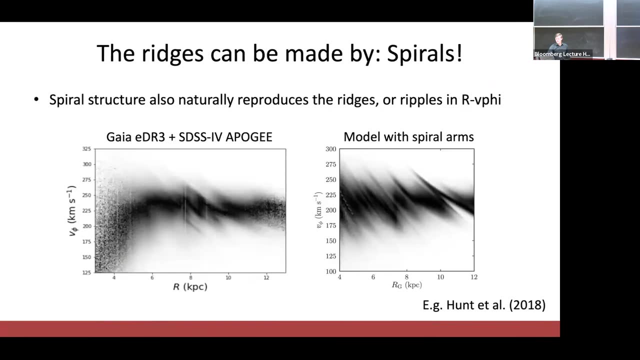 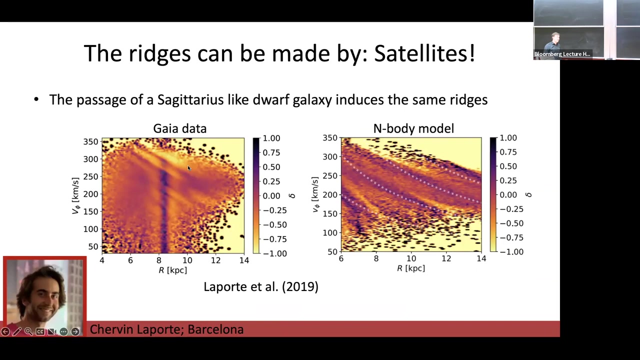 So the understanding that I think we have- and I've seen written on a bunch of papers- is that resonances should make those features linear. The other question is, when you have this kind of distance and the linear data- at the moment it's not entirely clear whether this 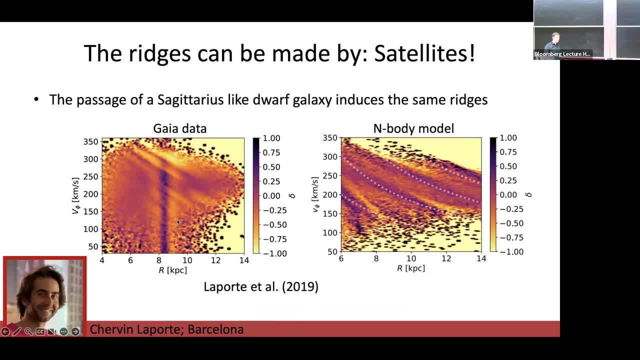 straight line here is truly a straight line, which would imply energy and phase mixing, or whether it is just the locally flat part of a curve, because we don't have enough fidelity to see whether it will later follow a line of constant angular. mentor, as you go out further into the disk. 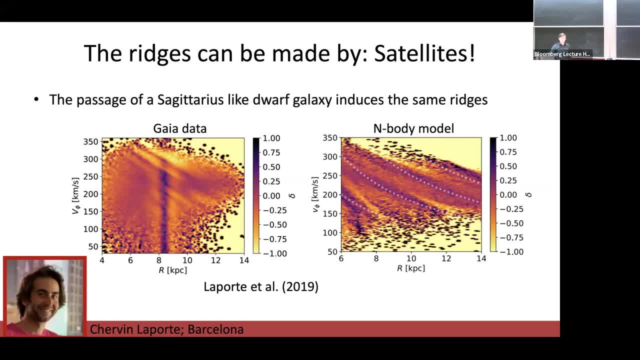 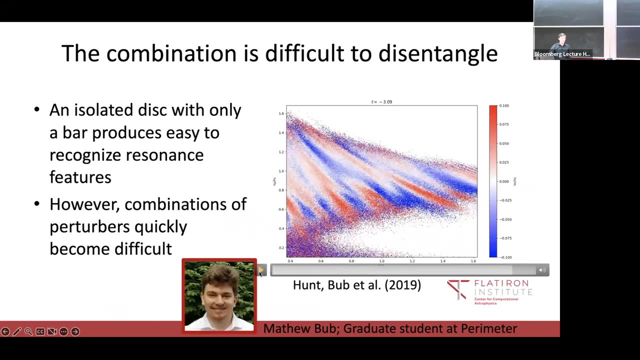 People do try to measure that, and so people have made a distinction between which could be resonant and phase mixing, depending on whether they follow constant energy or angular mentor. but I always like to caution for this, because when you have bars and spirals interacting, it's actually quite hard to measure like in any one frozen moment in time some lines can look. 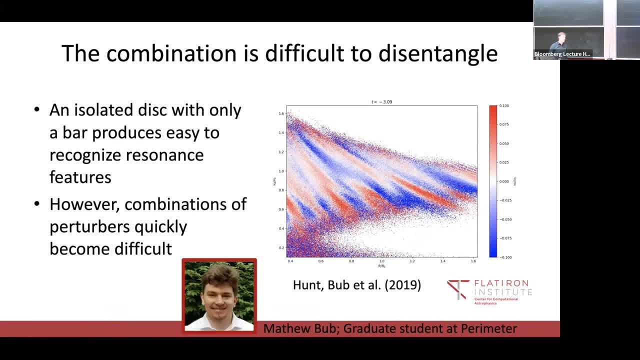 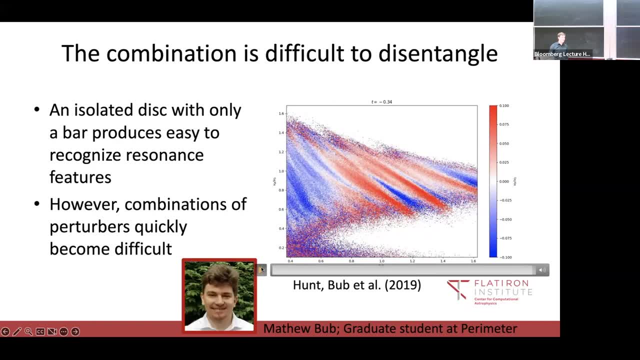 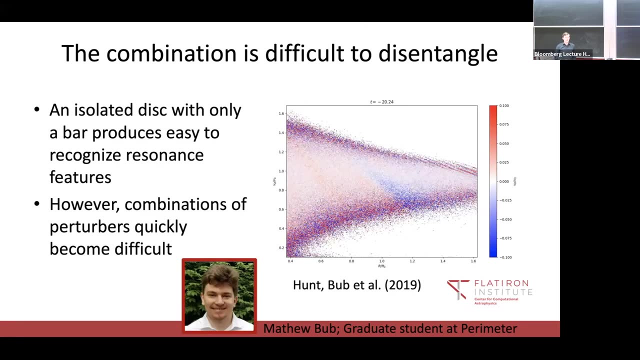 like they follow lines of constant angular mentor or constant energy, whereas in fact, given another 10 million years, the shape of this feature has changed from the interaction of the bar and spiral. fortunately, The slope of the lines cannot tell you whether it's constant energy. yeah, it should do that. that's what it should tell you. the problem is. 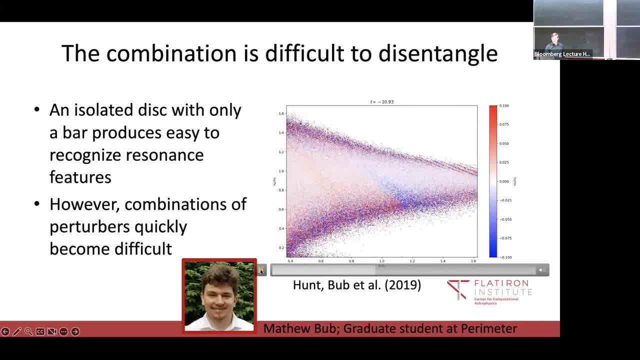 when you, when you have a clean galaxy with not much else going on, like this instance, you can measure these features. this isn't density, actually, so this is slightly misleading, because the density ridge follows a slightly curved line of constant angular mentor just on the top edge of this blue bit here, and that you can measure as you can. firstly, you 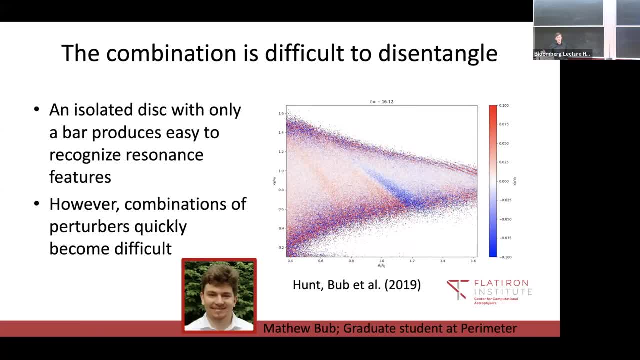 can tell it's a resonance. you can tell the order of the resonance by how it moves as a leaflet. you can tell the speed of the bar by where it occurs in the space. you can tell the amplitude of the bar from how strong a feature it creates. however, as soon as you have a more complicated space, 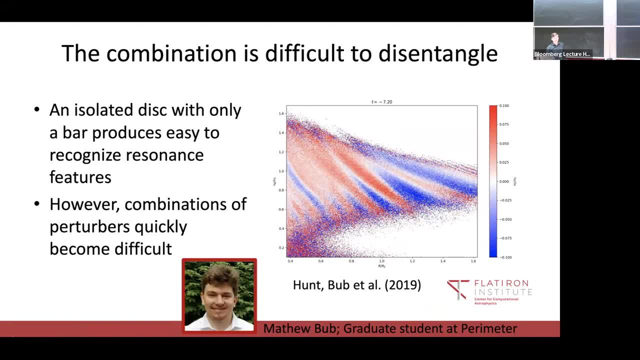 you don't know what you're measuring, you can still measure it. you just might might be killing the rough things you can't understand. what would be this, the simplest physical model that will give you the basic structure of the spiral, if I were to grab a central rotating fluid? 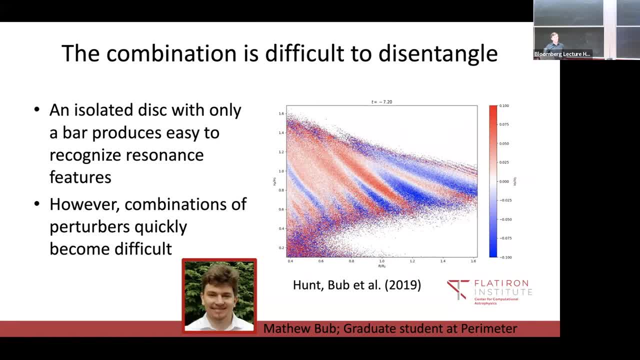 allow me for a second, and I do a local analysis, and I do, you know I impose on forcing the vertical direction. will I get the basic structure of the spiral right or not? and if not, what is that? that is getting wrong again, again. honestly, I don't know exactly how your model would respond to it. 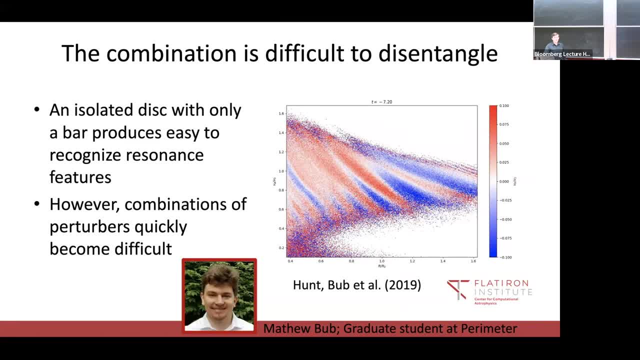 in this instance, anything if you had, if your self-graveling fluid would behave roughly as like the simple harmonic oscillator that mixes back towards equilibrium, then yeah, you'll get a phase spiral. if you're doing constant forcing, I suspect you'd get something that's more standing. 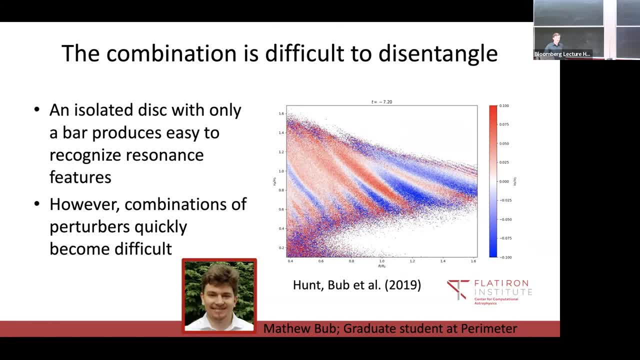 but I don't know, it's not quite right because if I remember correctly, you look at, you know the star weight, to get a bending weight and breathing motion in a disk, right, oh yeah, we can do that, and just you know often the question because it would be useful to have a very simple model that. 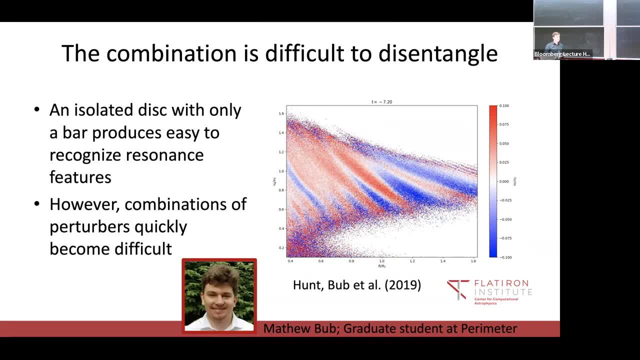 would get actually a very simple model. that would get a very simple model. that would get a very simple model actually, despite that. I mean you have some, you know, sketches and cartoons, but yeah, so the there are. there's the student we're working with from the dynamic summer school. the CCA has done a lot. 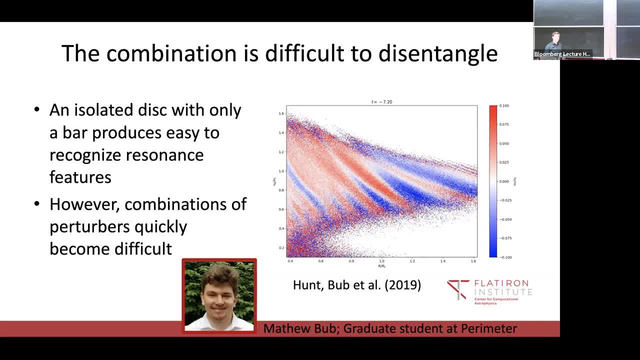 more of the simple analytical models how the spirals form and evolve. so I would direct you to his papers if you want to see that. but it's a good point. actually, I would do well to take some of his animations to show how they form, because he's done that quite nicely. 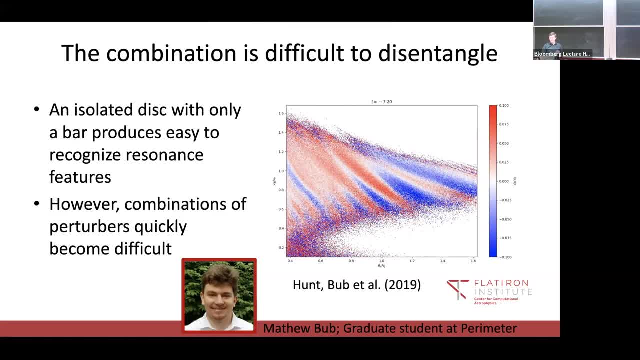 all right, so I think Jason wants more.